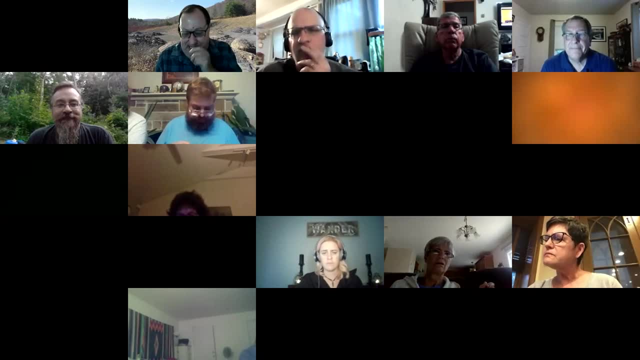 But he's a great webmaster and very efficient, And just keep Dick Naylor in your prayers, if you would please. The news that he's going to soon receive is going to be all good stuff. So, anyway, anybody, have anything else you want to bring up. 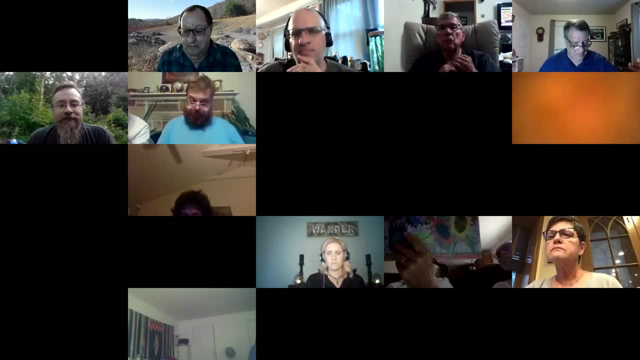 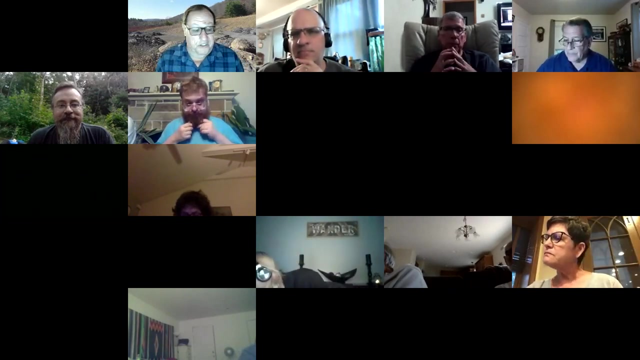 I don't have anything at this point, So we're going to pass it on. I'm going to move on And Give a little introduction to our speaker tonight. I believe that he can share the screen when he's ready to, And anyway, most of us know Steve Lindbergh. 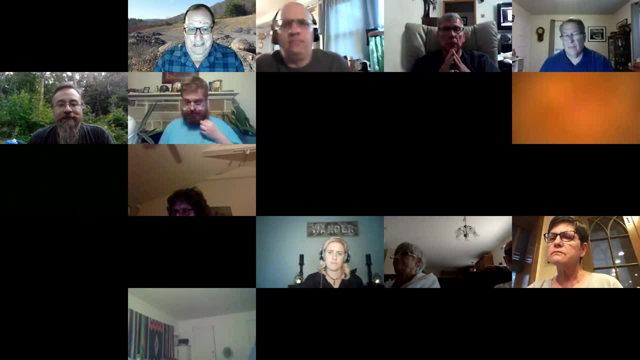 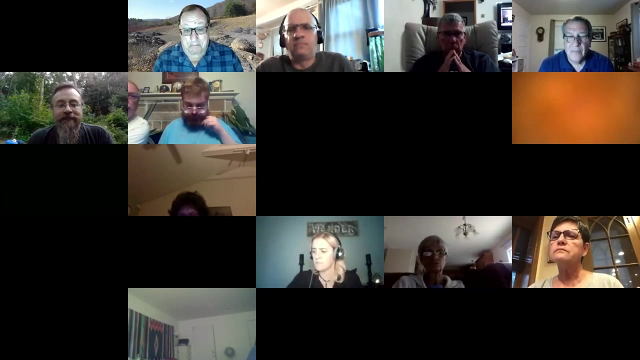 Been part of our Zoom Rock Room for a long time now And has been a great consultant when we needed some questions answered, And we're really, really happy And we're really happy that he's part of our, of our group. But Steve is a professor at the University of Pittsburgh in Johnstown. 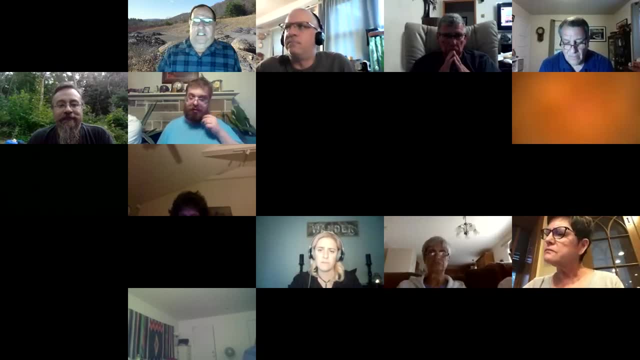 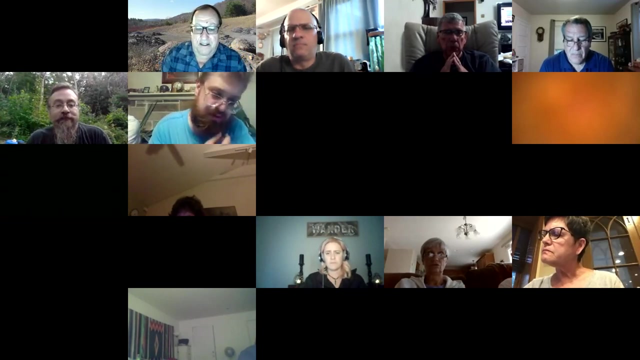 Part of the division of Energy and Earth Resources. He got his bachelor's of science at Waynesburg College in Pennsylvania And got his master's degree at Stony Brook in New York. He loves astronomy, meteorology, prehistoric life, earthquakes and volcanoes. 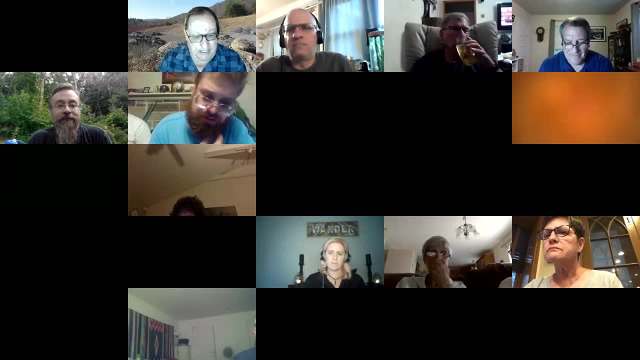 And I believe that at the college he also enjoys teaching geologic field methods. And I don't think anybody in the group tonight is going to be going on the Pennsylvania Conference of Pennsylvania Geologists in October But I know Steve has a huge part of that tour into western Pennsylvania. 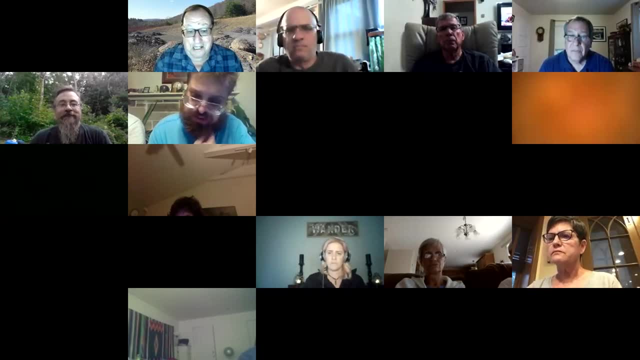 And I think he's going to be going on the Pennsylvania Conference of Pennsylvania Geologists in October. So, anyway, we're going to welcome Steve. He's going to talk about abundant invertebrate fossils tonight. So, Steve, go ahead, It's all yours. 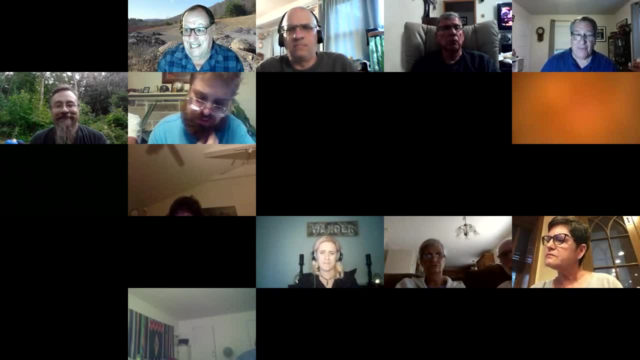 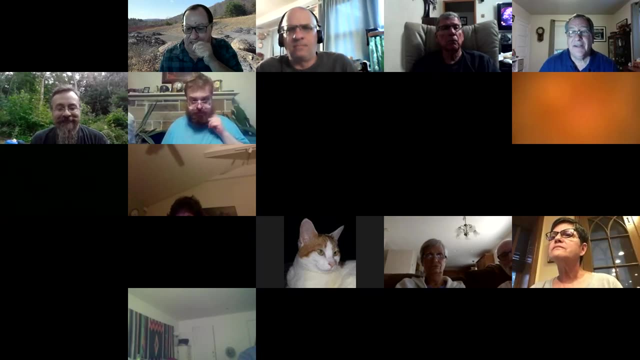 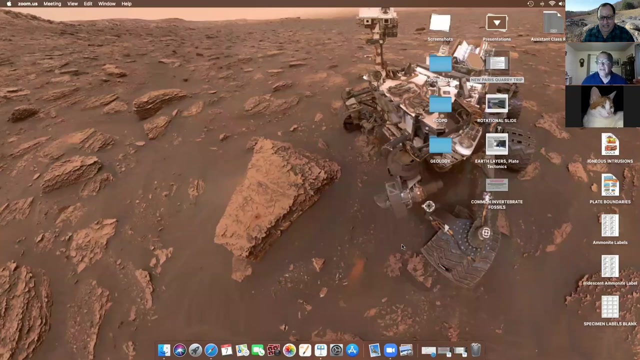 Boy. thanks, Jerry, I appreciate that overwhelming. Let me see Share screen. You don't have it, I don't have it. You don't have it. Let me see Yep, you got it. Oh, I got it. 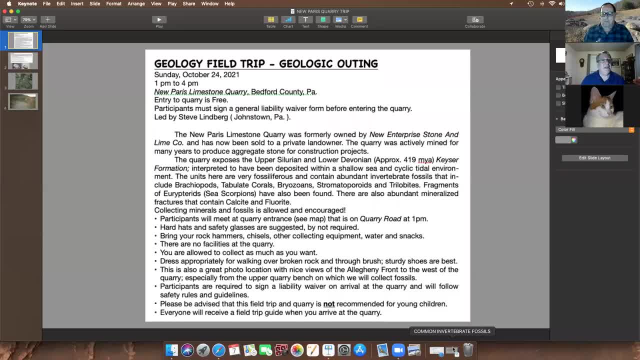 Okay, you're seeing my screen, not the. There we go. Okay, is that? Yeah, thank you for that nice introduction. It's nice to be with everyone again tonight. I very much appreciate the invite back. I'm going to keep. 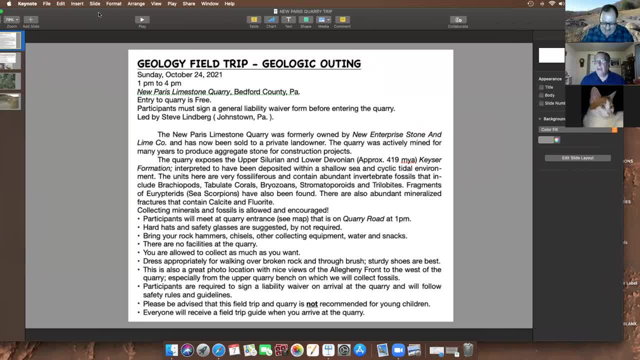 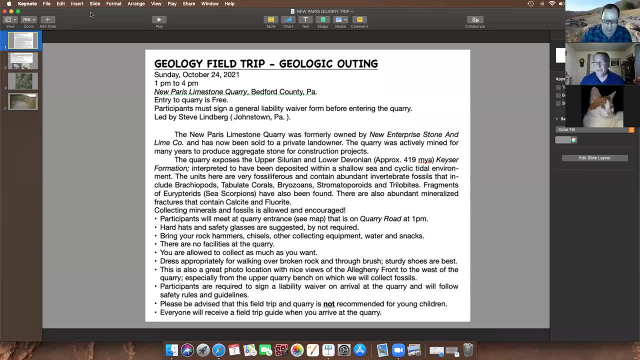 Is this visible to everyone? Can you see that? That's good for me. Okay, rather than go full screen with the PowerPoint, I think I did this before. I'm going to keep it like this as long as everyone can see it. 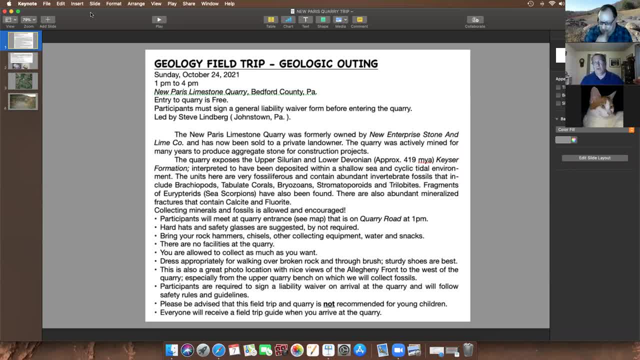 I had problems on last Friday morning when I taught my OLLI class. I went full screen with my PowerPoint and it kept locking up and freezing on me So and I had to restart and leave the class and come back in. So I'll just leave it like this. 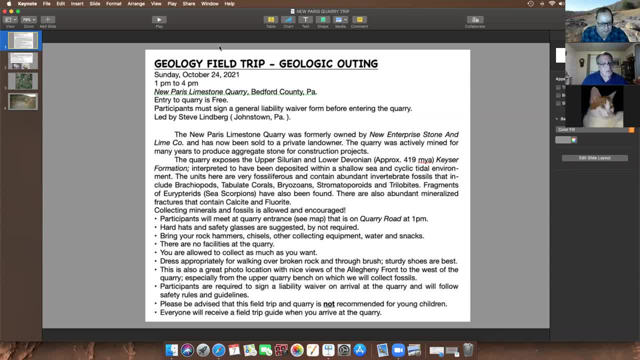 But just as a brief introduction- I know Jerry should have emailed us out to everyone- Here are the details of the upcoming October 24th field trip to the new Paris limestone quarry. This is the same exact thing that I sent Jerry. This was an active quarry owned by New Enterprise Stone and Lime. 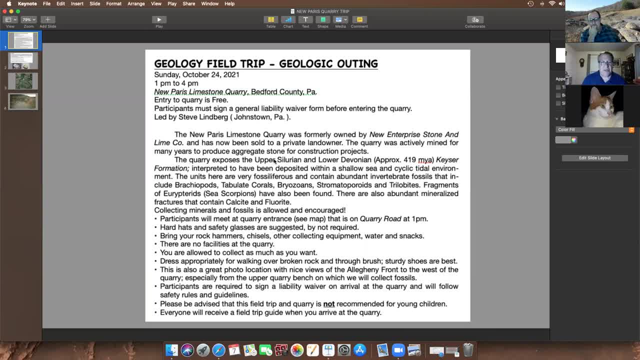 They were mining the limestone out of here for aggregate and building stone. It was shut down. I'm going to say in the mid-80s, the late 80s, it was shut down. It sat for a long time being inactive. 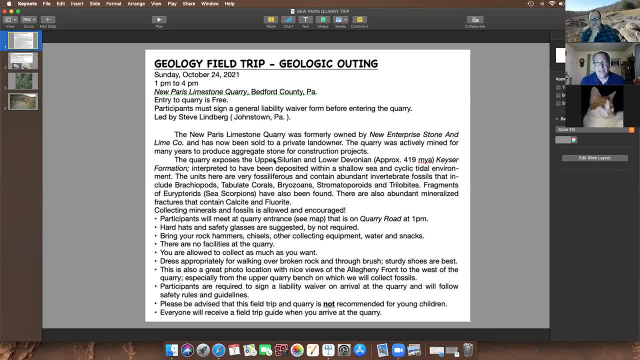 And I believe two years ago or two and a half years ago, they decided to sell the property And it was shut down, So it's been inactive for a long time. It's been inactive for a long time, So they decided to sell the property. 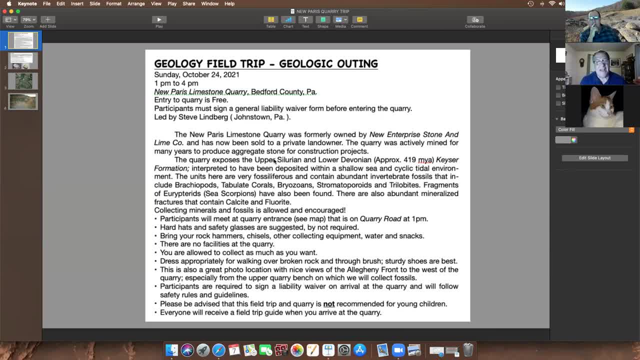 And the neighboring farmer. the neighboring property owner, Andy Lang, purchased it And we had a long history of bringing students there from Pitt and on field trips and to do field work, So he was more than thrilled to leave the quarry open for us to visit any time. 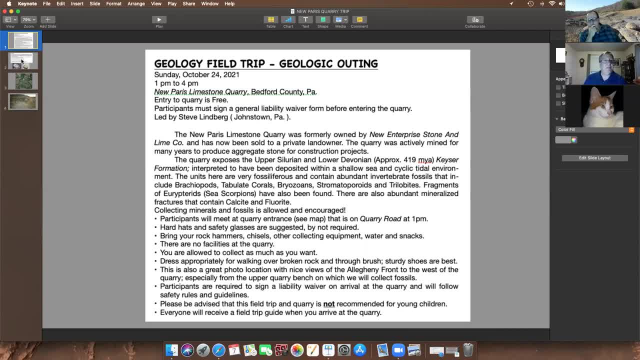 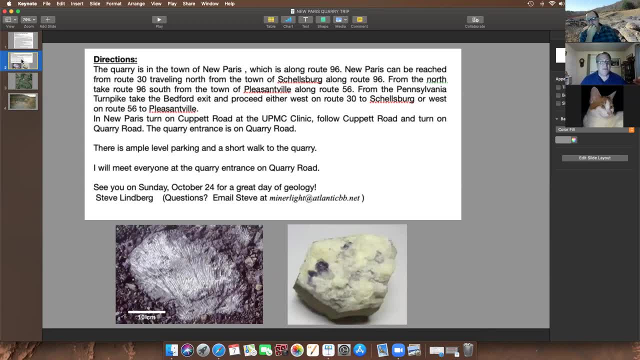 So there's no fee involved. It's- I have a couple of pictures here- ample parking. We have lots of time yet to plan. I'll meet everyone at the Quarry Road entrance. It is a gated road but once we drive in it's a short drive in. there's ample flat. 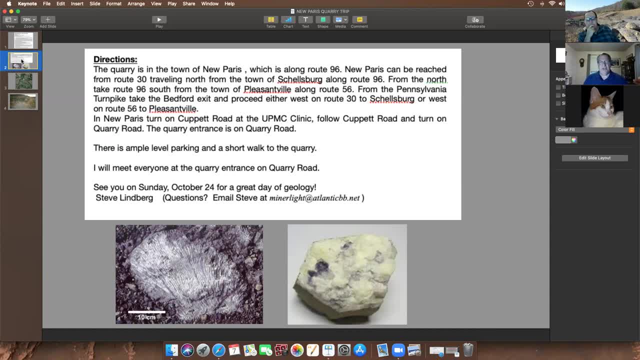 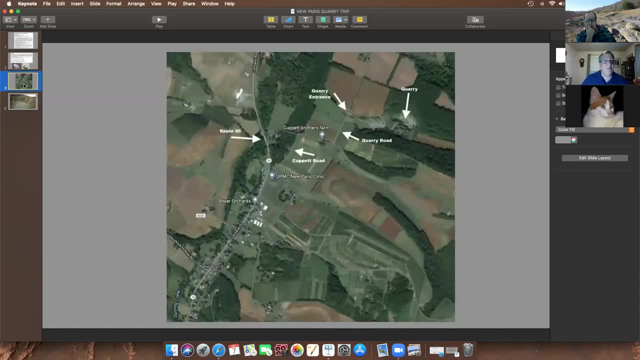 parking. The quarry's changed a little bit over the last five years from the picture I'm about to show you. We'll skip to. we'll go to the map first, real quick. but this is just a quick review. This is off Google Maps. The town of New Paris is a small little hamlet on Route 96, which goes 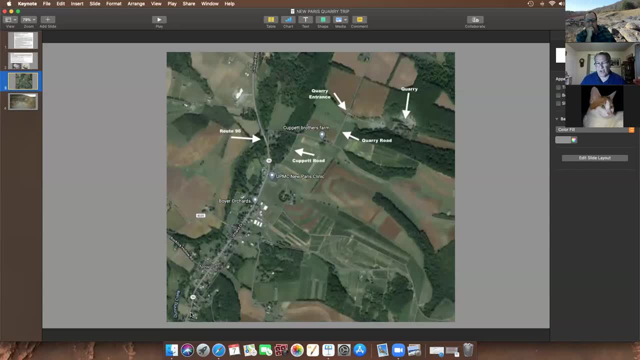 it runs south down to Shellsburg, which is on Route 30 and a couple of miles west of Bedford. If you're coming in on the turnpike from the east or the west, probably the quickest way to get here is to get off the Bedford exit on the turnpike, which is exit 11, head west on Route 30,. 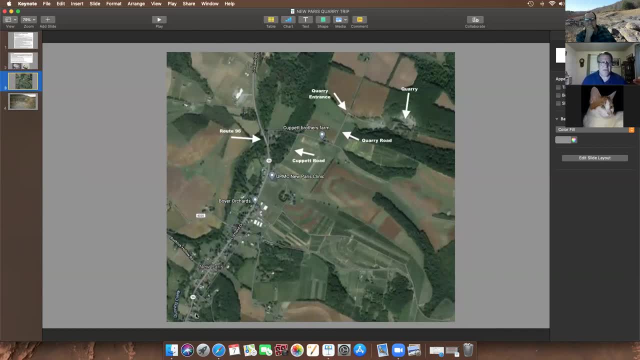 and it's probably not more than a 10 or 15 minute drive till you hit 96 north. You'll come north on 96 till you get to New Paris. As you're leaving New Paris, you'll pass the Boyer Orchards up on. 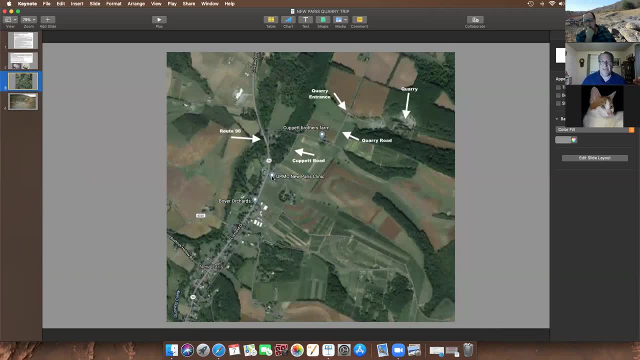 the hill If you're coming in from the south, on the right, and then there's a UPMC New Paris Clinic. I've had several people ask me about an actual address that they could put into their GPS to get them right there. The quarry itself. 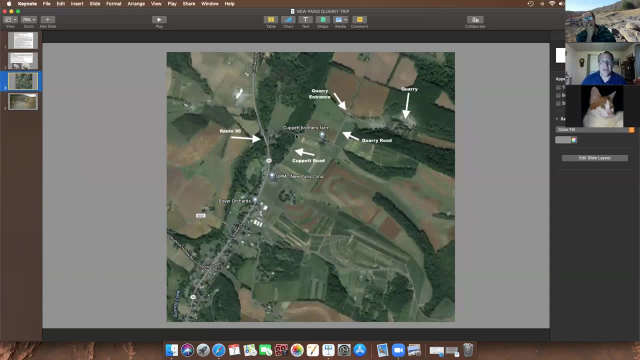 really has no road address, but there is a cup it. This is Cup It Road, the road coming in right here. This is Cup It Road. and then you make a left on Quarry Road, unless you find a way to come in from the north. If you put in Quarry Road, New Paris, PA, as a GPS site, it'll take. 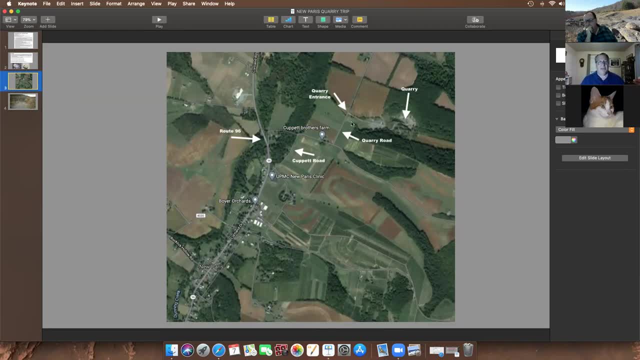 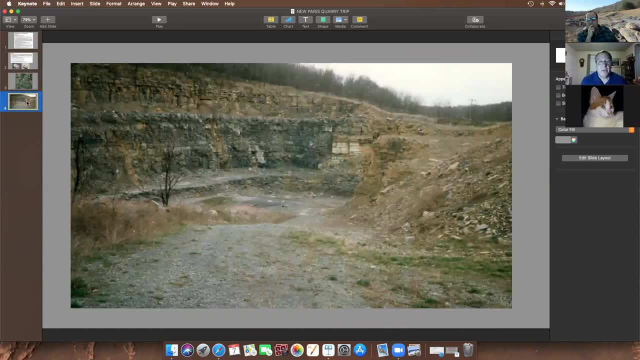 you right to the Quarry Road. The quarry entrance is well marked and that's where I'll meet you. And here's- here's just a view of the quarry from the entrance that I took a couple of years ago before New Enterprise Stone and Lime closed it down. I've decided to sell it privately. It's not an 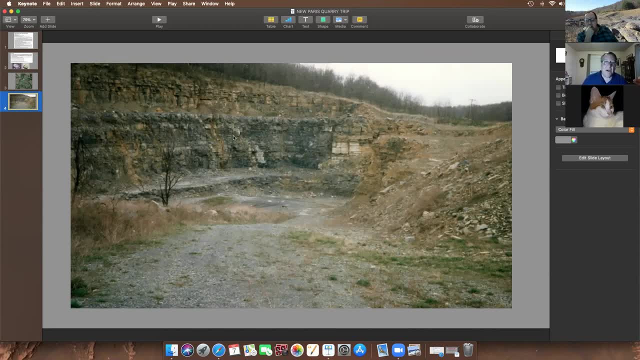 exceptionally large quarry, but it does expose a wealth of fossiliferous limestones and calcareous shales. What New Enterprise Stone and Lime did before they closed the quarry was they blasted down most of this high wall right here, So this part of the quarry is pretty much filled in with 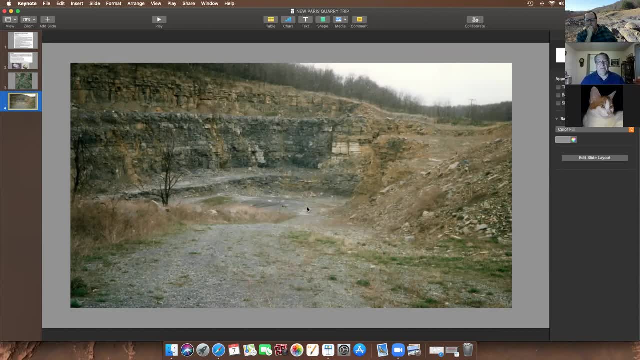 some very large talus blocks, But in a way that was beneficial. beneficial to collectors, because we actually discovered some telsons, the tails of Eurypterids, in these large blocks that were blasted away, The floor of the quarry, and I'll have a geological guide for everyone that shows up at the floor of the quarry. 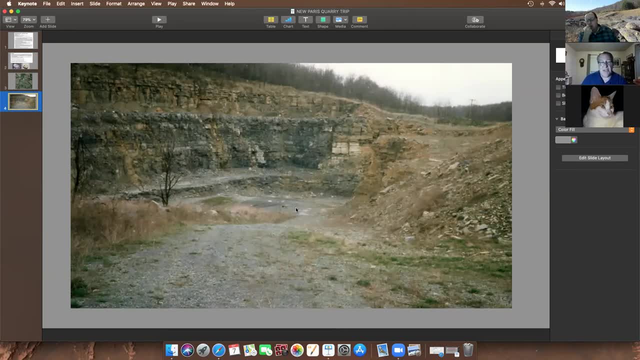 is basically Upper Silurian. This is the Kaiser Formation limestone. So this is Upper Silurian, the Jersey Shore limestone, And then right here at this first bench, which is about 15 feet high, at the top of this first bench, you transition into the Laval limestone, a calcareous limestone. 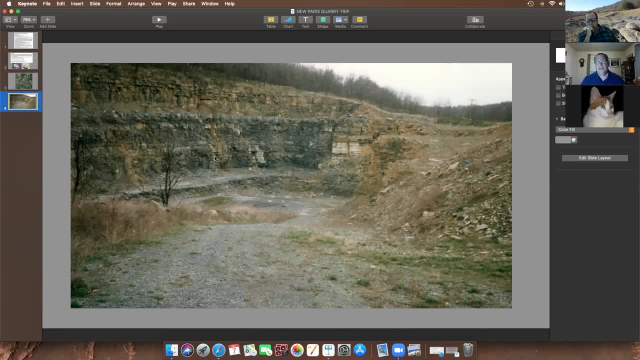 calcareous shale. This is actually Lower Devonian, So the neat thing about this quarry is that you can actually stand on the contact between the Devonian and the Silurian period, or if you're going from older to younger, the Silurian to the Devonian period. Every one of the 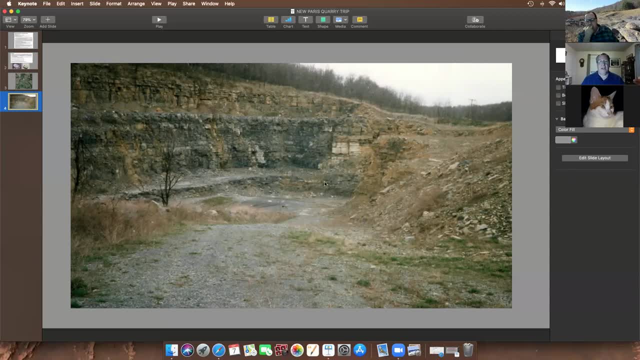 fossils that we'll go over tonight you can find here. If you can't find them in their entirety, you can find fragments of them, just about every one, And then we'll even go to the top bench of the quarry, The top bench of the quarry. we can walk around the edge of the quarry. 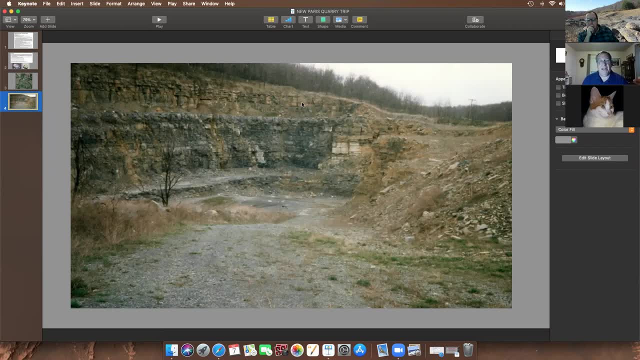 top bench of the quarry exposes the Corriganville and Mandata formations And we actually call this little corner up here- we've kind of nicknamed this trilobite corner, So your best chance of finding a trilobite will be in the talus that's in this. upper corner of the quarry And then we'll go to the top bench of the quarry. we can walk around the edge of the quarry. Top bench of the quarry exposes the Corriganville and Mandata formations And we actually call this little corner up here. we can walk around the edge of the quarry exposes the Corriganville and Mandata formations And we 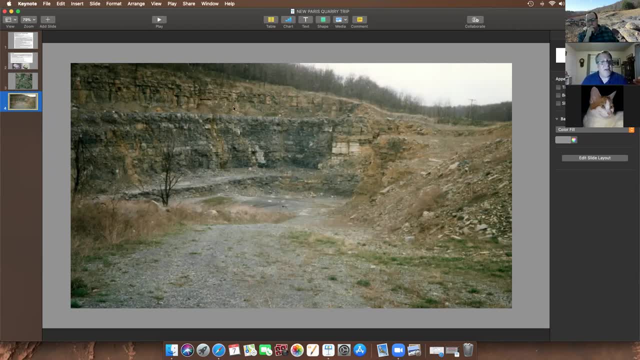 corner up here we can walk around the edge of the quarry exposes the Corriganville and Mandata formations And we. The neat thing about the Corriganville up here on top is you can see this little recessed area right there And that is a bentonite bed which is an altered volcanic ash. So 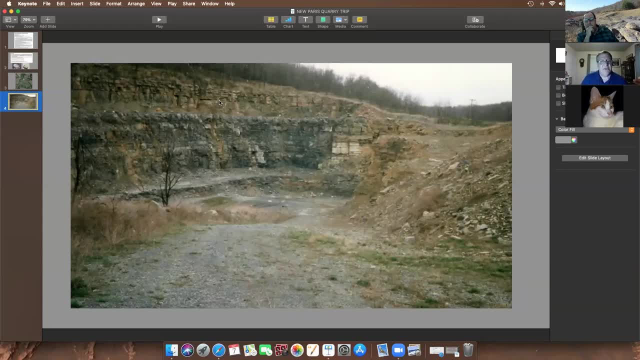 back during the Silurian, end of the end of the Silurian, into the Devonian, the volcanic arc off the east coast of North America. these active volcanoes were depositing layers of volcanic ash on the sun on the shallow sea floor. 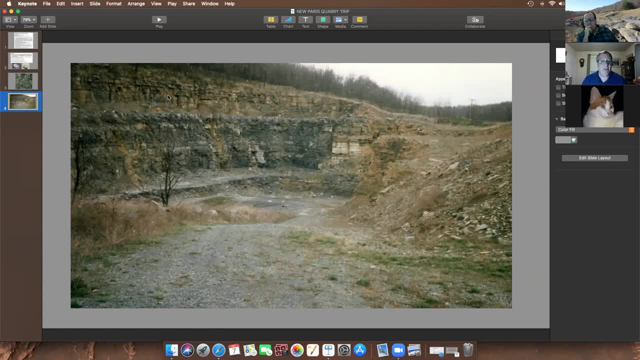 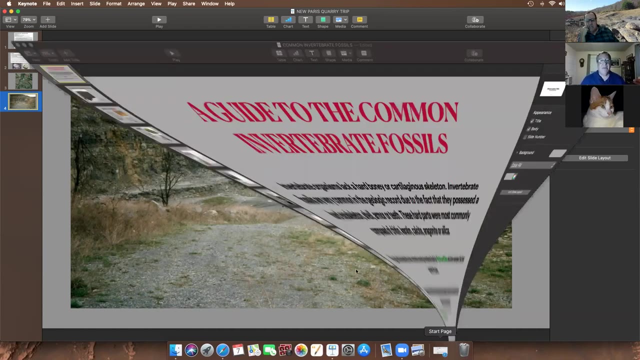 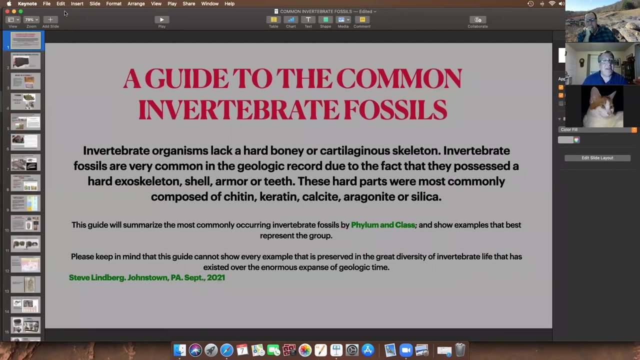 and this volcanic ash can actually be radiometrically dated, So we actually have really really good age dates for for this unit here. So just a little bit of a preview. And there are. there are some pretty spectacular fossils and also other sedimentary features exposed in this quarry. So, with that said, let's go right into. once again, I want to thank everyone for allowing me to speak again tonight. 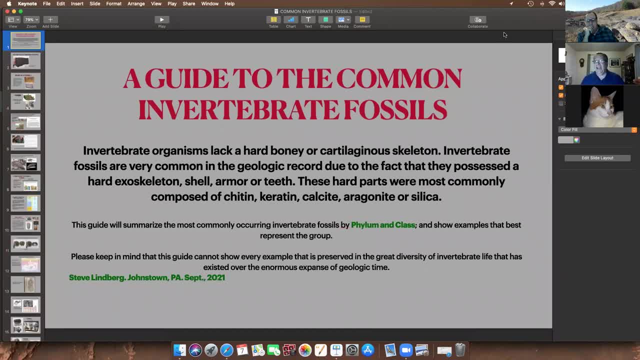 I promise I'll try. I'll do everything I can to be done by eight o'clock Because I know I can get long winded. So tonight's presentation is a guide to the most common invertebrate fossils. So those are real quick. a definition of invertebrate fossils which happen to be fairly fairly common fossils. Invertebrate organisms lack a hard bony or cartilaginous skeleton. 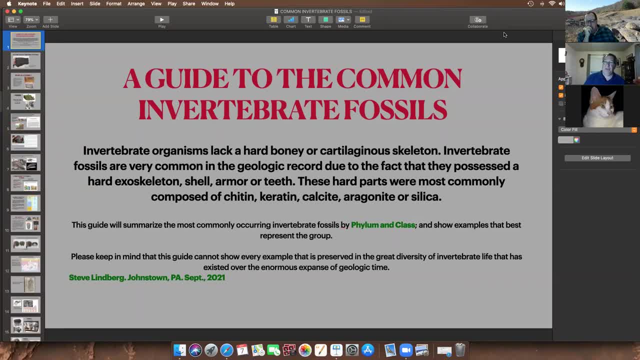 Invertebrate fossils happen to be very common in the geological record, especially in the upper Precambrian, the Paleozoic era. when we get up into the Mesozoic and Cenozoic, of course we find more vertebrate fossils, But for the most part invertebrate fossils. 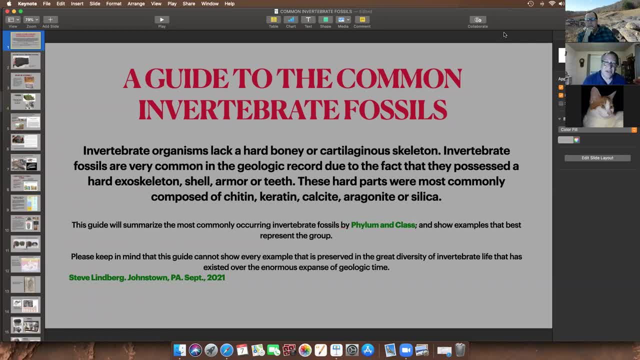 had hard parts that consisted of an exoskeleton, a shell, armor, teeth. The hard parts of a lot of the invertebrate fossils that we're going to look at tonight were composed of chitin or keratin, a material similar to your fingernails- calcite. 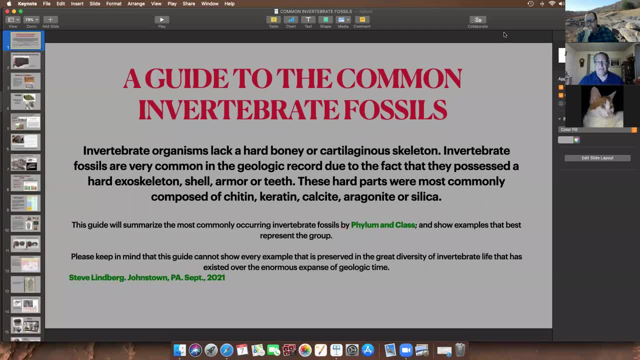 aragonite or silica. So what I've done is I've divided the fossils into categories by phylum and class, And of course this isn't 100% complete and not every class within every phylum is represented, because that would kind of physically be impossible to do unless we spent an entire semester. So tonight we're just going to look at the fauna. 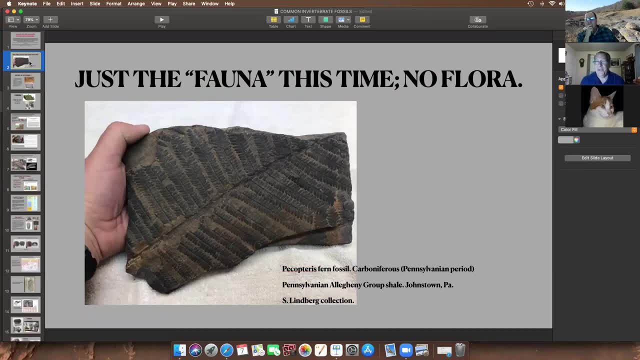 Just the animals, No plants this time. so maybe in the coming year, at a future time, we can look at fossil plants. So we're going to skip the fossil plants. This happens to be a picopterus, a well-preserved picopterus frond from right here about a mile. 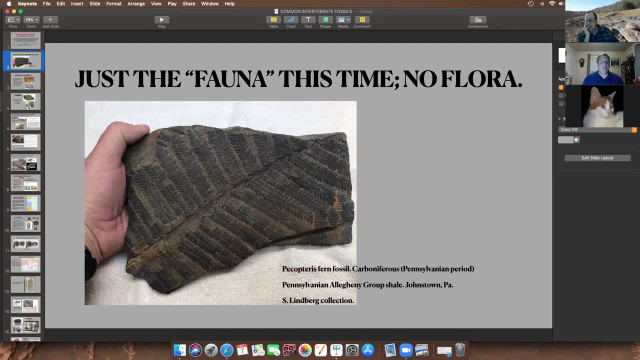 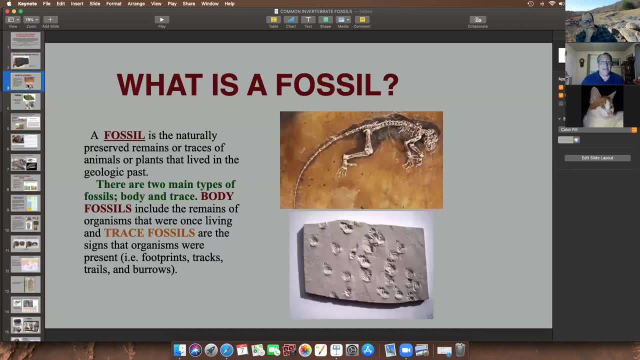 from where I live in Johnstown. This is from the Allegheny group, shales, which dates to the Pennsylvania period. So a quick review. What exactly is a fossil? A fossil is basically the natural preserved remains or traces of any plants or animals that lived in the geologic past. 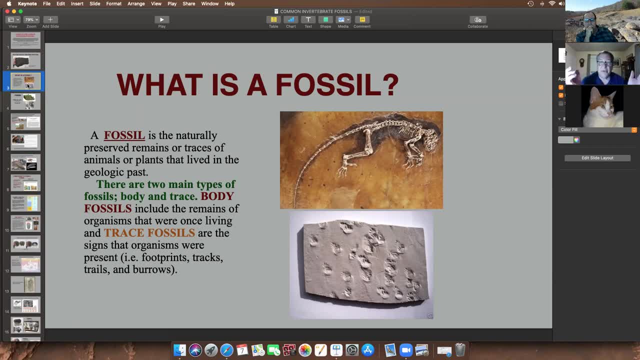 And when we look at fossils, we divide them into two major groups. There's two categories of fossils. The first type of fossil is what's known as a body fossil. A body fossil consists of the entire organism, the entire plant, the entire animal, or part of the plant or the animal. 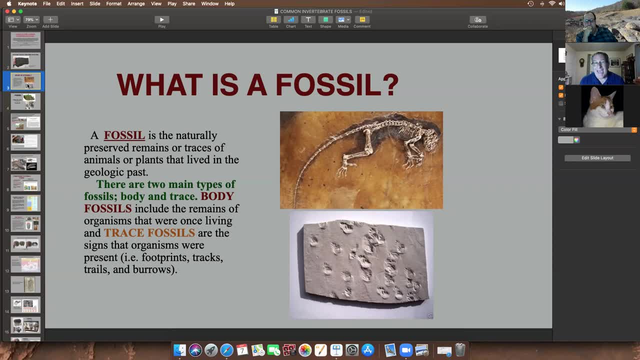 a bone, a shell, a tooth, You have the actual preserved part of the animal's body. The second category of fossils, whether they're vertebrate or invertebrate, are trace fossils. Trace fossils are the evidence that an organism was there, but we don't have the actual organism. We have the footprints, the tracks, the trails. 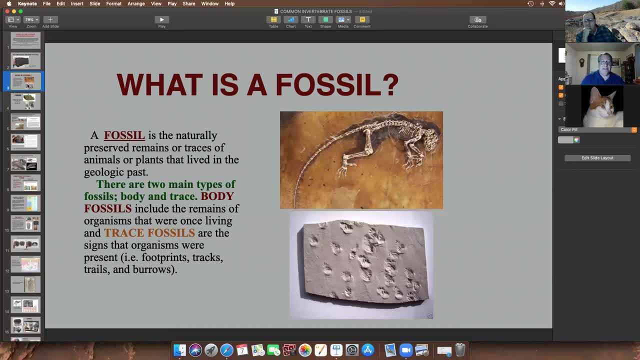 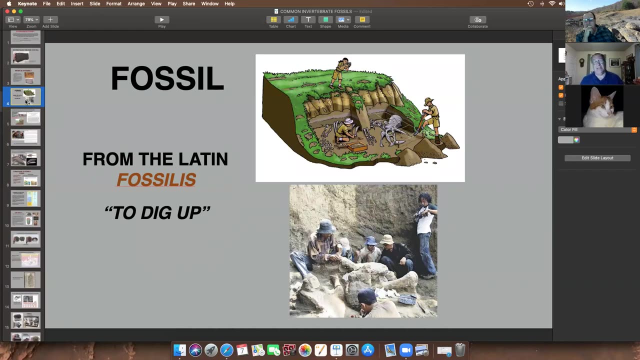 the burrows, a slide, something like that, The coprolite. I love coprolite, So coprolite would be a trace fossil. So what exactly? the word fossil comes from the Latin fossilis, which means to dig up. So basically, unless you're picking them right up off the ground, I guess technically. 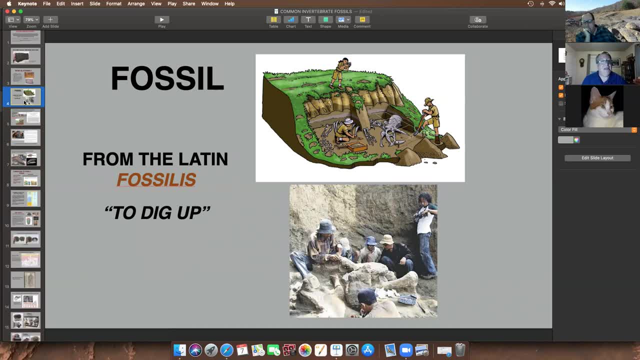 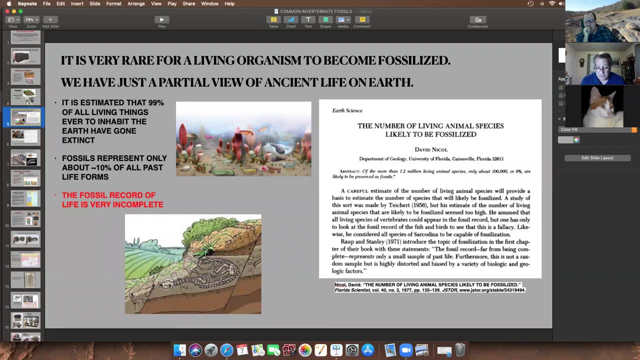 you're still digging them up. So one of the tenets of paleontology that I stress with groups that I speak to and also the students in my class, is I try to impress on them the length of time that living organisms have existed on the Earth and the almost overwhelming 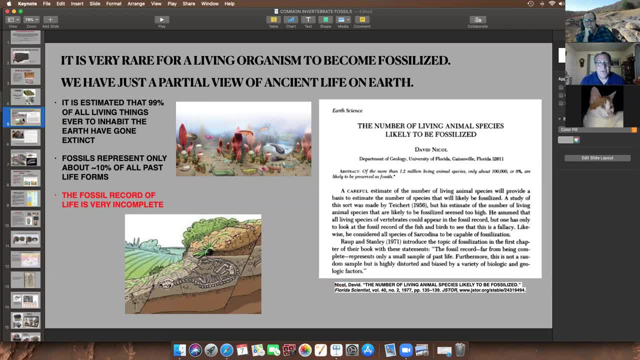 number of organisms, of species that have existed on the Earth, and some persist today, if not as a species, as a class or an order of family. But think about the last two or three billion years of Earth history, And when we first find, we go back. 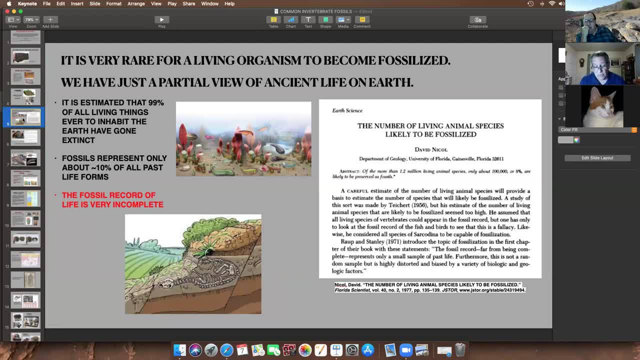 it's the pretermian and we first find evidence of fossilized organisms. Think about this enormous length of time and how many living organisms must have existed on the Earth, And when we look at the assortment and number of different families and orders and species of fossils that we find where. 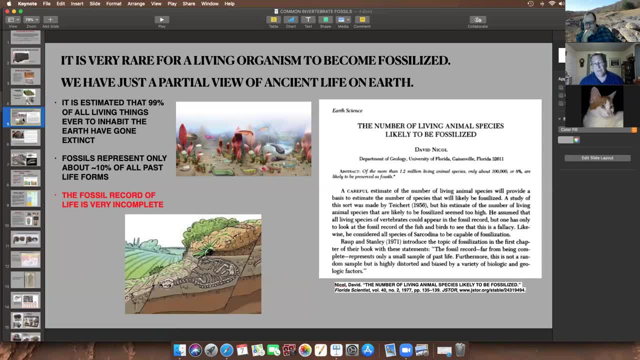 we realize that we're looking through a glass very, very darkly, as a biblical saying goes. We only have a glimpse, an estimate of what the total range of living organisms on the Earth would have been like. We can say with great certainty that the fossil record is very incomplete. We continue to find new. 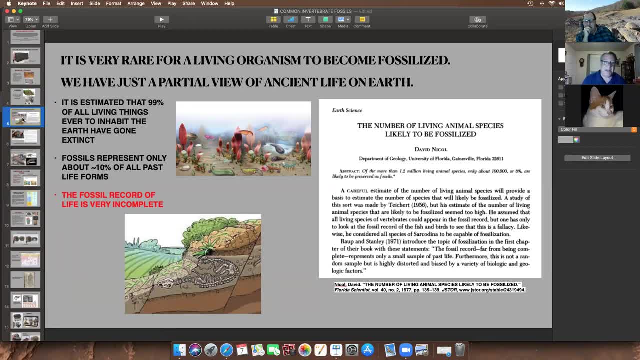 fossils, new dinosaurs, new invertebrate fossils. We continue to make links and find transitional animals, but when we look at the length of time that individual species inhabit the Earth and then possibly go extinct, we know that we have a very incomplete picture of organisms that have come and 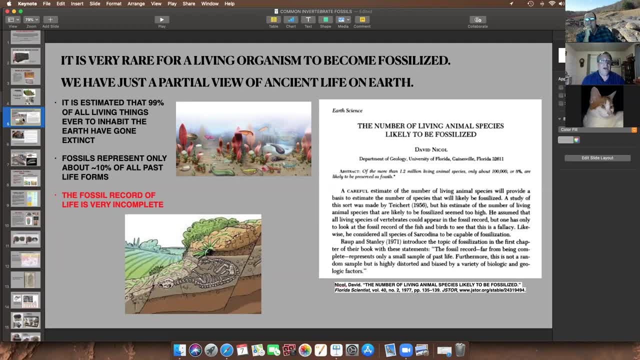 gone, evolved and disappeared on the earth, And we may never know. Paleontologists estimate estimate one of the statements I have here. paleontologists estimate estimate that 99% of all living things to have ever inhabited the earth have gone extinct And out of that, 99%. 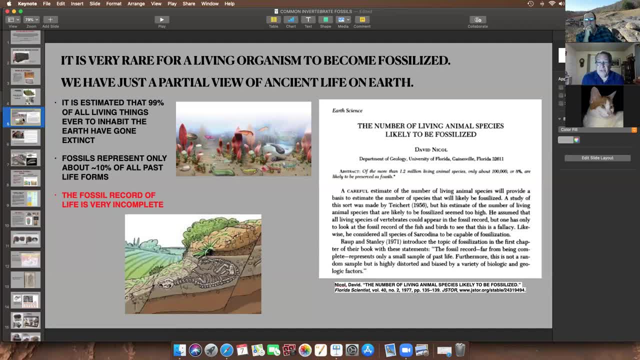 of organisms. we only find a small percentage of them And I've copied in another little highlight here, kind of the abstract from a text, And this is from David Nickel at the Department of Geology University of Florida in Gainesville, And one of the statements: 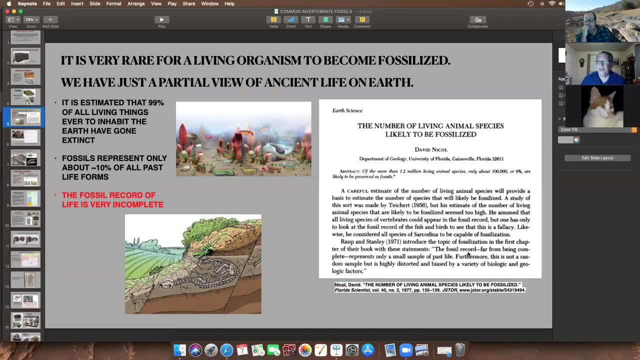 well, he quotes from a previous paper- is that the fossil record, far from being complete, represents only a small sample of past life. Furthermore, this is not a random sample, but it's highly distorted and biased, based on a variety of biologic and geological factors. So when we look at fossils, we got to realize we're looking. 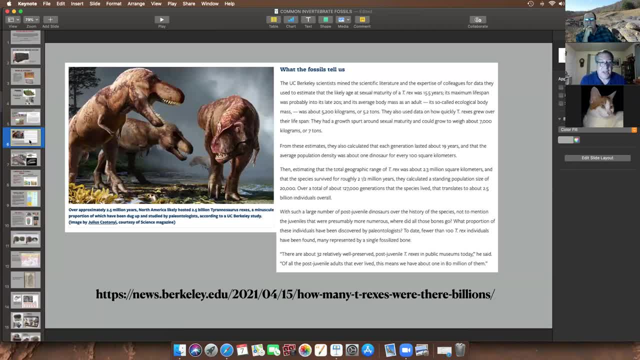 at a very skewed view of what ancient life on the earth would have looked like, And I couldn't move on to invertebrate fossils without first mentioning this. This had made the news last year. I made it for some interesting reading and this has continued. 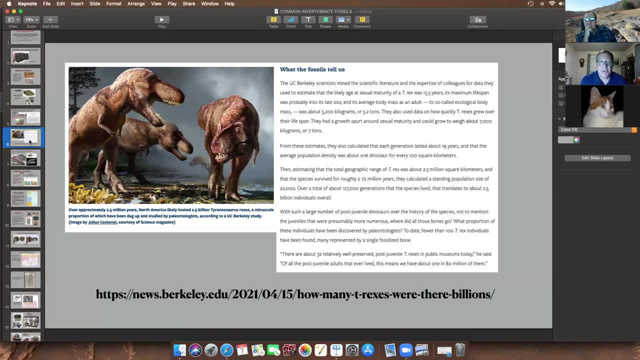 To undergoing a study, but Tyrannosaurus rex, for example- not an invertebrate, but if you mention a dinosaur, most people know T-Rex. We're seeing a lot of new studies now where we're estimating the total number of individuals that may have inhabited the earth over the range of 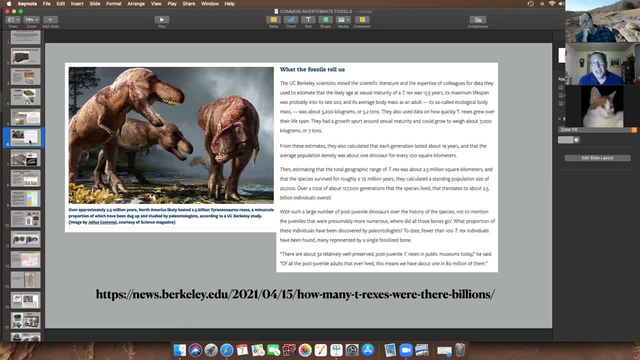 their existence, Tyrannosaurus rex had a very brief period in which they roamed or inhabited the earth. We know that T-Rex was only around for about 2%. It's still a long time, but relatively short on the geological timescale, Well over the 2.5 million. 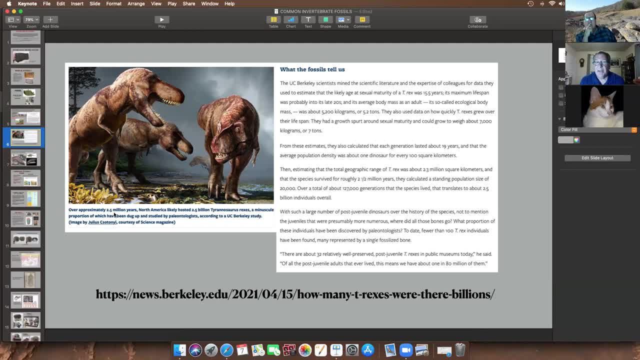 years that T-Rex inhabited the earth. based on fossils that we find, they're estimating that at any given time there would have been a standing population of 20,000 individuals. So what that means is, if we could go back to the last year, we'd be able to estimate that at any given time. we would have seen a population of about 20,000 T-Rex at any given time. If we multiply that out over the length of time that T-Rex existed, we get a number of about 2.5 billion, I mean. 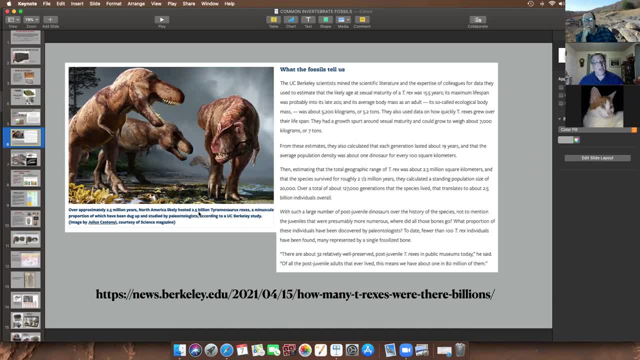 imagine that. That's like staggering. So over a geological time period of 2.5 million years, 2.5 billion T-Rexes inhabited the North American continent. So if there were 2.5 billion T-Rexes? 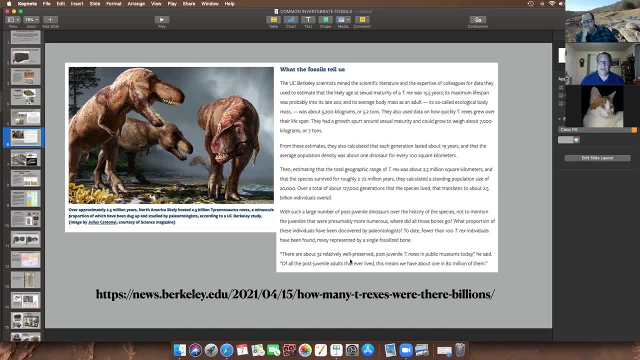 how many well-preserved fossils do we have? Well, you look at the bottom of this little insert. there were only about 32 well-preserved post-juvenile T-Rexes in public museums today. That's about one out of 80 million. So even though T-Rex is a very popular fossil, 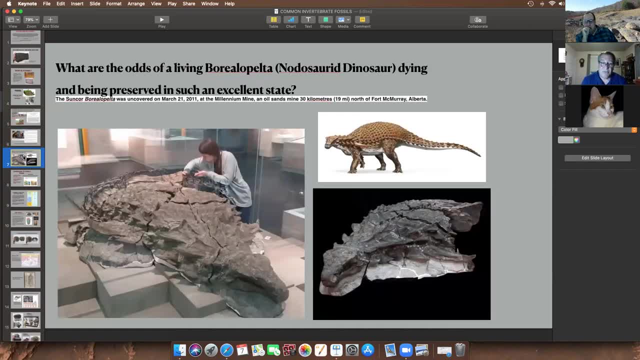 we only have a brief glimpse of what it was really like. Most of the T-Rexes that inhabited the North American continent died and disappeared without leaving any fossil trace, And I wanted to mention this, too, before going on to the invertebrate fossils, the recently discovered. 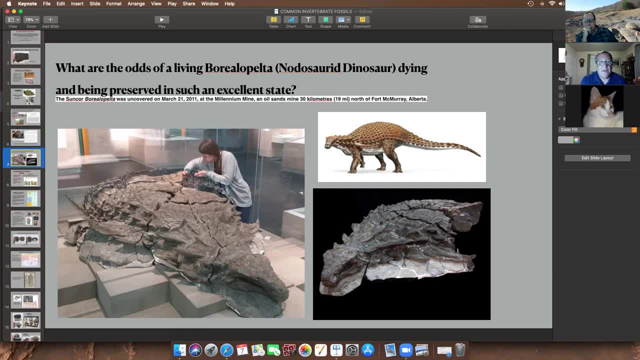 nodosaur, the Boreala pelta that was found at the Suncor tar sands mine in Alberta. that incredibly preserved nodosaur the armored dinosaur. Think of the odds of something like this dying and being preserved, and especially being preserved in this fantastic state of preservation. 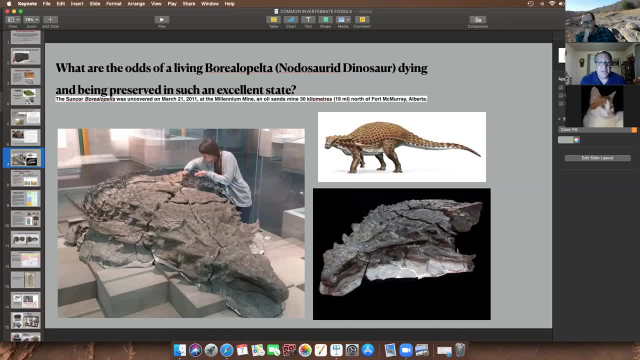 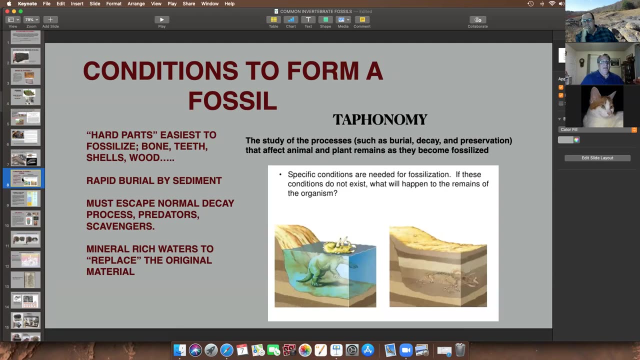 where we've even been able to detect color in the plates on the back of the dinosaur. This probably ranks as one of the most outstanding dinosaur fossils ever discovered. But let's go on. Let's move on to the invertebrate fossils. So something else just to go over very quickly. 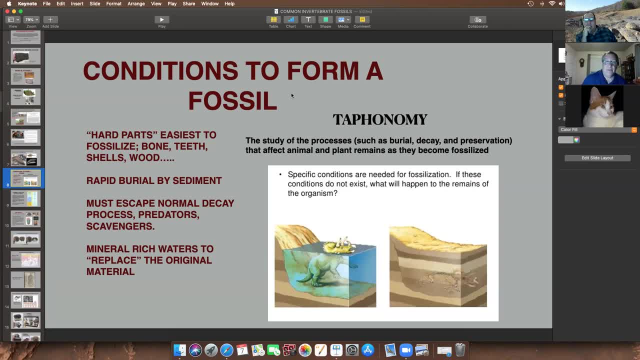 is, the conditions for something to form a fossil in most cases are pretty unique. What makes the best fossil? Well, hard parts. If you have hard parts- bones, teeth, shell, wood, calcite, silica parts- they will be preserved the easiest. 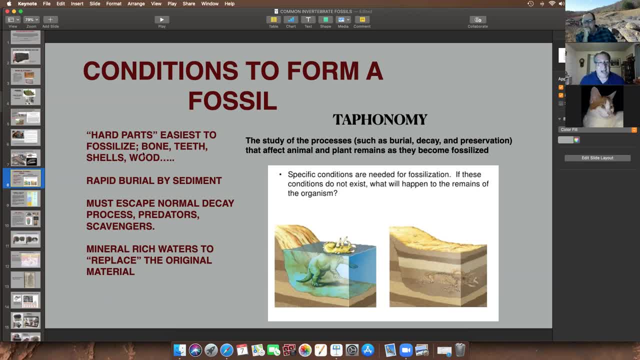 Typically, after an organism dies, we look for it to be buried very rapidly by sediment. We want the organism to sink into mud, We want it to be covered by a landslide or some type of rockfall. We want it to be buried in silt or in tar For the organism to be fossilized completely. 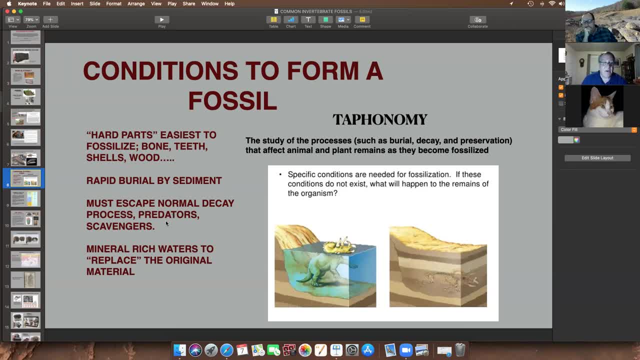 it must escape the normal decay process most of the time. We want to avoid predators and scavengers that die. We want to avoid predators and scavengers that die. We want to avoid predators and scavengers that die. We want to avoid predators and scavengers that rip the organism apart and scatter the parts. 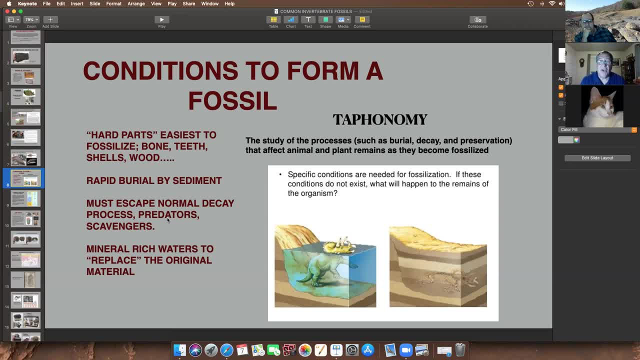 We want an environment that tends to be quiet, where the entire organism will settle to the bottom and be preserved. And then, probably most importantly, there's lots of different methods of fossilization, But normally animals, invertebrates, invertebrates- are fossilized. 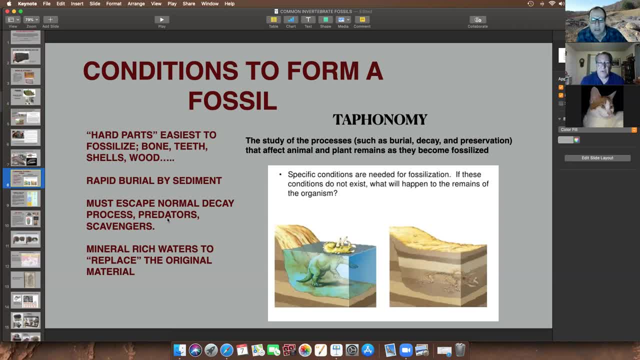 by the process known as replacement, where the original material dissolves away and it's replaced, molecule by molecule, with minerals that are in mineral-rich water. So you know poor, Mr Triceratops here, or for us, not so poor, because that's why we have the 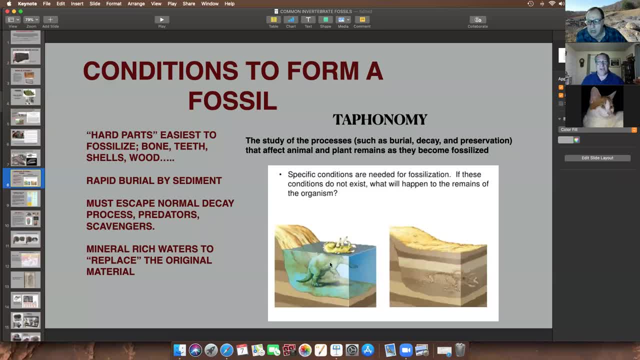 spectacular fossils of Triceratops. Triceratops or another organism- slips into a body of water and he drowns. He sinks to the bottom, Predators and scavengers can't get to him, He's rapidly covered by sediment and the magic of fossilization takes place. The science of studying what happens. 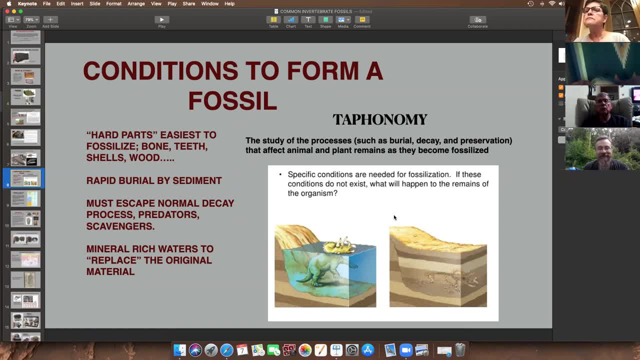 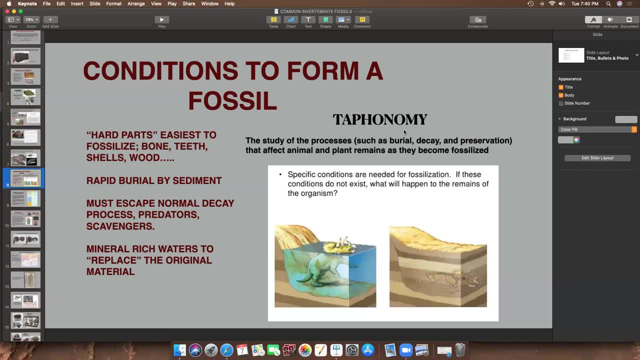 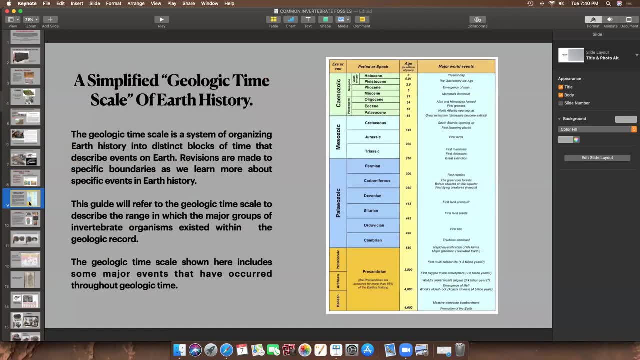 studies the process of fossilization and what happens during burial decay and preservation. So the invertebrate fossils I'm going to show you will be keyed out. I'll explain to you when they existed, what their geologic range was, from like pre-Cambrian to pre-Cambrian. 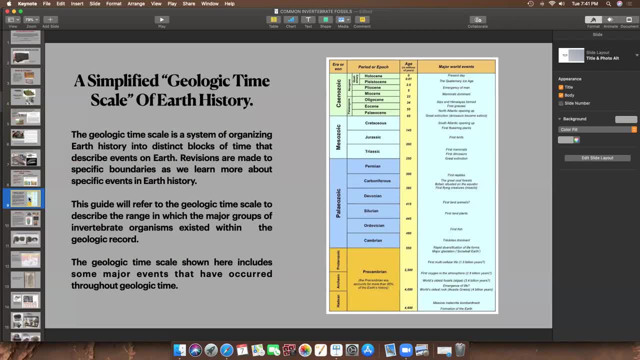 So we're all familiar with the geologic timescale. I'm not going to take a great deal of time to go over this, But one of the things I noticed when I put this timescale up- obviously this is from a European country. 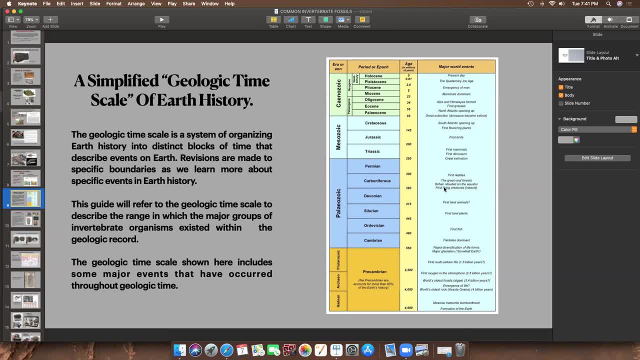 because right here it mentions the great coal forests of Britain and they have the Carboniferous and it's not subdivided into the Mississippi and Pennsylvania, So European geologists like to just call it the Carboniferous here in North America. 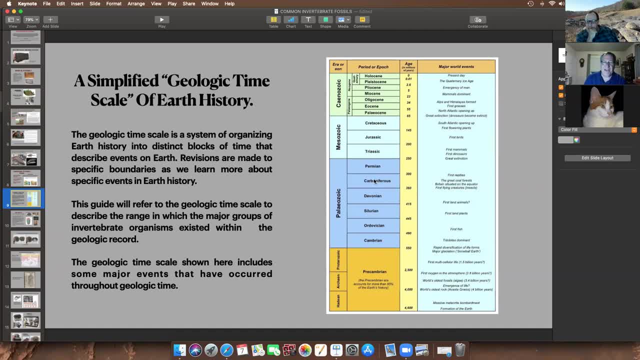 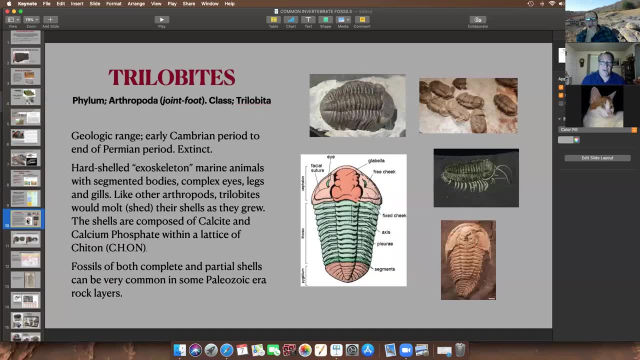 They like to swing out the Mississippian and Pennsylvania. So let's look at the invertebrate fossils. So we'll start with what has to be pretty much everyone's: Trilobites aren't your favorite invertebrate fossil. 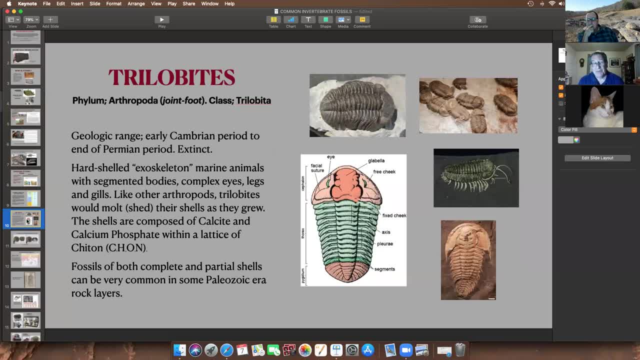 Maybe after we go to the New Paris limestone quarry and you find a couple of really neat trilobite Pagidiums or Cephalons or possibly a whole trilobite. maybe they will be So trilobites. 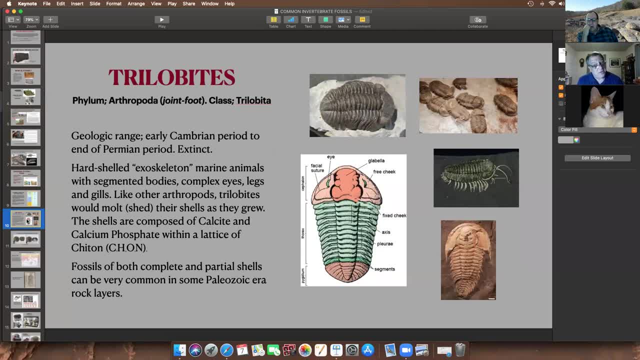 an exceptional invertebrate fossil. They're an important invertebrate fossil for a lot of different reasons. They're fairly common. We know of thousands of different species. Trilobites belong to the phylum Othropoda, which is from the Latin means jointed foot or hinged foot. Trilobites are in their own class. 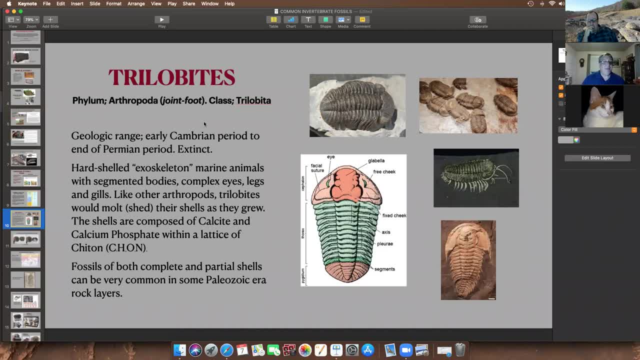 They're class Trilobita. The geologic range is we begin to see trilobites from the early Cambrian period. They were victims of the Great Dying at the end of the Permian, but during the Permian period. 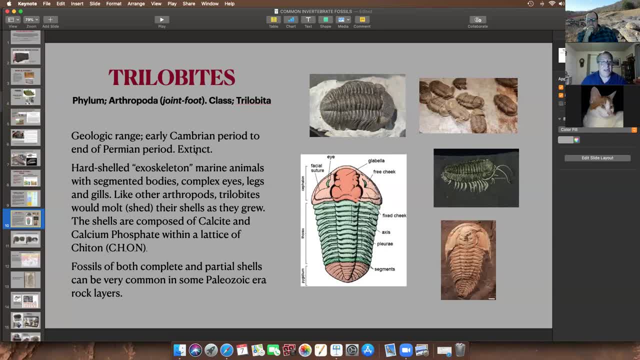 they were already on great decline. Trilobites today are extinct. The typical trilobite was covered with a hard exoskeleton. It had. these were marine, exclusively marine, saltwater animals. They had segmented bodies, very evolved, complex eyes, legs and gills. 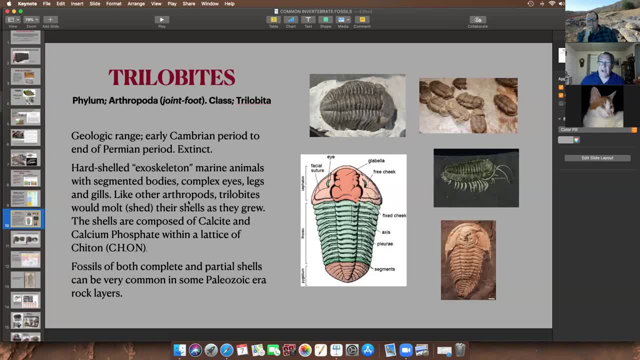 Like other Othropods, trilobites would move to the east of the continent. As a result, they were identified as a species of the marine molt their shell. The shell does not grow. The animal grows and then the shell gets too small. 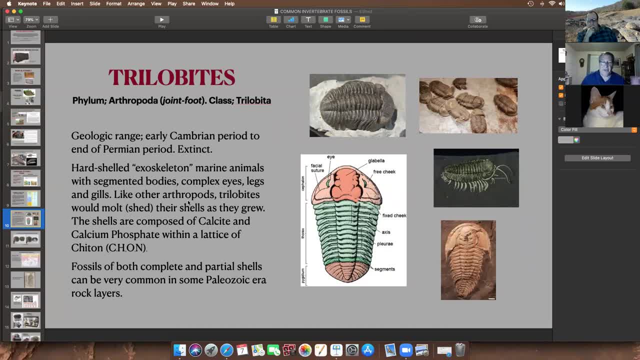 and they split out of the shell. The shell will sink to the bottom or be munched on by predators for the little bit of tissue that might be left in it, And then the animal, over a period of several days or weeks, hardens a new shell similar to crabs, lobsters and other arthropods. today, 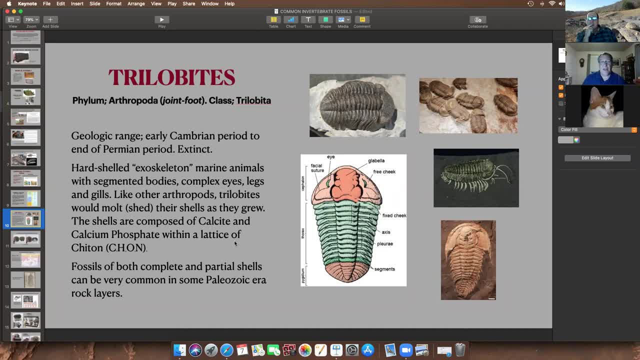 Uh trilobite shells were composed of calcite, calcium phosphate, within the lattice of chitin Um. and not to get into a lot of chemistry here, but the basic formula for chitin um, chitin, is actually a type of a polysaccharide. So uh trilobites are found as both complete and partial. 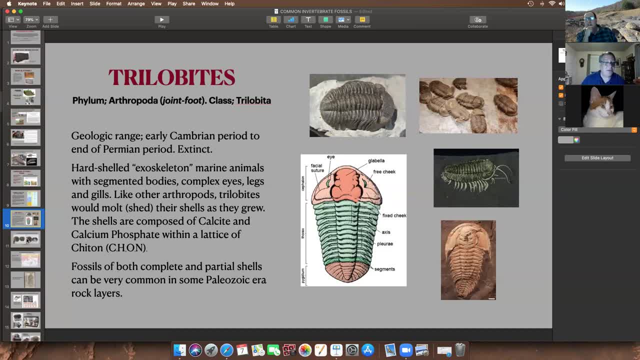 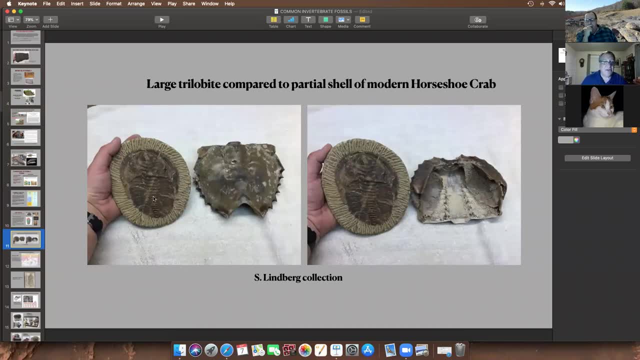 shells. They're very common in paleozoic rock layers. Uh, here's a um. I included a lot of photographs of the fossils from my collection. Here's a large trilobite, partially restored. This is from Morocco, Uh, and here is uh from down by um Ocean City. Here's uh part of the uh shell of. 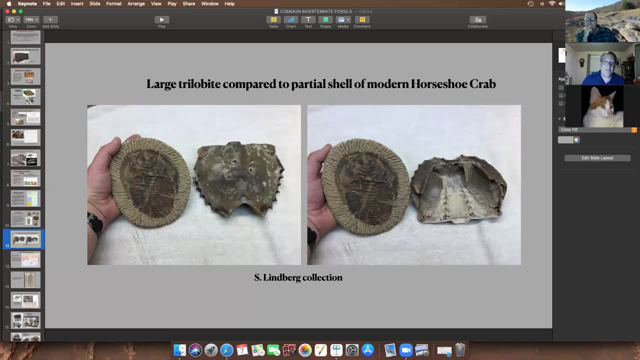 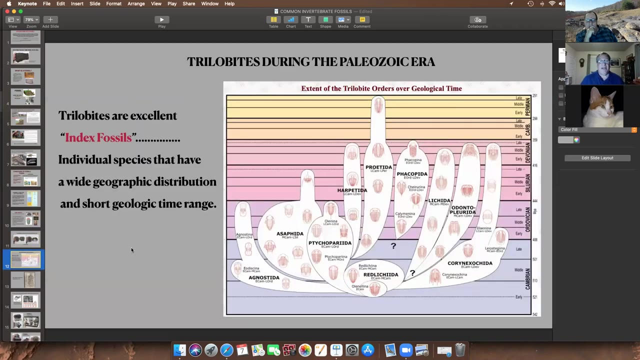 a horseshoe crab, which is often called a living fossil, not really related to a trilobite, but we can imagine if you've ever seen a horseshoe crab shell uh down on the beach, the same type of material uh probably made up the shell of a trilobite, Um trilobites. 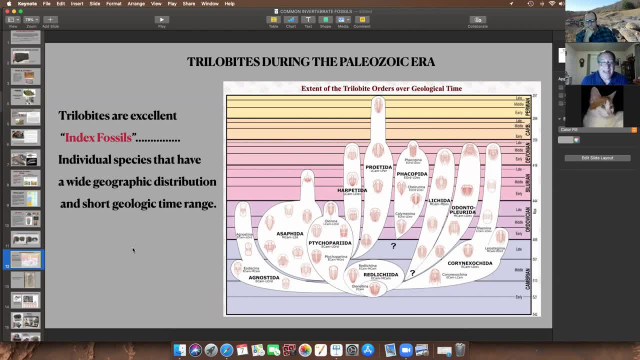 uh, make excellent index fossils. Uh, an index fossil is a fossil that tells you pretty much what geologic period uh, or epoch or stage uh, you're working in. Uh, trilobites evolved very, very rapidly. Um, at the beginning of the Cambrian period they had a very, very rapid evolution. 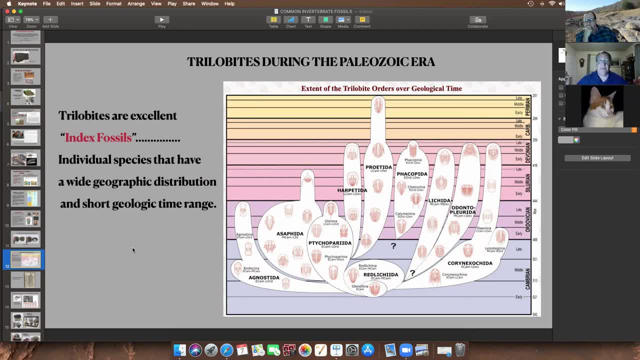 um, and they diversified into different families very quickly. So we can, um, we, depending on the type of trilobite that we find, uh, we know, uh, what the age of the rock layers are that we're working in, Uh, so the definition of an index fossil is an index fossil. 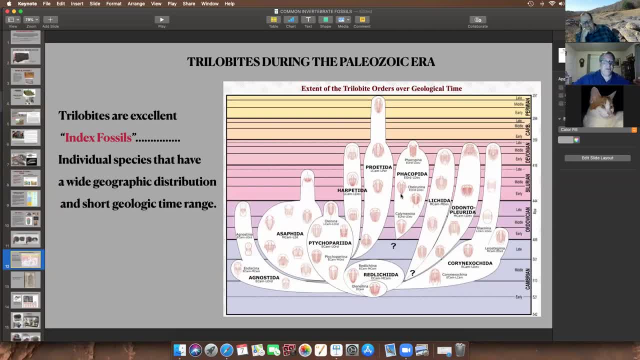 is a fossil that should have a wide distribution. You find it across a large geographic area, but it only existed for a short period of time. Uh, T-Rex would be a good example of that. When you find a T-Rex uh fossil uh in place in situ. 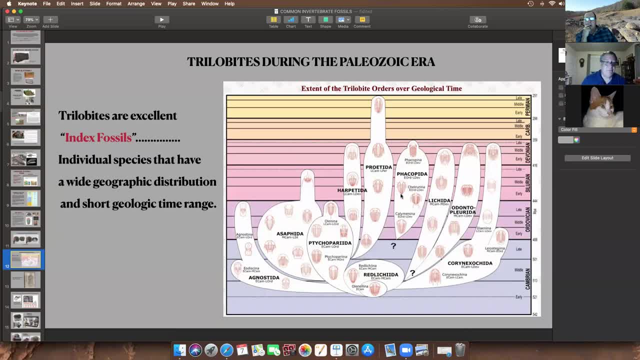 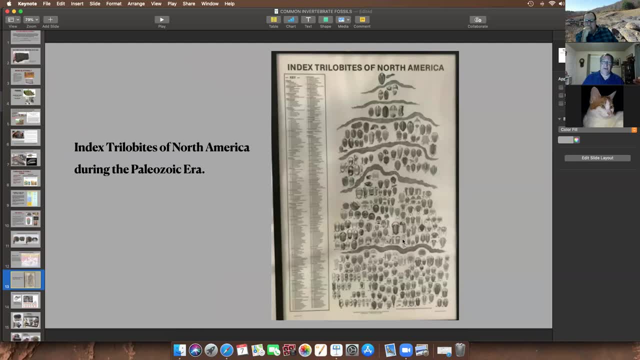 rock. uh, you know, you know that you're looking at that 2.5 million year time period. Um, here's- uh, I've got to get a copy of this poster. Unfortunately, I don't have one, but these are index trilobites of North America. Um, these are all of the important trilobites. 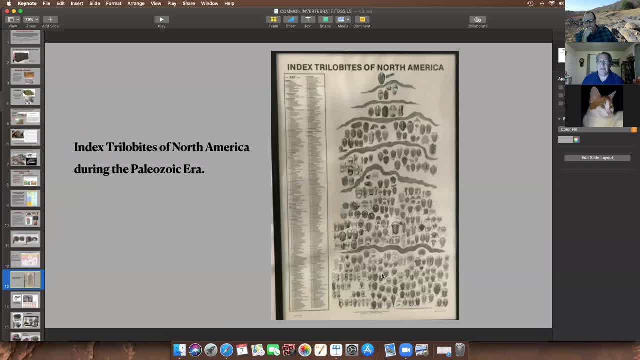 that we find here in North America. I think these are subdivided by- it might be by family- um beginning with the uh Cambrian period. So these are all of the uh Cambrian trilobites. 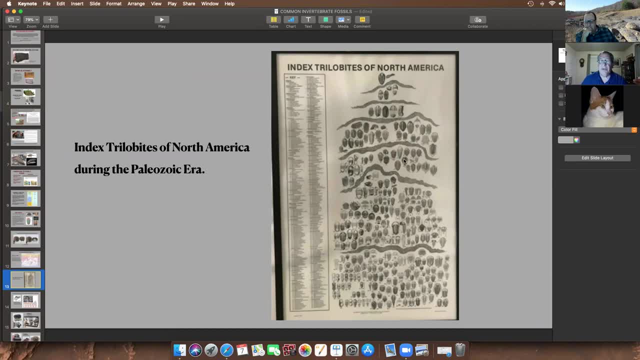 Cambrian, uh Ordovician, Silurian, uh Devonian Mississippian. and you can see that by the end of the Paleozoic era trilobites are going undergoing a huge decline. uh Mississippian. 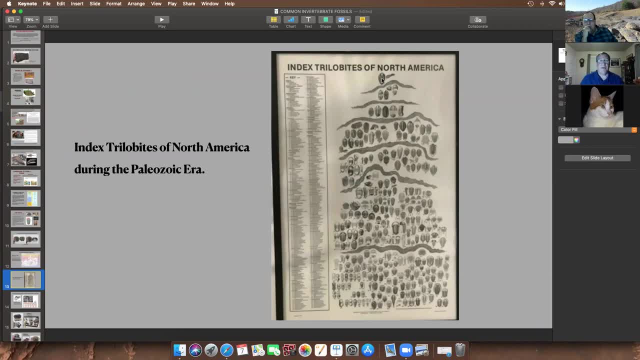 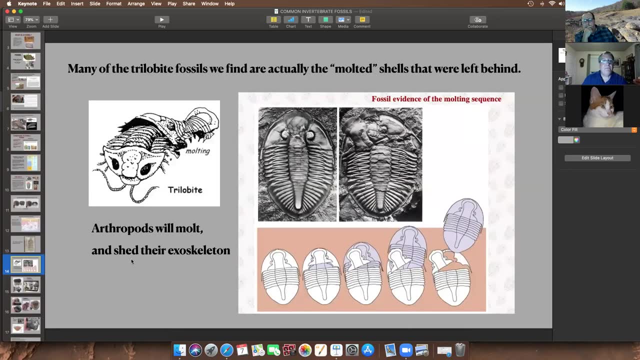 Pennsylvanian and then finally Permian. So by the time you get to the Permian period, um, you only have one or two species of trilobites uh remaining. Um, many of the trilobite fossils that we find are actually molted shells that were left. 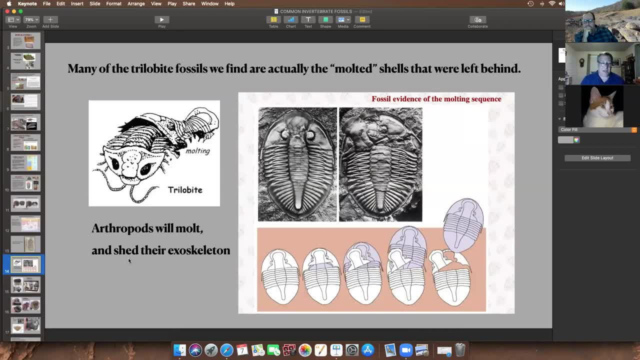 uh, I'm going to say the majority of trilobite shells that we find. Uh, if you think about it, when you find a, when you find a fossil trilobite, there's really only two possibilities: You. 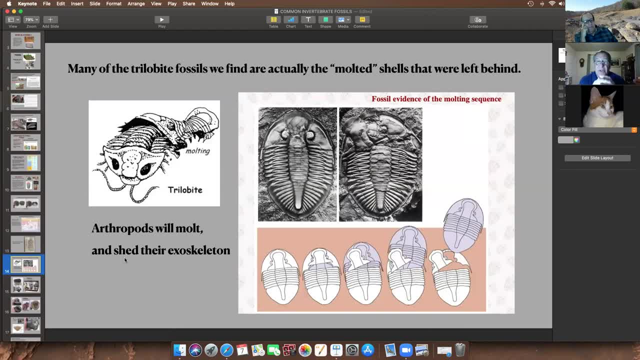 you have the actual animal that was died quickly, maybe in a underwater, uh, landslide, or a mudslide, or a poison, uh, a small little area like at high tide that dried up. So you either have the entire animal, um, or you have a molted shell, Um. so 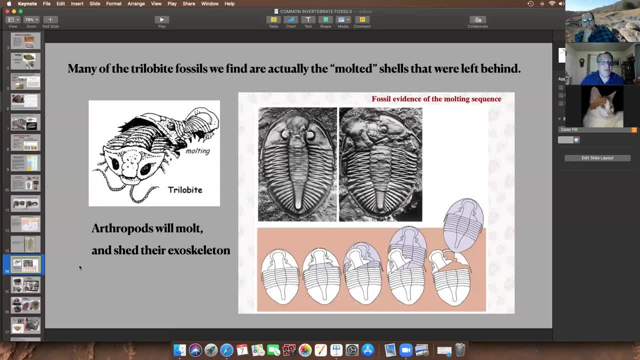 usually most of the shells that we find of trilobites are molted And and a lot of times there's a way that you can tell, uh, when trilobites molted uh the cephalon uh had. 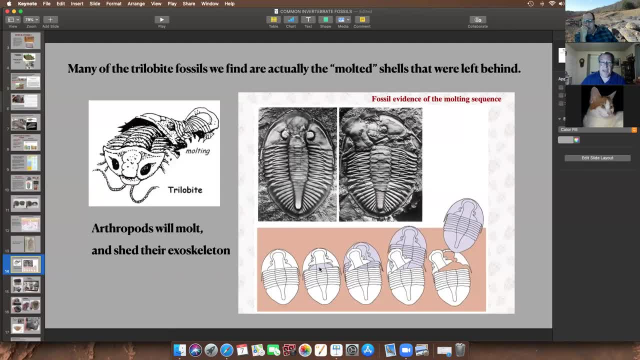 weak points in it, called the free cheeks, And what would happen is that's where the shell would split and the uh cephalon, the glabella, would usually tip to the side and the trilobite would wiggle out of that shell and leave the shell behind. So a lot of times we find trilobite fossils that look 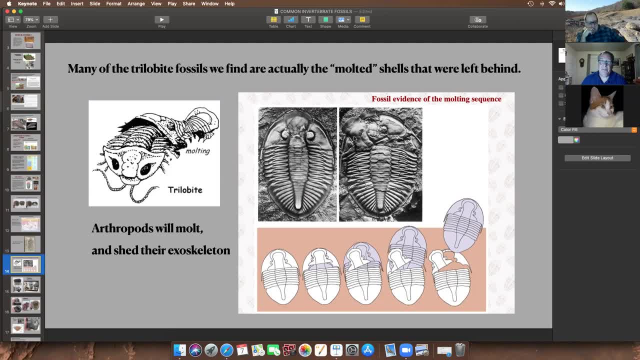 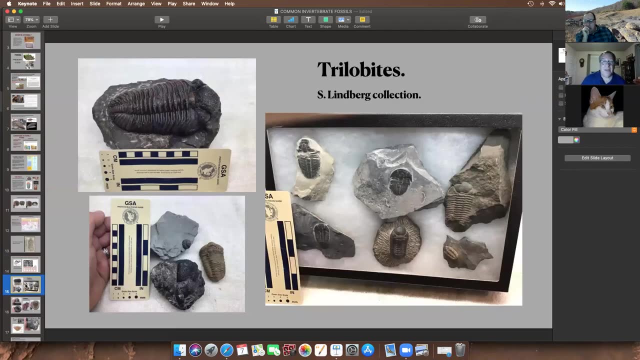 like a molded shell. So you're seeing, the um cephalon has separated from the rest of the thorax and the trilobite has crawled out and gone his way and that shell sank to the bottom and and became fossilized. So, uh, here are a couple of trilobites, uh, from my own collection. 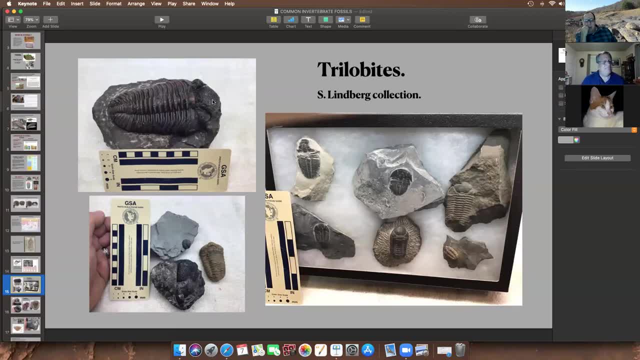 I believe this is a drotops from, uh, the Devonian of Morocco. Um, here's what I just call it a flexi. This is from the Ordovician of Ohio. Uh, this is a uh. this is a uh, this is a uh. 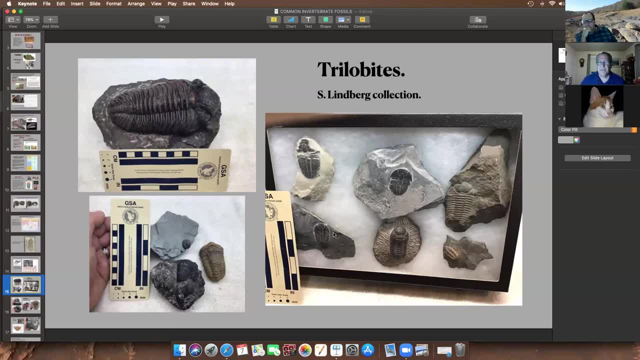 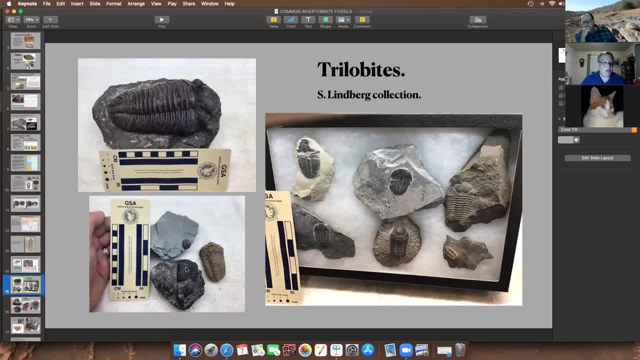 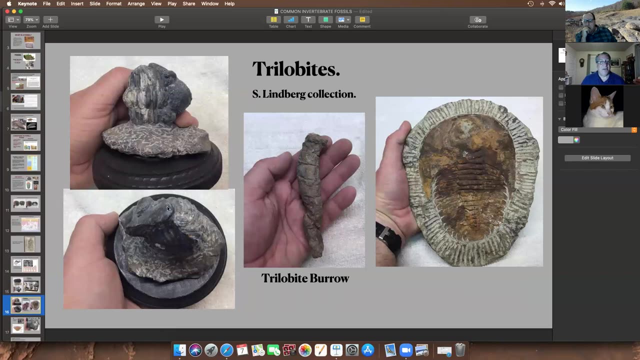 in Pennsylvania, Another one from Morocco. Uh, here's a large coiled Moroccan trilobite. You're kind of looking down at his glabella, the beak of his nose, and here's his left eye. Um so, uh, here's another view of that that previous trilobite. So this one is mounted on a 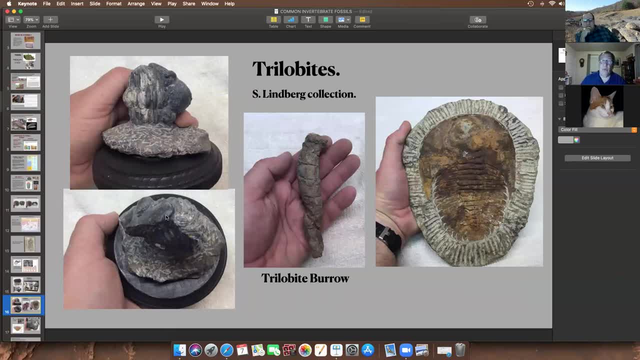 wooden platform. Uh, trilobites would occasionally burrow into the mud. Um, they would burrow down into the mud looking for food and we occasionally find- at least this is what we think they are. here's a trilobite trace fossil. This is from down. uh, it was from I. 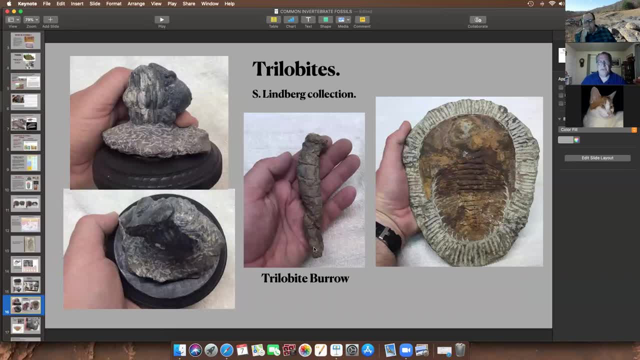 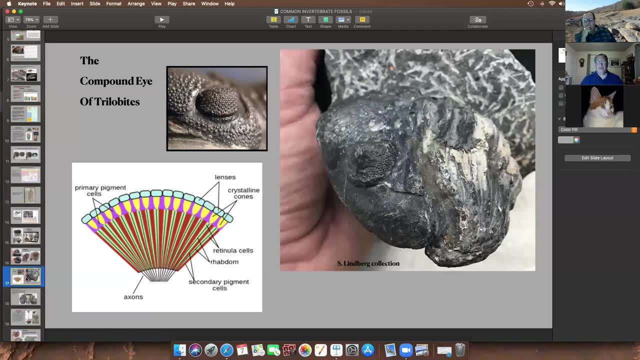 believe it's from down in West Virginia. Uh, so this is a burrow that was recovered um from a trilobite that had burrowed down into the mud. Um, trilobites had incredibly evolved eyes. 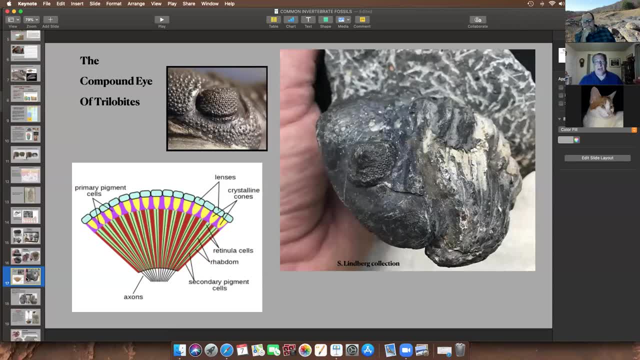 Um, as a matter of fact, the eyes of trilobites uh are used to classify them. there were different uh different groups of trilobites based on whether they had a single cornea or separate corneas, but the trilobite eyes were made of crystalline lenses usually. 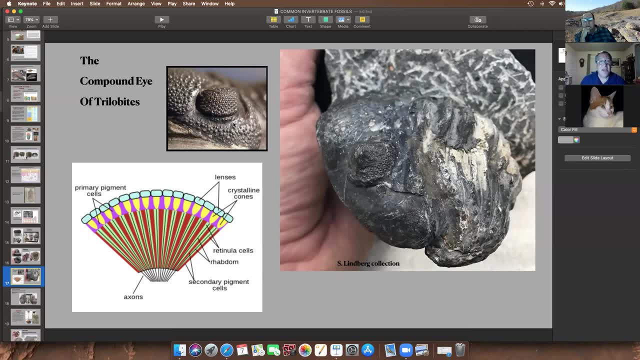 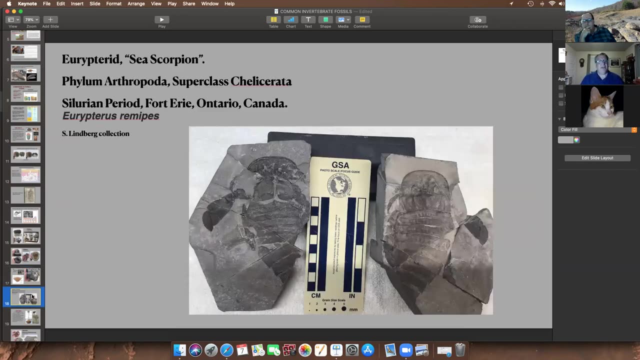 calcite lenses and they were faceted like the eyes of insects and occasionally, if you have a well-preserved trilobite- uh, this one from my collection- you can see those beautifully faceted individual eyes cells. um, i didn't, uh, i didn't want to spend a lot of time on this one, but 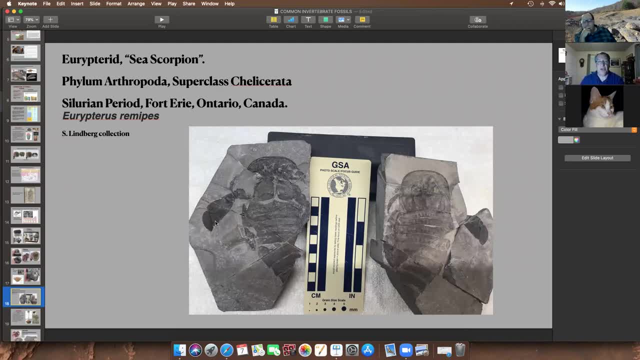 another arthropod that makes spectacular fossils are the eurypterids, or sea scorpions. another jointed uh arthropod with a hard kite in the shell. uh, eurypterids are are typically salurian period. uh, this happens to be one of my better, better finds that i've had in my collection for many. 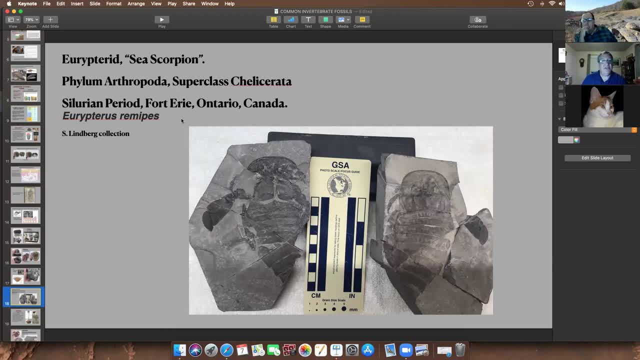 years. this is a eurypterid, uh remipedes. this is from the salurian period up in fort erie, ontario, canada. we were splitting apart the limestone and i broke the piece apart and wow, there he was, um, unfortunately, the other pieces. this was on the edge of a little outcrop. the other pieces. 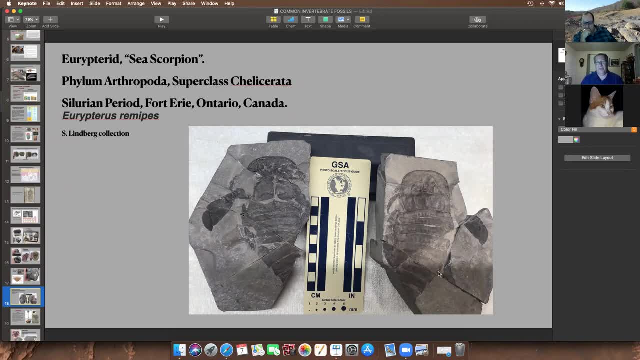 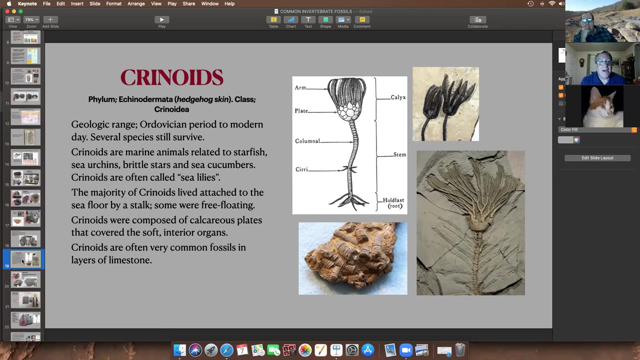 telson and the tail was missing, but i was. i was more than pleased just to find that much the positive and negative of the uh eurypterid. so those are the trilobites. all right, now we have the um, we have the crinoids, uh, spectacular uh, echinoderms, uh, trilobites, uh, i'm sorry. 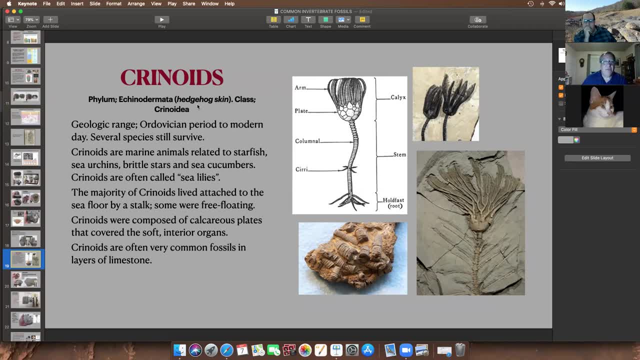 crinoids are in the phylum echinodermata, uh, which means hedgehog skin or spiny skin. they're in their own class, class crinoidia. uh. they thrived beginning in the ordovician period and many species still survive today. uh, they are um echinoderms. they're related to starfish sea. 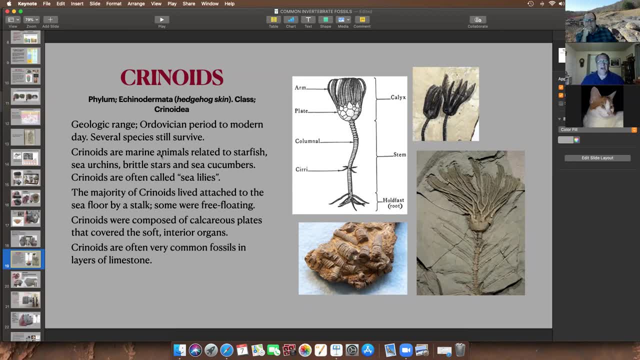 urchins, brittle stars, uh, sea cucumbers. uh, the majority of crinoids resembled, uh, plants, kind of like a flower, but this is actually a, a living echinoderm. uh, some of them grew up to four, five, six feet in height, or larger. typically they were. a typical crinoid is within maybe five to six. 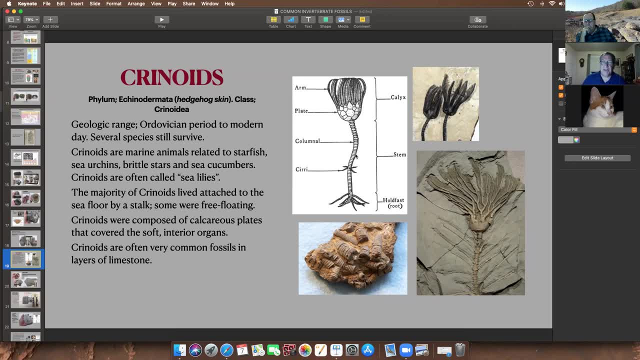 inches, uh, the body, or calyx, the, the stem, and then the holdfast, the roots- uh, there were. there are a layer of echinoderms that are in the phylum echinodermata, and then there are a layer of limestone where you can find nothing but thousands of crinoids all laid out, and it's kind of like a 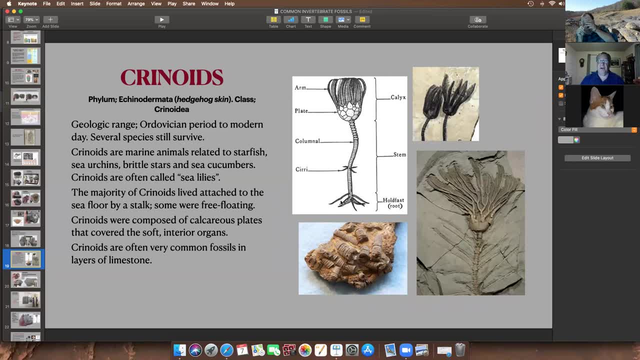 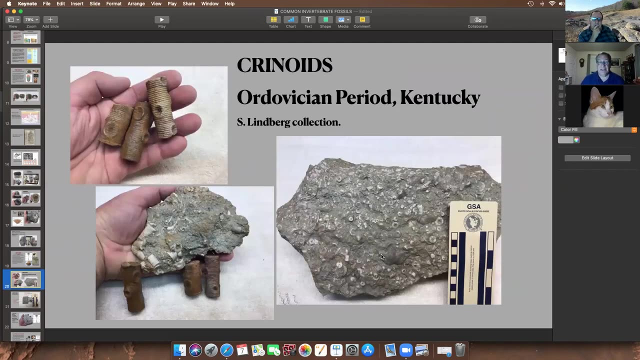 death plate, where they must have been covered by some underwater turbidity current. uh. they make spectacular fossils, since they consisted of calcium carbonate uh plates. they are usually extremely well preserved. uh. these are pieces from the ordovician period in kentucky: a piece of limestone with disarticulated 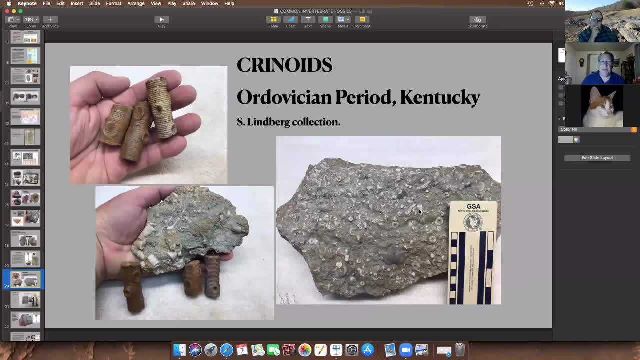 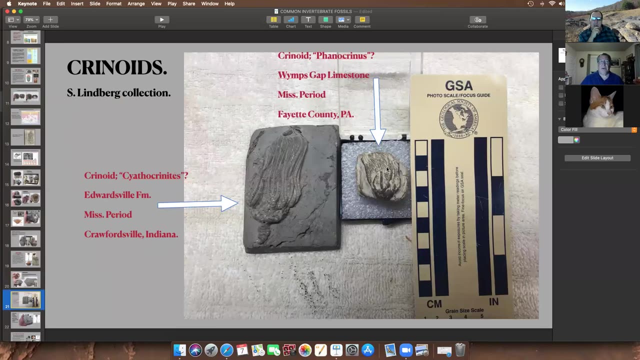 columns and plates from crinoids that have been beautifully preserved. uh, some much, much larger crinoid column sections. they resemble like stacks of little cheerios. there are also some brachiopods in here. um, two of the better crinoids that i have in my collection. um, this is from the edwardsville. 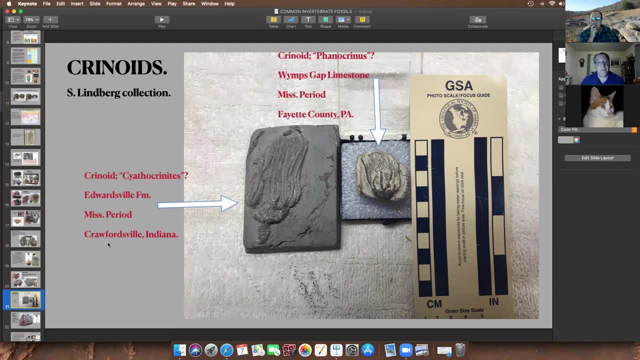 formation which is mississippian period, from a very, very famous location, crawfordsville, indiana. we have the stem and the calyx of the crinoid, along with all the beautifully preserved arms and these little pineals, and then this- um, if anyone's taking part in the field conference of pennsylvania geologists. 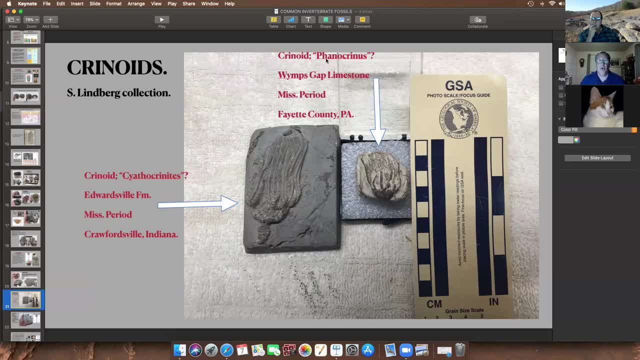 uh, the weekend of october 7th, 8th and 9th. uh, the quarry that i found, this one and we will be going to this is from the jv thompson quarry in fayette county, uh, pennsylvania. uh, this is from the. 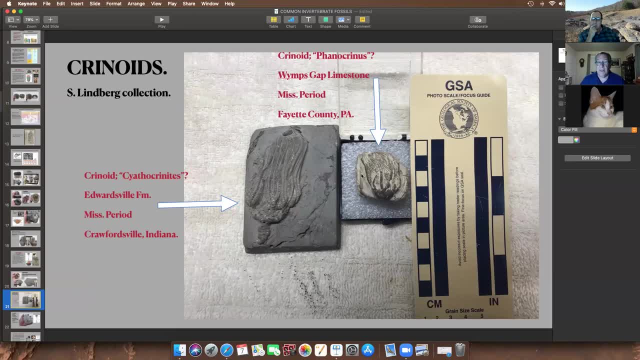 mississippian period, whipscap, limestone. uh, a tiny little, about an inch inch and a half crinoid. i did a little bit of prep work on this to remove some of the matrix around it, but a beautifully preserved calyx and arms and these little tiny pinnials. so here's the hold fast. 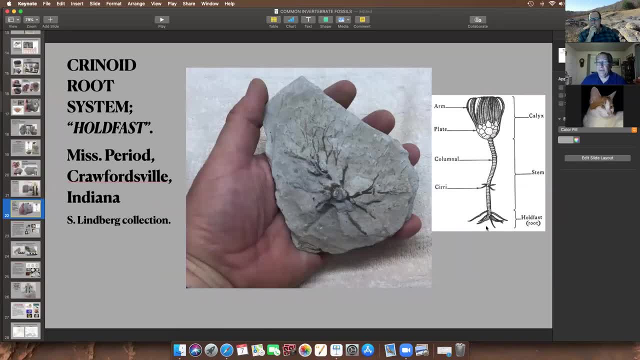 the majority of crinoids stayed anchored to the sea floor by what looked like roots but were actually, uh, part of the living stem, so these roots would have had a soft, fleshy interior. so actually, looking down the length of the column, so that's the crinoid, that's the main column, that's the. 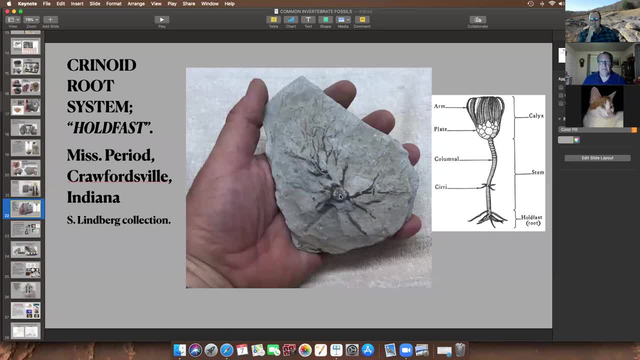 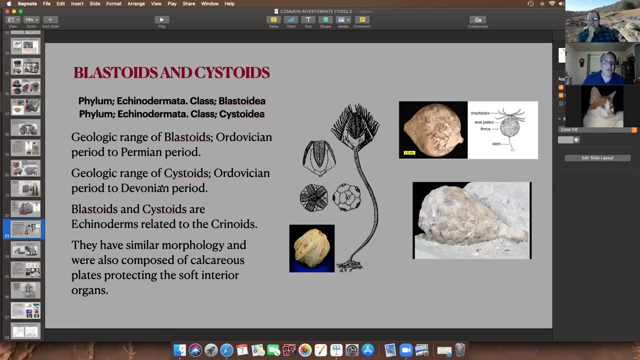 this would have been. you're looking down at the seafloor and the column- the stem of the crinoid being snapped off here. That's how I found that sample, So I never found the rest of the crinoid that was attached to it. In the same phylum as crinoids are blastoids and cystoids. A cystoid. 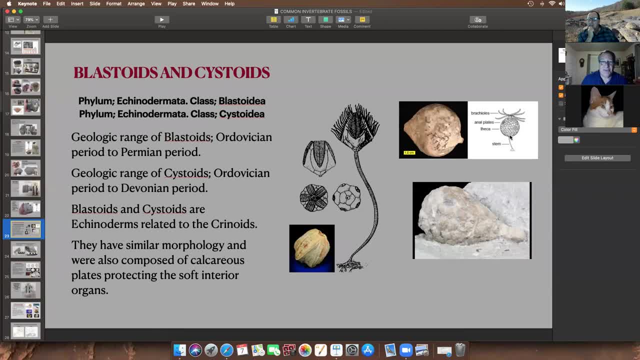 name because it kind of looks like a biological cyst and a blastoid because it resembles some blastoids resemble like the blastoid stage of a fertilized egg. Blastoids are also present in a lot of Mississippian Pennsylvania period rocks. 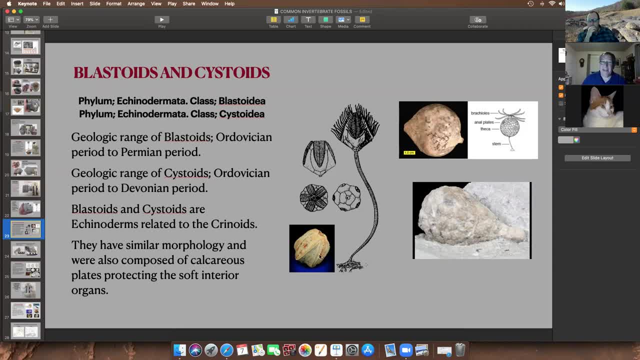 Ordovician to Permian period. same thing. calcareous plates. These are echinoderms. They were basically filter feeders in the ocean, with the little openings and resembling a sand dollar or a serotonin. But picture it attached to the ocean floor with the stem. 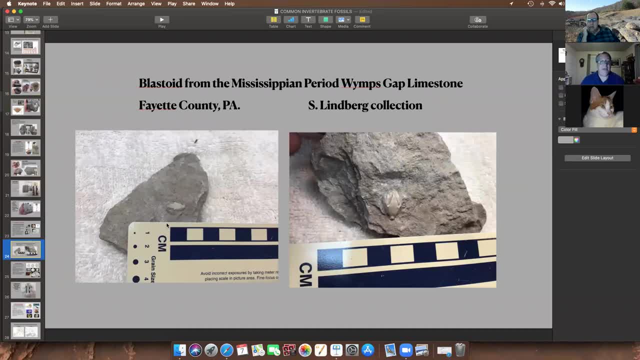 Here is a. here's a blastoid that I found from the same Whimscap limestone quarry in Fayette County, Pennsylvania. a relatively small one. It's been cleaned a little bit, did a little bit of prep work on that. The stem would have been attached to the bottom here. This is the calyx. 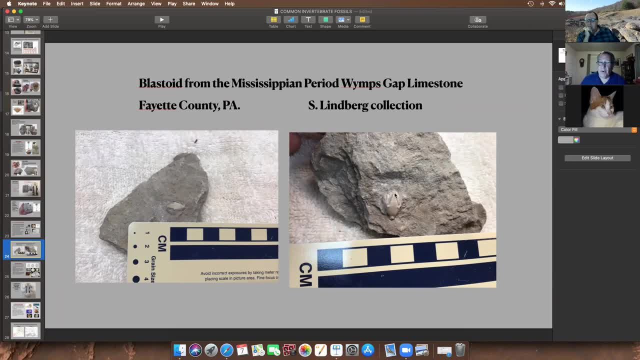 and these little grooves would have been open And this is where the seawater would have filtered through, And we call these the ambulacrum. These are the macral grooves, Cystoid, a little different morphology than a crinoid. Then we 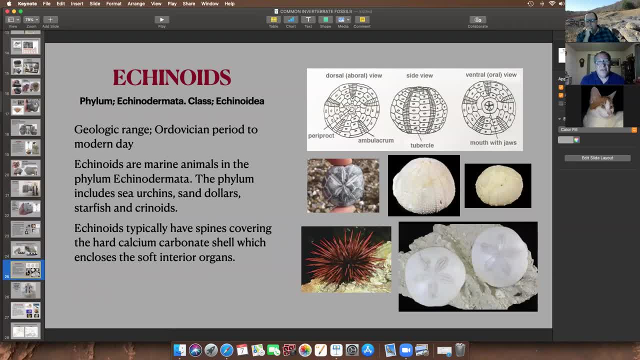 have the echinoids- Still same phylum, but the class echinoida. Echinoids are the sea urchins, the sand dollars, Very, very common fossils, especially in cenozoic sediments. if you get down to the Gulf Coast, You can also typically find these along the Georgia and. 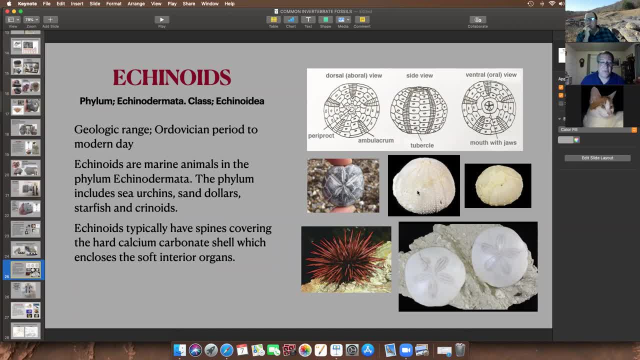 North and South Carolina coast Living ones. these are the Echinoids. And these are the Echinoids. These are the Echinoids, But also fossilized ones that come out of the sediment. Here are a few Echinoids. These are: 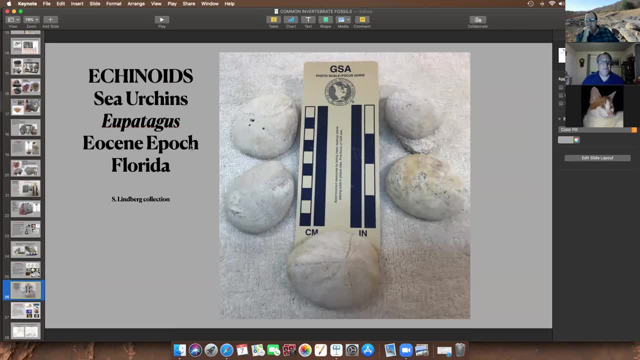 from the Eocene, relatively recent cenozoic era, Eupatagus, very, very common fossils. These can be collected in many, many places down in Florida and the southern states And they're often very, very beautifully preserved Cephalopods, I think. 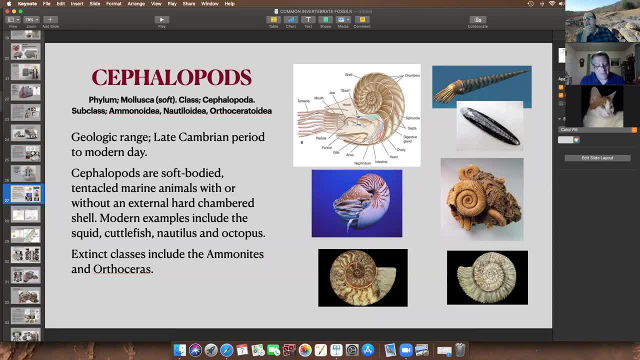 after trilobites or I don't know. I'm kind of torn between what are my favorites: trilobites or the cephalopods, the ammonites- It might be a tie, But cephalopods make absolutely spectacular. 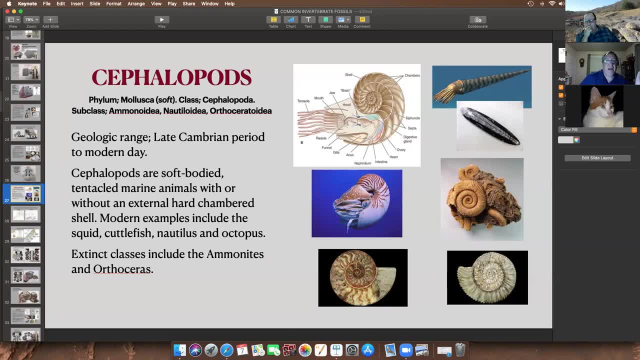 fossils And the phylum or the group of cephalopods. the phylum mollusca encompasses hundreds and hundreds of different animals, Mollusca meaning soft- I believe that comes from the French meaning soft. So the mollusca, the cephalopods, are soft-bodied animals. So the 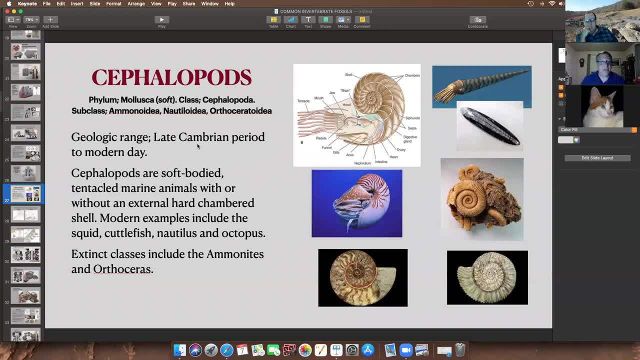 geologic range is Lake Cambrian. to modern day, The modern chambered nautilus of the Pacific Ocean is a living example, almost a living fossil, of what nautiloids looked like 200, 300 million years ago. The cephalopods, the nautiloids and ammonites were soft-bodied. 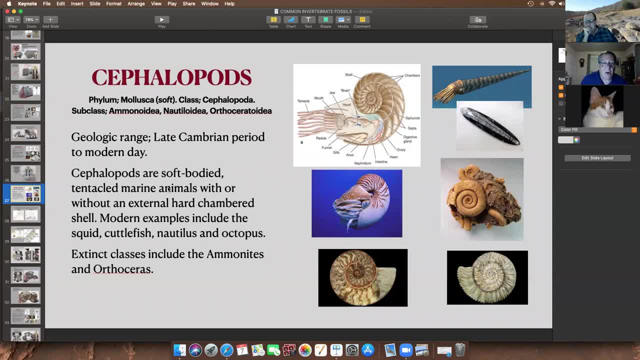 They were the main animals that may or may not have a hard external chambered shell. Modern examples of the cephalopods are the squid, the cuttlefish, the nautilus and the octopus. Extinct classes- extinct groups of the cephalopods include the ammonites and the orthoceras. 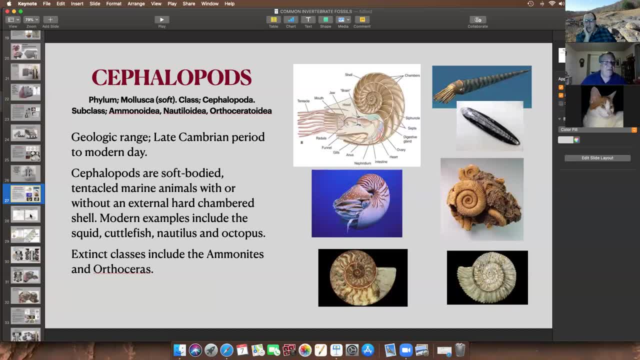 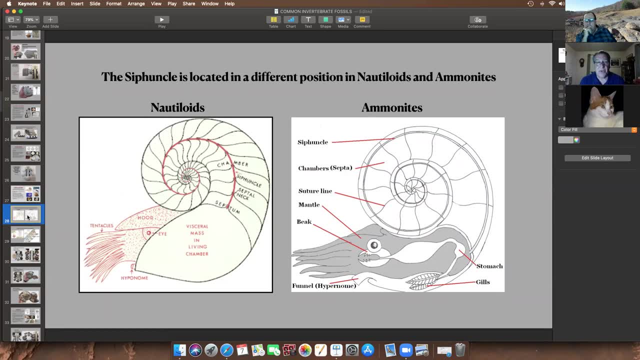 the straight-shelled orthocones. Oftentimes these fossils grew to enormous sizes. I mean, I've seen fossils of the cephalopods. I've seen fossils of the cephalopods. I've seen fossils of ammonites and cephalopods from the Mesozoic era that are three, four, five feet in diameter. 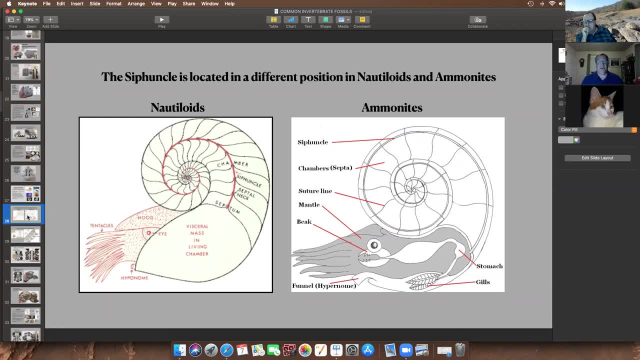 They evolved very rapidly during the late Paleozoic and into the Mesozoic era. One of the main differences between a nautiloid- if you have a nautiloid shell- and an ammonite is the internal anatomy. A nautiloid has a tube that connects the different growing chambers. 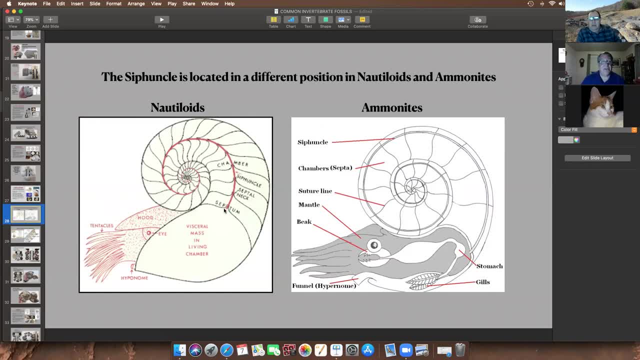 called a siphoncle, And in a nautiloid, the siphuncle runs through the center of the shell and follows the spiral of the shell. This is basically a gas-regulating tube, and that's how the animal would regulate his buoyancy. 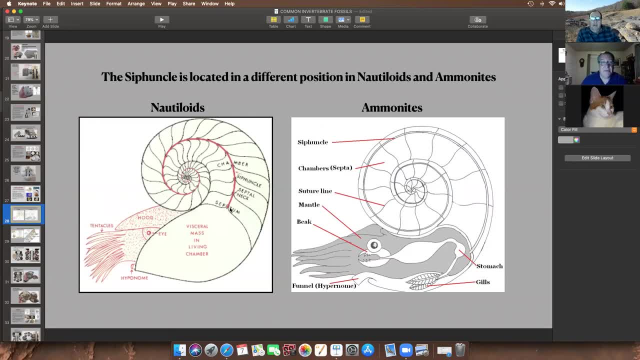 So in a nautiloid the siphuncle which is sometimes preserved in a fossil siphuncle, runs through the middle of the shell, But in an ammonite the siphuncle runs along the outer edge of the shell. 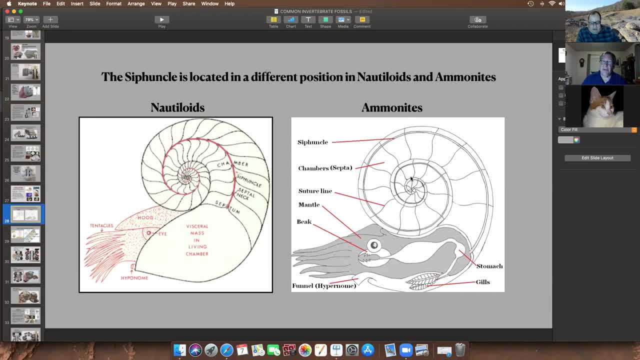 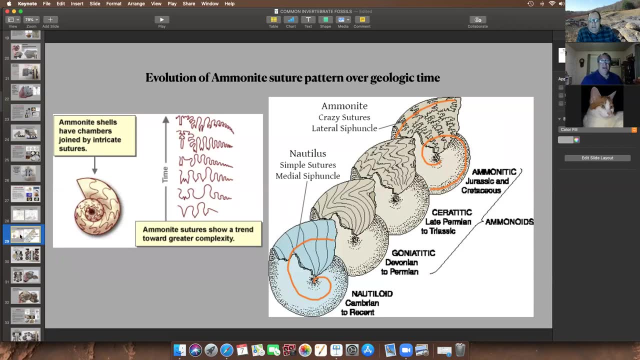 So if you can't tell from the outside, you can always slice the shell in half and look and see where the siphuncle is. Ammonites and nautiloids have what's known as a suture pattern Inside the shell. the animal lives within the opening- the front chamber. 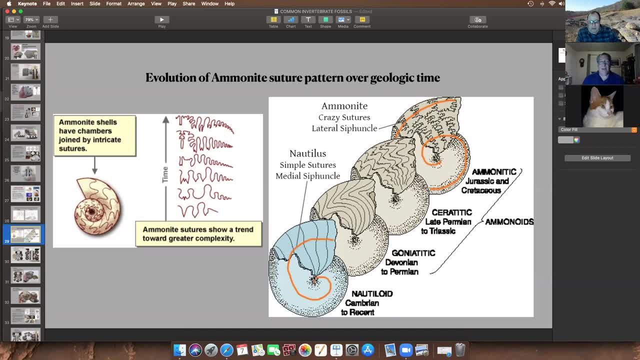 But the siphuncle runs through all the previous growing chambers And as the animal grows he seals off the chamber behind him And Over geologic time we call this the septa, the septa or the septum, the. 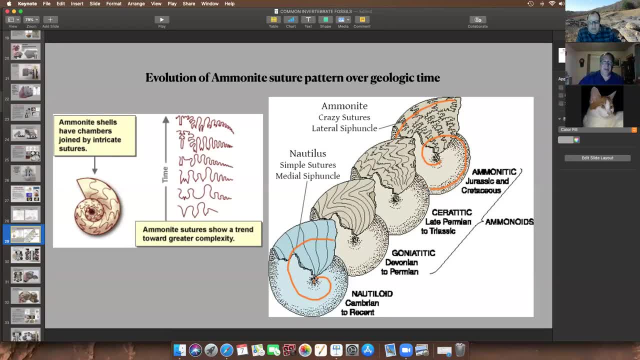 The plate. the plate that seals off the growing chamber becomes more and more complex over time. So in a nautiloid, the septa, or on the outside of the shell, we refer to this as the suture line. The suture pattern is very simple. 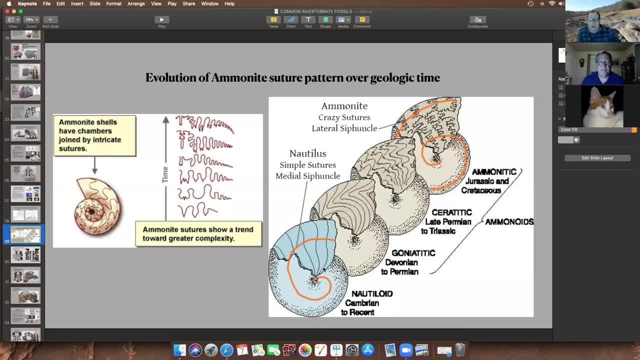 And there's actually a technical term for this that I didn't Include. but the suture line that shows the internal ceiling of each chamber is very, very simple, which is some basic waves And then, as we go through geologic time, especially well, the ammonites. ammonites started out with what we call a goniatite suture pattern and then a ceratite suture pattern. 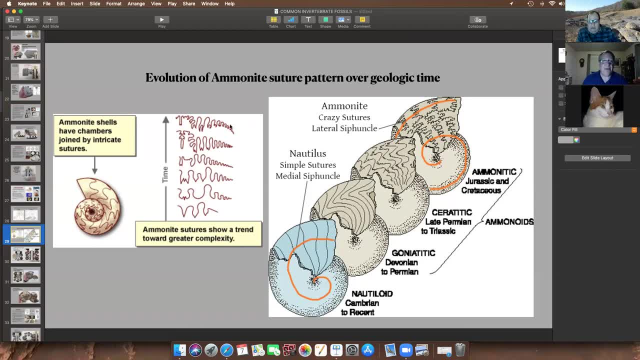 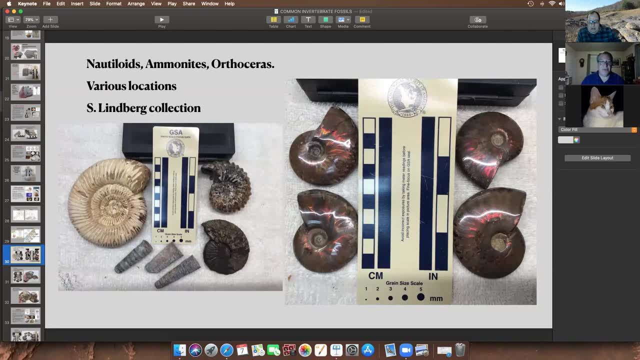 And then finally, the classic ammionite suture pattern. So we get this very, very involved suture pattern that, when you polish the shell, can be absolutely Beautiful. So here's just a couple of examples. These are: this is an ammonite from Madagascar. 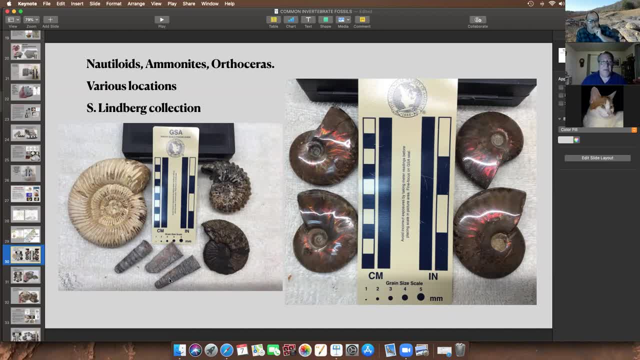 These are straight shelled orthoceros from Morocco. This one is from Russia. This is a Russian ammonite for the Mesozoic. I believe this one is also Moroccan, And these are iridescent ammonites- The aragonite that was preserved on the outside of the shell. 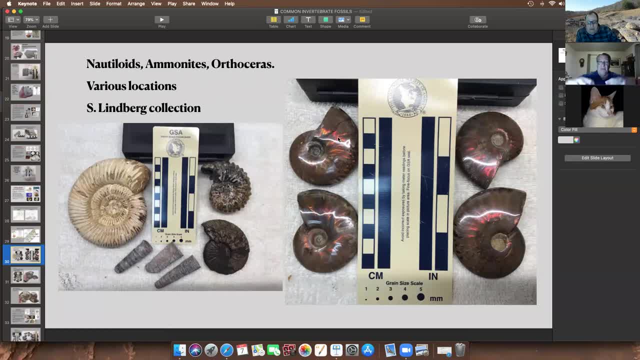 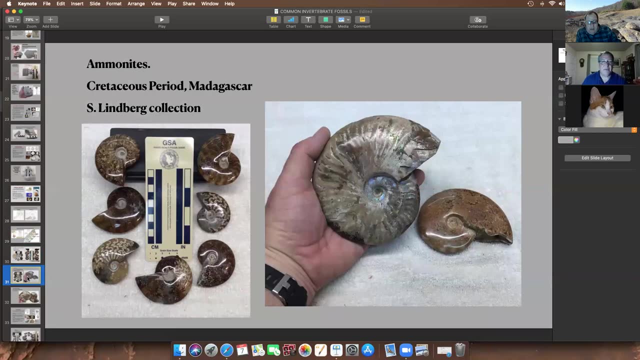 Will diffract and refract the light that's being reflected off the internal layers, And this happens within the first few thousandths of an inch of the outside of the shell. So we often find these beautiful iridescent ammonites where that part of the aragonite on the shell has been preserved. 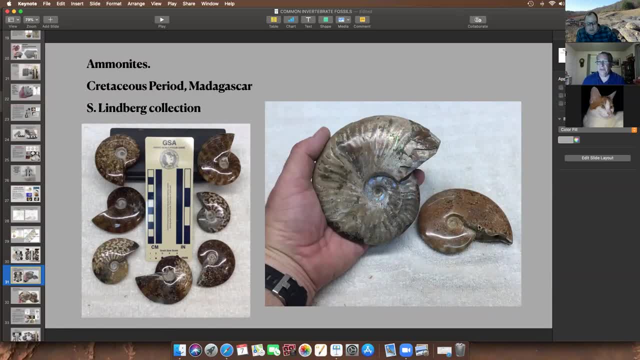 Here are some other ammonites. This is: these are from Madagascar. These are Madagascar ammonites And the reason I showed these is you can see the outside of these shells have been Polished and you can see this beautiful, wavy, intricate suture line that zigzags across the outside of the shell. 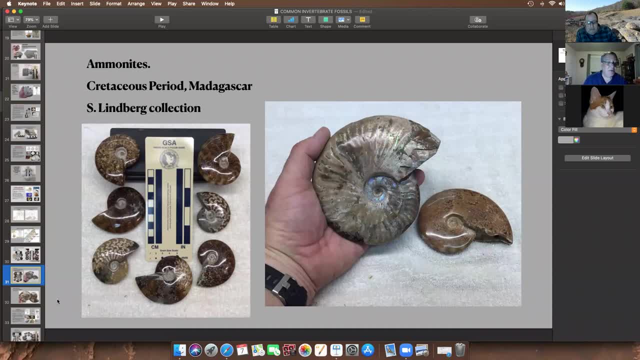 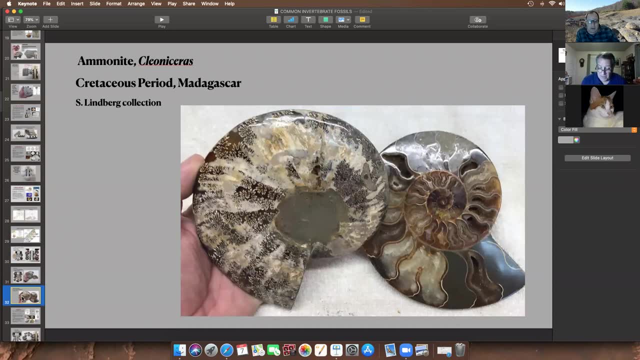 And that's how you can tell that these are ammonites and not a nautiloid. Here's a classic. These are being exported from Madagascar at a very high rate. I'm not quite sure how much longer the supply will last, but they make beautiful display pieces. 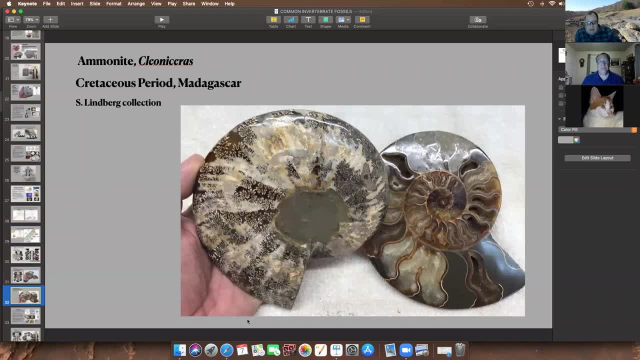 This is Cleonoceros, a Cretaceous Period ammonite from Madagascar, and the outside of the shell has been polished and you can see that beautiful, intricate, involved suture pattern and that represents this right here, that septa. it represents that point right there where the internal septa touches the outside of the shell. the zigzags back and forth, very involved. 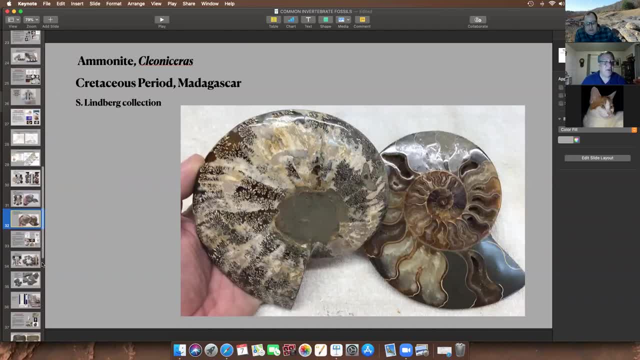 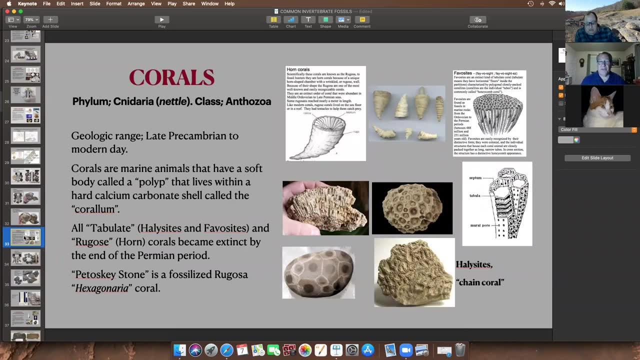 And we're able to see that And we're able to trace that across the evolutionary period of ammonites. So corals, We'll move on to corals- Very, very common fossils because they have a hard calcium carbonate shell. Corals belong to the phylum Cnidaria. 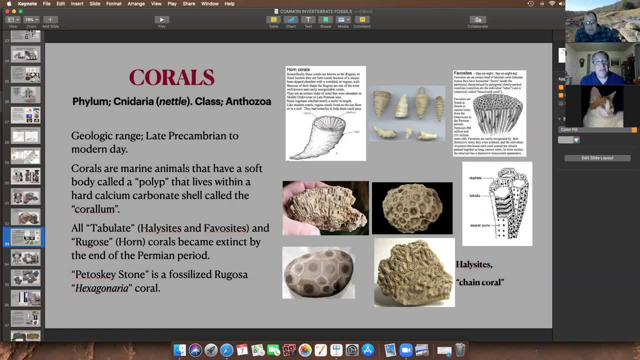 That's a relatively new change. It's a new phylum name. Cnidaria means nettle or stingers, because most corals have little tentacles on them and stinging cells. Corals are present from the late pre-Cambrian to modern day. 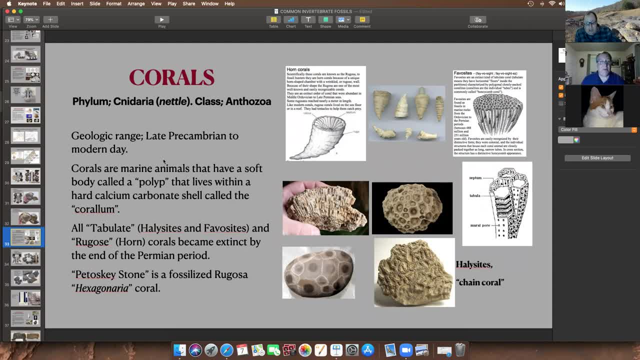 The animal. it's a soft-bodied animal that lives in a shell called a corellum. The body of the animal is called a polyp. I don't show really any examples of living corals here. There are hundreds and hundreds of different species of modern living corals. 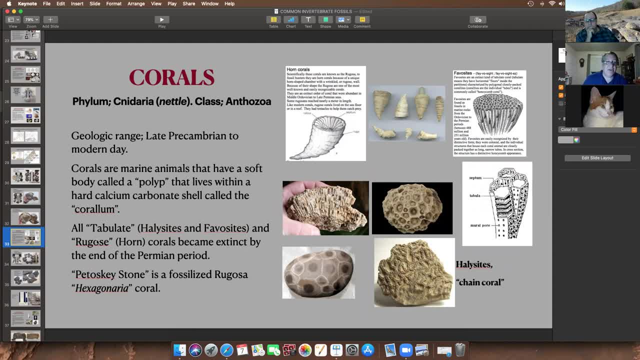 The two most common fossilized ones that are now extinct are the tabulate corals that we call Halicites and Favicites, And also the rugos, the horn corals of the Paleozoic era. If you go to the New Paris Quarry on October 24th, you'll be able to find some pretty neat Halicites and Favicites corals there. 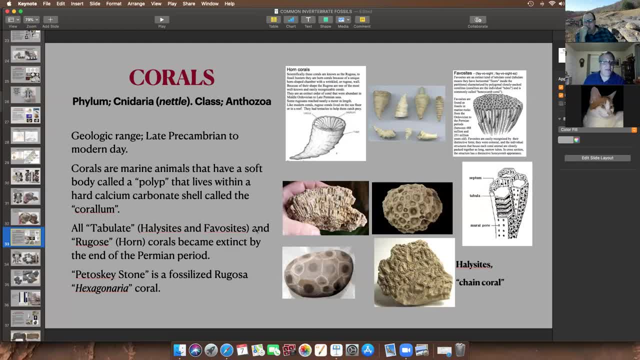 And you might even have a chance of finding some horn corals. The popular Petoskey stone- from Michigan, I believe there's even a town called Petoskey- is a fossilized Ragusa. It's a hexachoral that's now extinct. 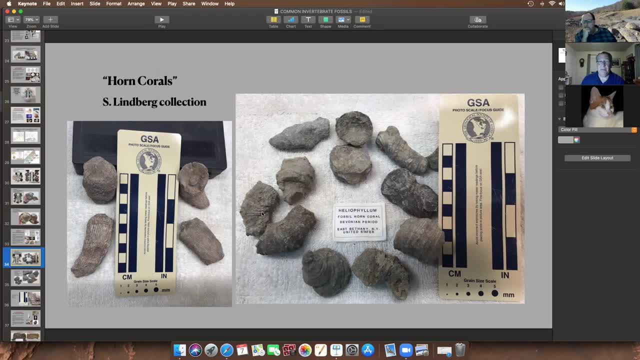 Fossil corals, or at least corals from the Paleozoic and Mesozoic and Cenozoic era, make really really well-preserved fossils because they had a hard calcium carbonate shell. These are horn corals. This is Heliophyllum from the Devonian period of New York. 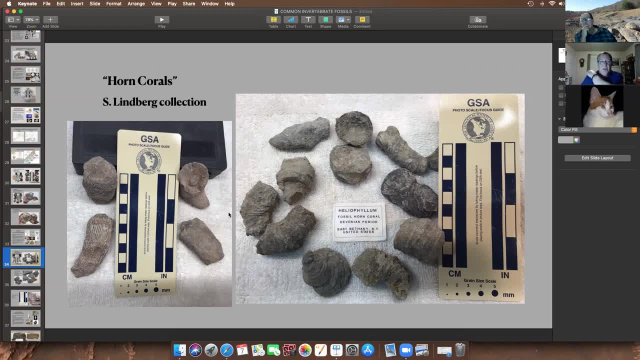 There are places I've been to in upstate New York where you can literally pick these up off the ground. They weather out of the surrounding shells And here you're kind of looking down into the shell. That's where the soft-bodied animal would have been living in that shell and anchored in by all these little septa that radiate out from the center of the shell. 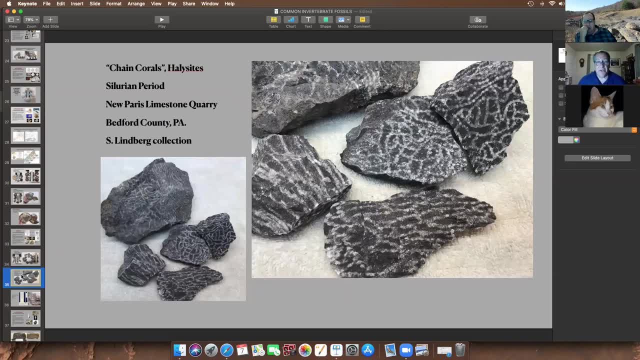 This is from the New Paris Quarry that we'll be going to. This is a Halicites chain coral that was broken out of a large block of limestone. This is actually a fairly large piece. I didn't put a, I didn't put a reference in here for scale. 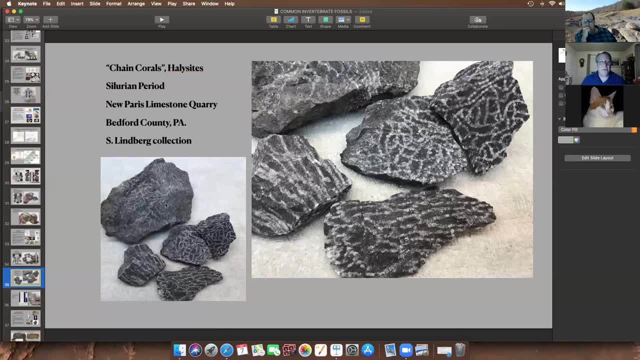 But this piece right here is about the size of- Oh, it's about the size of my hand And you can see the intricate. These are the chain corals. There was a little animal, a little polyp, that lived in each one of those chambers. 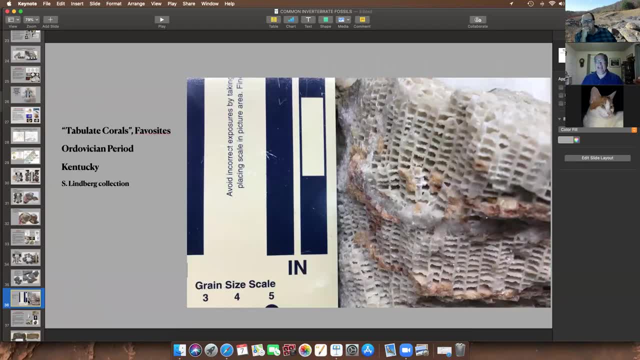 And these are now extinct. today Here's a tabulate coral. close up. You're looking kind of like at a cross section. The living surface of the coral would have been up here, And these are previous polyp chambers. So as the corals die, a new one grows on top. they seal the chamber off below them. 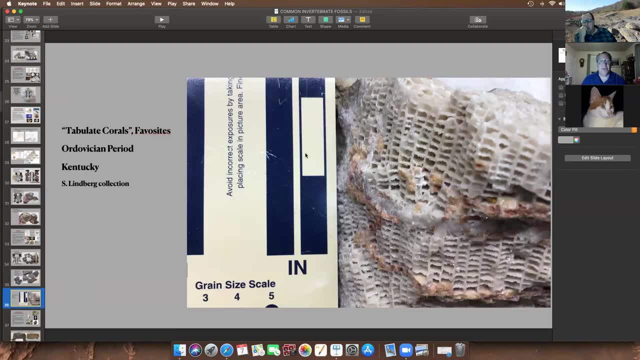 And you can see, this is why we call these the tabulate corals. This scale is in inches, So we're probably looking at- We're looking at little chambers here that are about a millimeter in width, And this is from the Ordovician period of Kentucky. 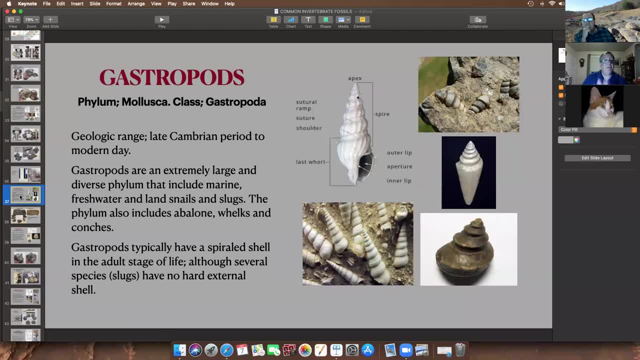 Gastropods. We're still in Nope. now we're in the phylum mollusca, All right. Well, back in mollusca. the same thing as the cephalopods, But the gastropods are what we typically think of as snail shells. 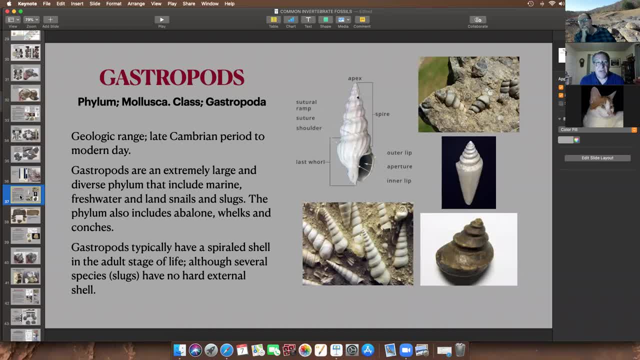 Very common fossils, the Lake Cambrian. to modern day, The gastropods are an incredibly large and diverse group of animals. It includes welts, conches, snails, abalone. There are some modern species like the slug, That's a gastropod that has no shell. 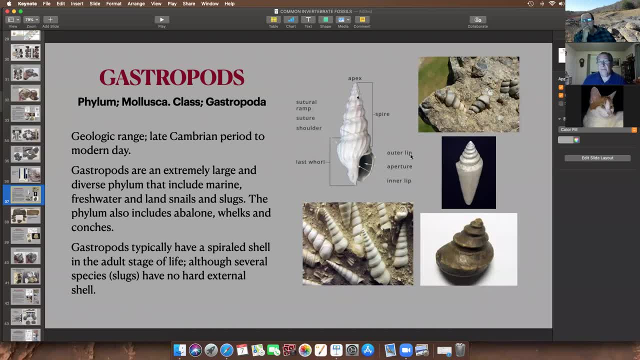 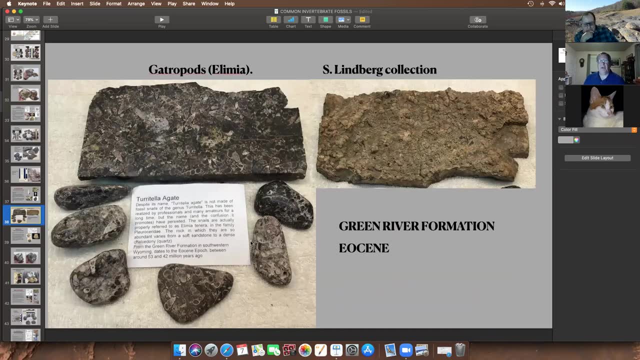 Very, very common invertebrate fossils. The main reason is because they have a hard shell, The teratella agate of common name, that's found out in the Green River Formation, the Eocena viomi. Here's a slab that I have in my collection: a rough piece, and then cotton polished and then some tumble pieces of teratella. 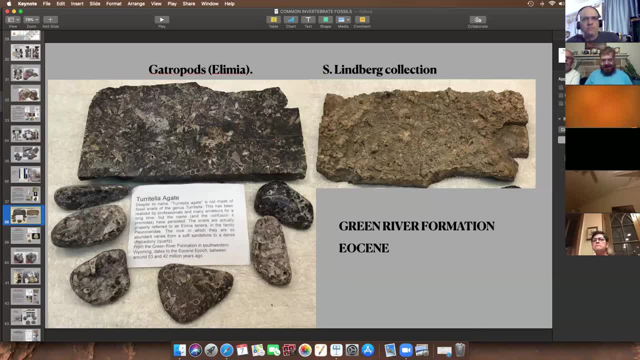 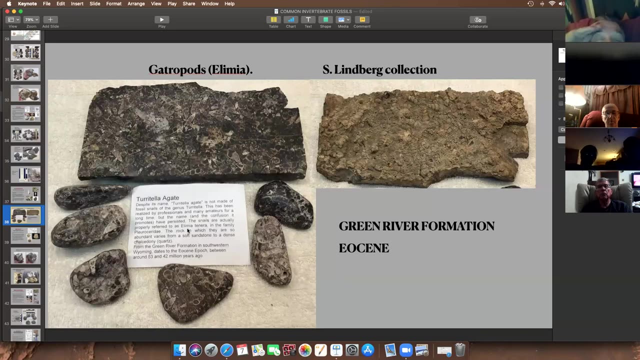 These are preserved. These are preserved gastropod shells. But the interesting thing about teratella agate is these are not teratella and this is not agate, So the tag here describes that it's actually. it's actually a gastropod known as Alemia tenera and the rock. the rock is actually a dense chalcedony. 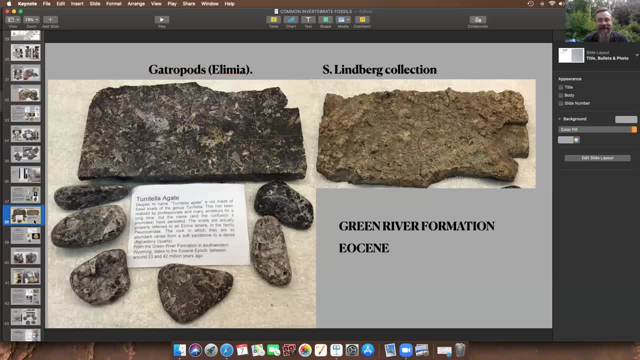 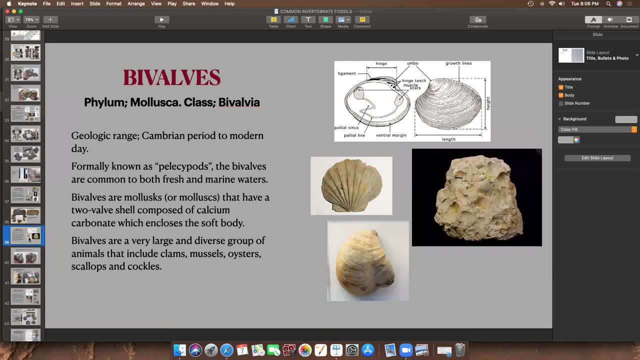 In order to be an agate, it would have to be banded, and it's not. So it's misnamed, but it's an excellent example. Okay, It's one of the more recent gastropod. Okay, Then, under phylum mollusca, we have the bivalves. 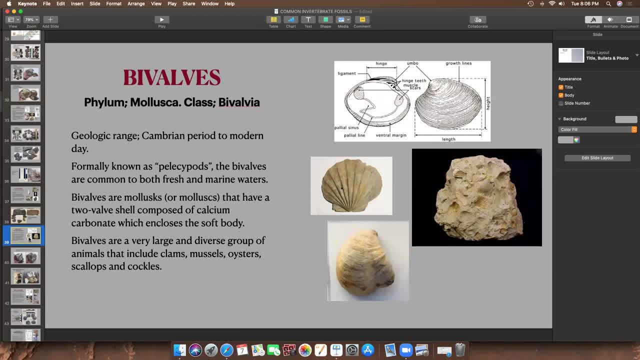 Bivalves are the clams, the oysters, clams, oysters, mussels, cockles, scallops. If you have ever been down to Calvert cliffs, Maryland State Park, that's the, that's the bivalve. 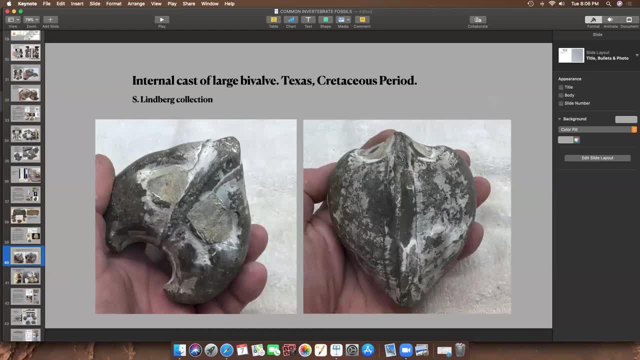 Bivalvia mollusca collecting haven. Here's a large. it's been in my collection for a while. I can't even remember remember where I acquired it, but this is an internal cast. This is where the muscles would have been attached to the shells. These are sometimes called the heart fossils or heart. 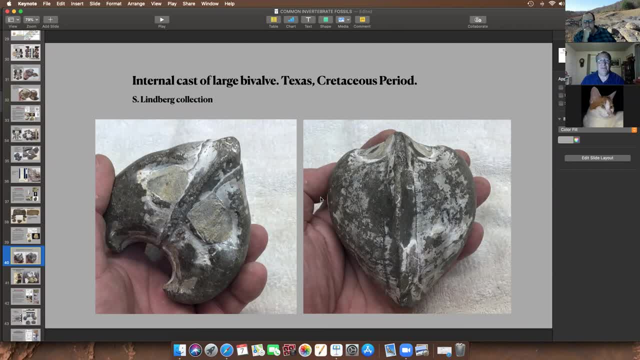 clams. They kind of resemble the size of a large mammal heart. but this is the internal cast of a large bivalve and this is from the Cretaceous period in Texas. You can see some of the original calcium carbonate shell material is still on there and the scars were the internal muscles. 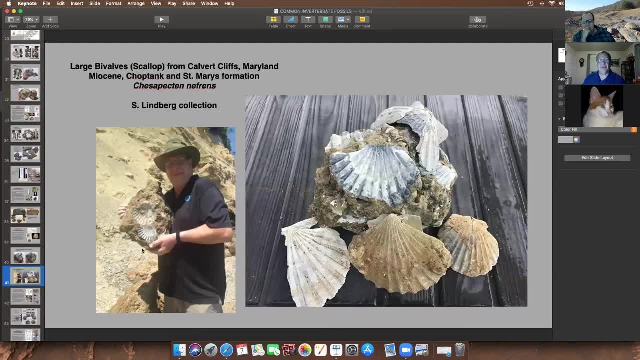 that held the shell together can still be seen. Here's Calvert-Cliffs. This was a couple of years ago. I was kind of thrilled to be able to collect that large piece. These are large bivalve scallops from Calvert-Cliffs, Maryland. This is myosin. These are from the chop tank. 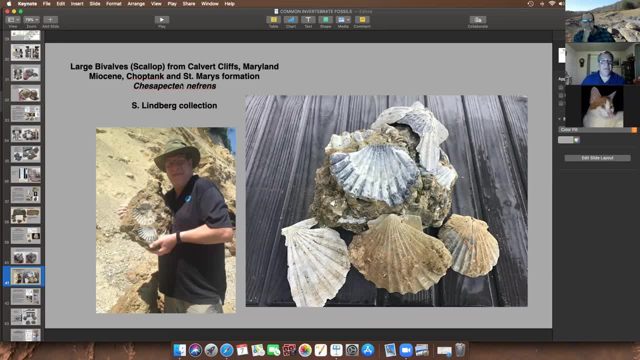 I know Jerry has talked about Calvert-Cliffs in the past. This is from the chop tank in St Mary's Formation: Chesapectins, nephrons, and there are places down here. All of these loose blocks were packed with absolute tens of thousands of these. I had to go away. 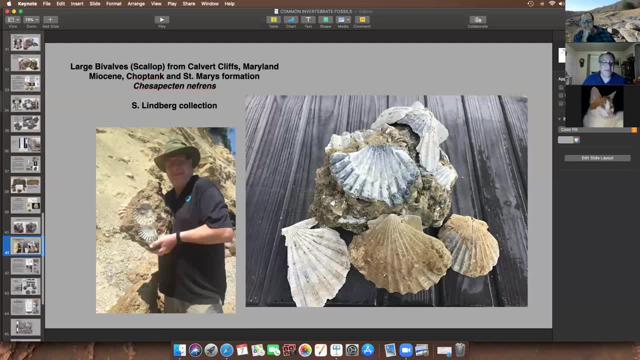 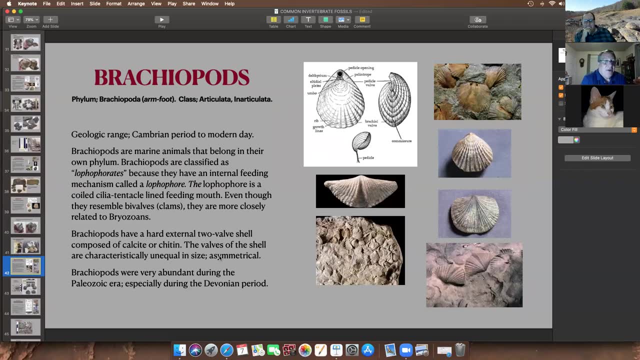 with the large scallops. I wasn't successful in finding any shark teeth that day. Okay, The brachiopods. I'm going to try to speed up here a little bit. I don't want to go on too long, but the brachiopods mistaken for clams and bivalves, but they're not, So they look very much like 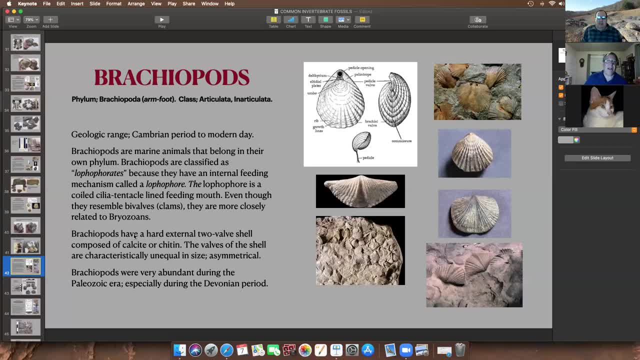 bivalves and clamshells, but brachiopods. the word brachiopod or brachiopoda means arm foot, in reference to the pedicle, this tough little muscular stalk that would anchor the shell to the bottom So he could- mainly a lot of brachiopods would- float back and forth in the 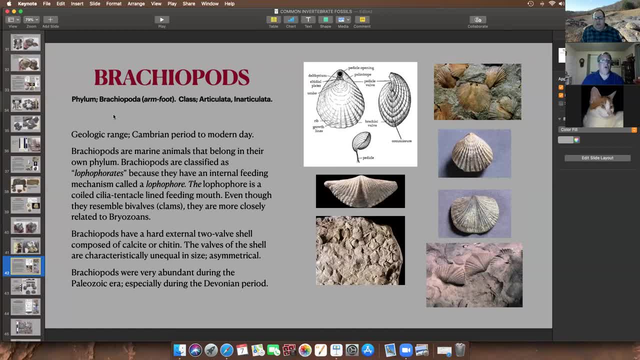 current because they were filter feeders. But brachiopods are in their own phylum. They are not mollusks. They are in their own phylum. brachiopoda- They're from Canberra, modern day, They are. what makes them different than bivalves clams and mussels is brachiopods. 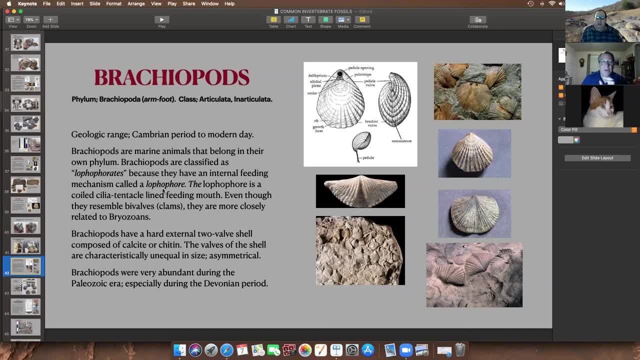 are. they have a lofophore. A lofophore is a horseshoe shaped feeding organism that's lined with cilia And the organism will open and the cilia will make the water flow into the organism to filter feed. 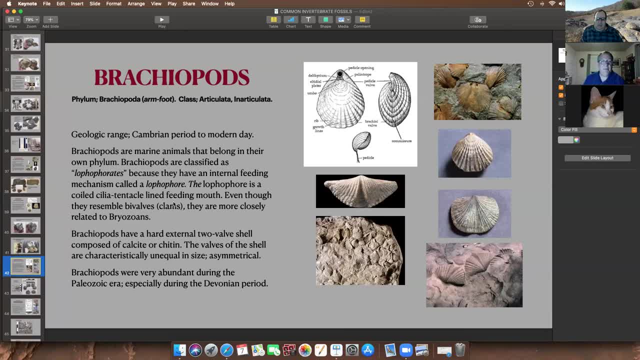 They're more closely related to bryozoans than they are clams. But brachiopods make spectacular fossils. Some of them are quite large. They're extremely ornate. especially the spirophors and the atropas They have these ornate shells. They were bivalves but 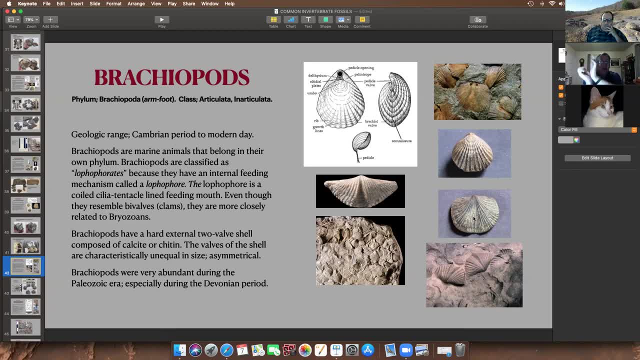 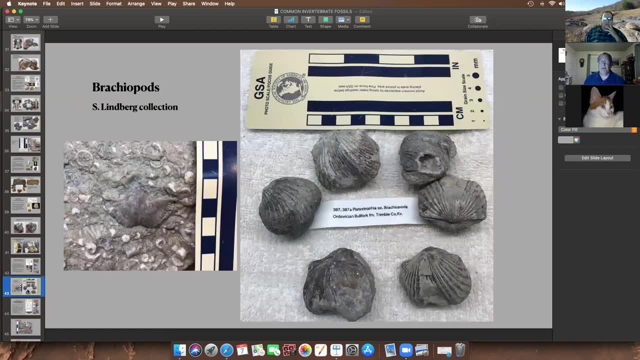 one valve was always larger than the other, So they have unequal, they're asymmetrical in their valves. In some places brachiopods can be picked up by the thousands. These are from. these are from Trimble County, Kentucky. They're platystrophia ordovician brachiopods. These 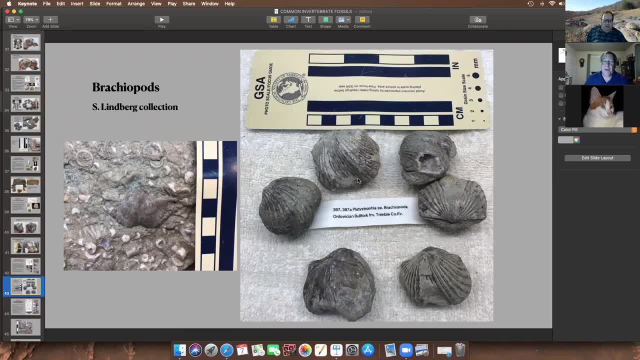 are some of the largest brachiopods I've ever seen. I was absolutely amazed when I saw the size of these brachiopods. You can see the scale of inches up here. Some of them are two inches across and they're perfectly preserved. I haven't cleaned them completely. The neat. 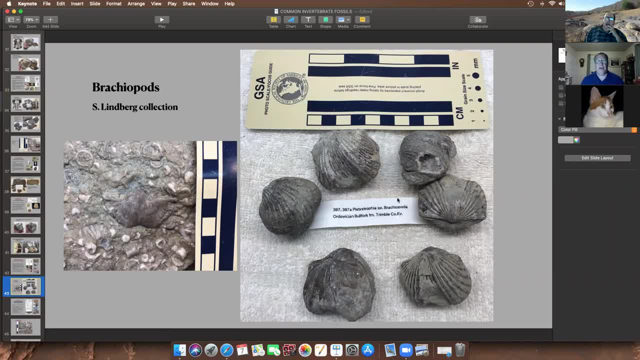 thing about these, a lot of these brachiopods. they're not as large as they used to be, They're like little geodes. Here's a spirophor brachiopod. that's on that same piece that I showed you. 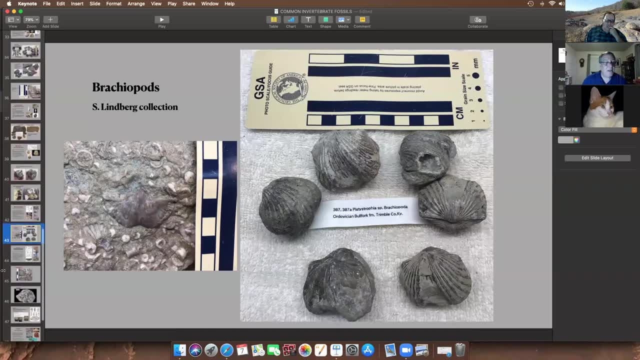 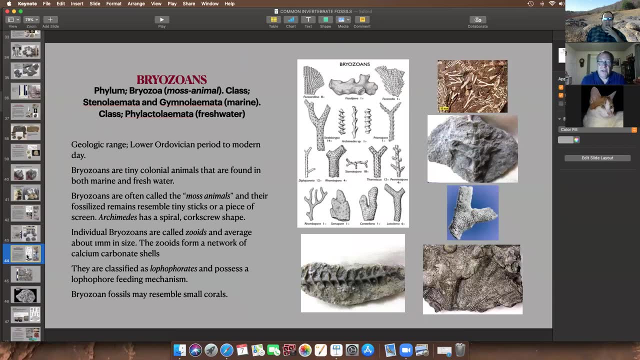 earlier, with the crinoids on it. So bryozoans- depending on the units that you're looking in. well, bryozoans can be extremely difficult to find, but in some places they're really common. There are lots of bryozoans at the New Paris Limestone Quarry. During the Paleozoic era. 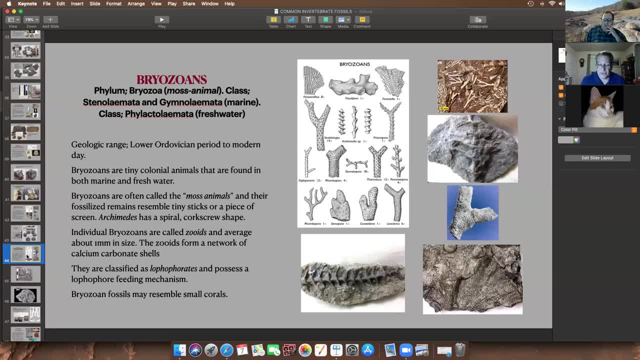 bryozoans were major reef builders. along with corals, They were the builders of reefs. The word bryozoa: they are in their own phylum, an important enough organism to be in their own phylum, So it's phylum bryozoa. Bryozoa means moss animal, because they look like little. 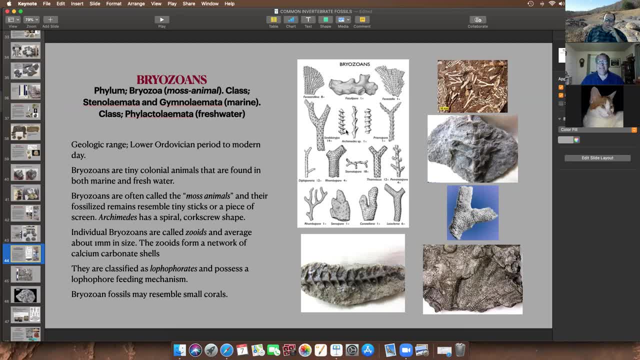 sticks of green moss. They're easily mistaken, sometimes for corals, especially the stick bryozoans with the little openings on them, And that is. those are the zooids where the little individual animals live. So bryozoans are colonial animals. There were hundreds and hundreds of different species. 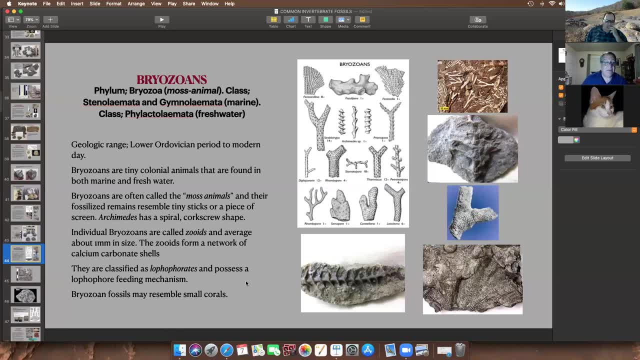 They occasionally make spectacular fossils of different types on the rock. There are lower Ordovician. to modern day, Bryozoans still inhabit both the New Paris Limestone Quarry. They have both fresh and salt water today And they have a loafer fork. The microscopic 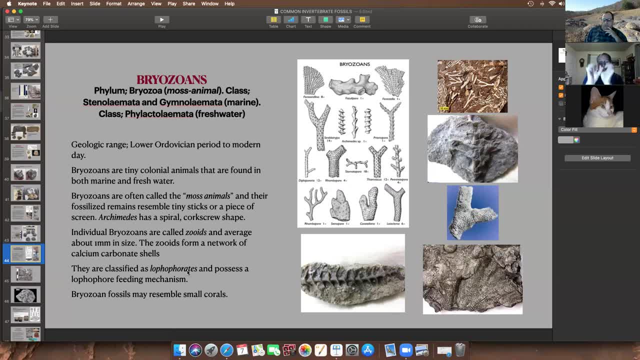 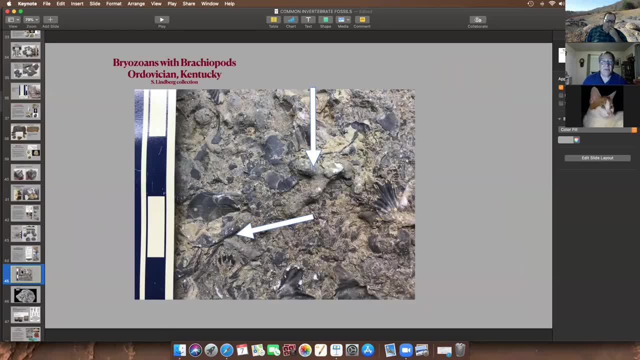 animals have a little horseshoe shaped organism with cilia that bring the seawater into the filter feeding mechanism And they may resemble. they may resemble corals. So here's a. here's a fossil- I like to call it a fossil- hash plate brachiopods, broken brachiopods And 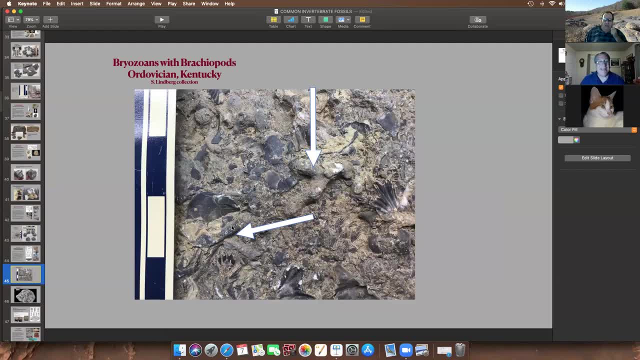 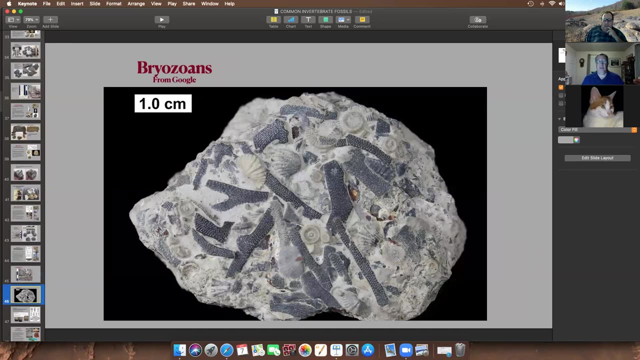 here are some, although they're really not well preserved and I haven't really etched these in These out yet with vinegar or acid, but here's. here are some large stick bryozoans And these are fairly numerous at the at the New Paris Quarry. Here's a. really this is not mine. 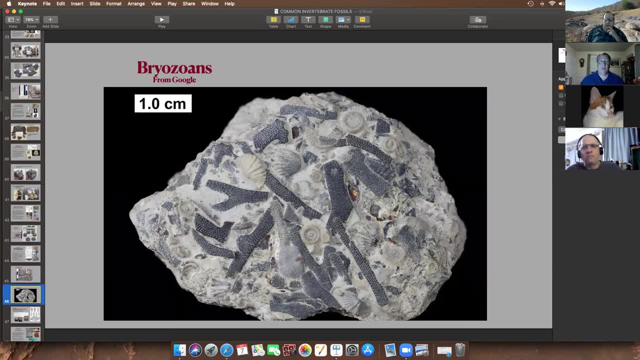 This is a snatched off Google, but this is a really really well preserved And I included it here because it's just a spectacular example of when you find really, really nicely preserved bryozoans. Now this is a- one centimeter is the length of that. 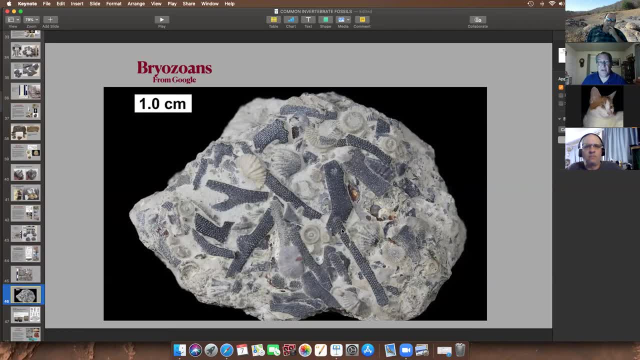 Box right there. So we're looking at bryozoans. that, oh, you know, maybe about an inch in length or less than an inch. So we have brachiopods and we have bryozoans. I usually tell people 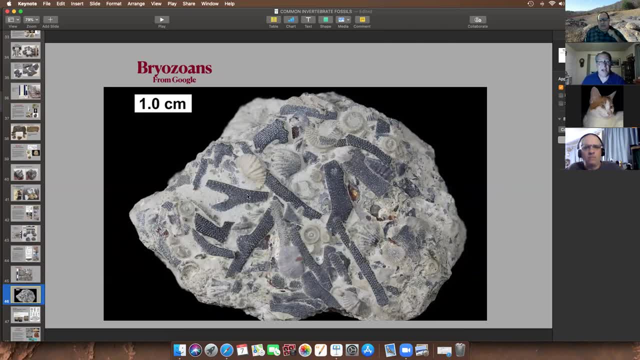 the easiest way to identify a bryozoan if you can't see it with the naked eye, look at it under hand lens and you'll see all the little openings on the preserved skeletons, on the on the colonial bryozoan Sponges. So kind of closing in on the end. here It's. 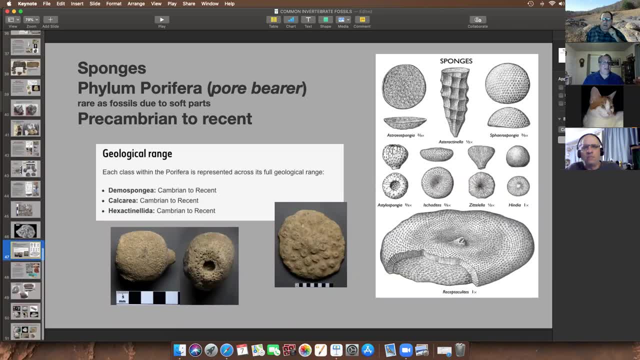 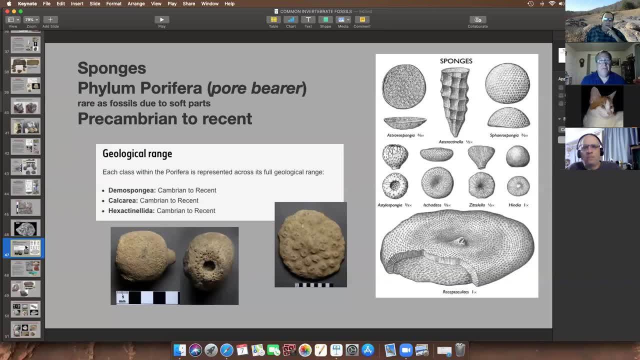 So the Porifera, phylum Porifera, and the word peripheral means poor bearer Sponges They're. they were very abundant during the Paleozoic, Mezozoic and still are today in the Cenozoic. 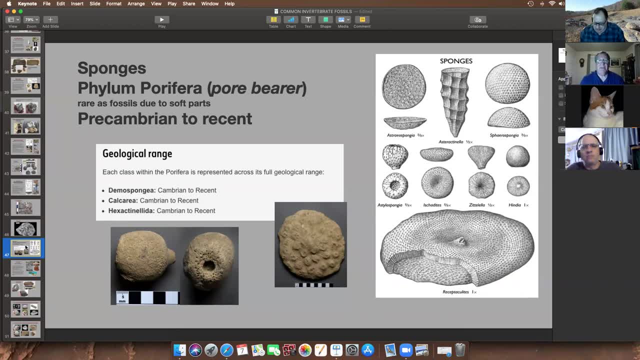 but it's kind of rare to find sponges as fossils because they mainly they're soft gelatinous organisms. there's one class of sponges that had silica spicules. You can see that here. This is a diagram. These little star-shaped, the astreospongia, had spicules of either silica. 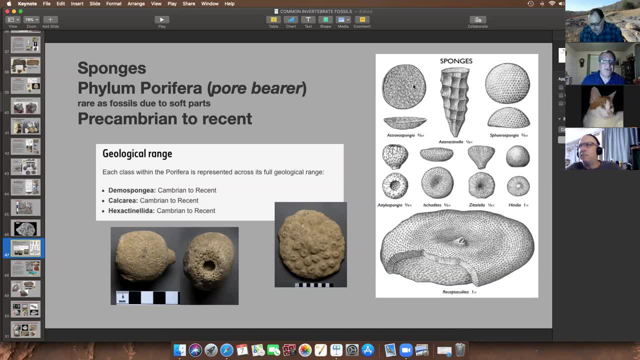 or calcium carbonate, and they preserved very well. Sometimes you just find spicules. Sponges were filter feeders. There's three main classes of sponges that are all represented as fossils. also, They range from pre-Cambrian to recent. I don't think I've ever found a fossil. 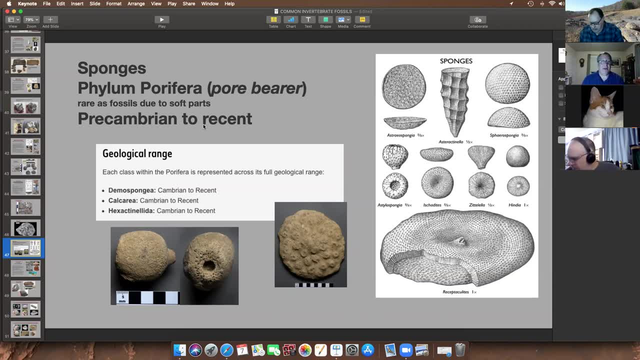 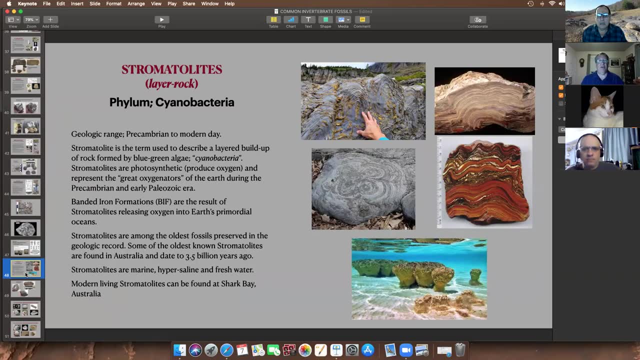 sponge. I've just never found one. I don't even think I have any in my collection. Then we move to the stromatolites. I'm including stromatolites in the invertebrate fossils because stromatolites in the pre-Cambrian period, these were the great oxygenators. 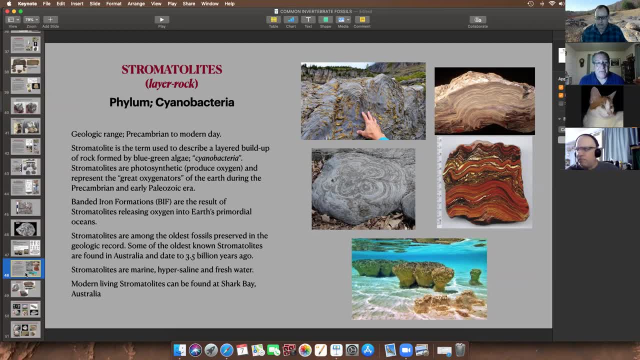 During the great oxygenation period of Earth's atmosphere. The word stromatolite means layer rock, Stroma means layer and light, from lithos. so layered rock or sheet-like rock. They're in their own phylum. It's phylum cyanobacteria, the green-blue, green-blue algae, green-blue 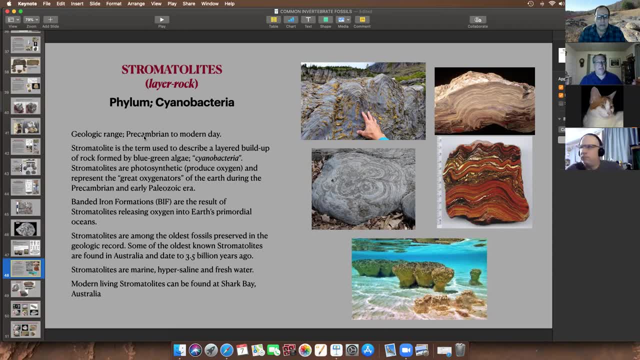 bacteria, The geologic range. there are stromatolites that still exist today. The bottom picture here. this is Shark Bay, Australia, A hypersaline, shallow, warm, salty water bay that has growing colonies of stromatolites that 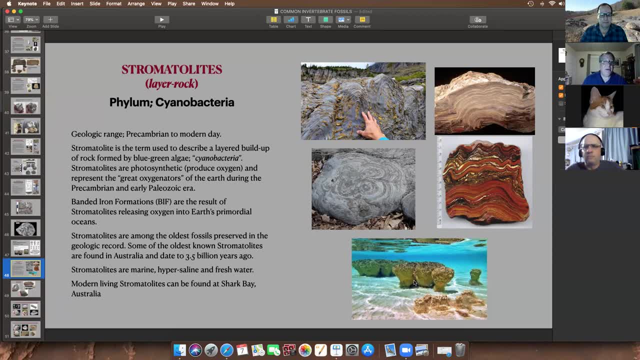 have survived over geologic time. We believe that back in the pre-Cambrian, stromatolites were the first large colonial primitive organisms to populate the Earth's ocean, and they were photosynthetic: They released oxygen into the Earth's atmosphere. 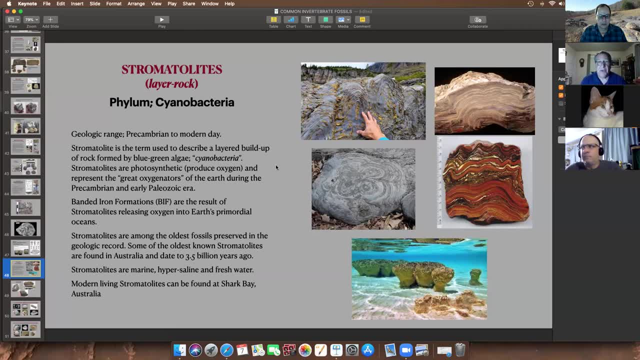 But as they released that first oxygen, it encountered all of the iron that was present in the oceans. And oxygen and iron have an affinity for each other and they bind chemically and they form Fe2O3, which is hematite, or Fe3O4,, which is magnetite, So as the stromatolites. 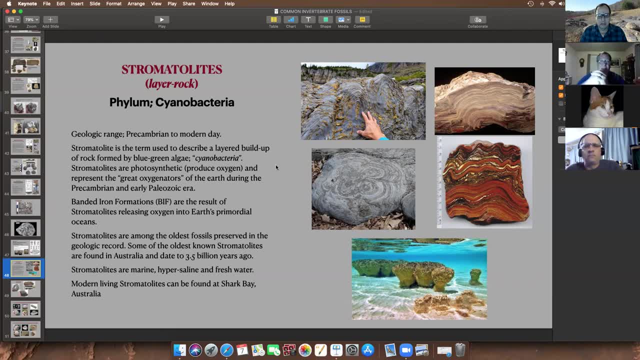 in the ancient pre-Cambrian oceans released oxygen. it combined with iron. That iron precipitated to the bottom of the ocean and it built up the famous BIFs, the banded iron, And that's why we call them the iron formations. Some of these are the actual stromatolites themselves. 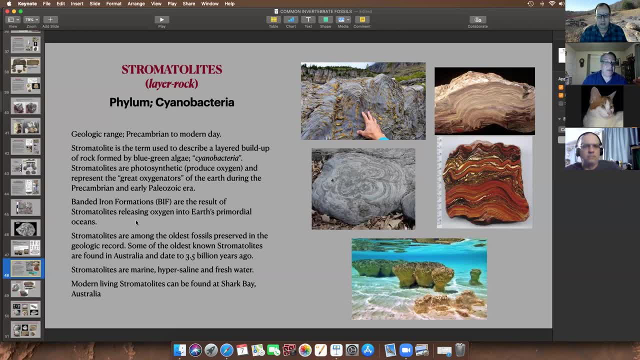 And we're lucky that this happened, because during the great oxygenation event of the Earth, after all of the iron was oxidized, then it was free to be released to the atmosphere And we had the oxygenation of the Earth's atmosphere. Stromatolites are fairly common. 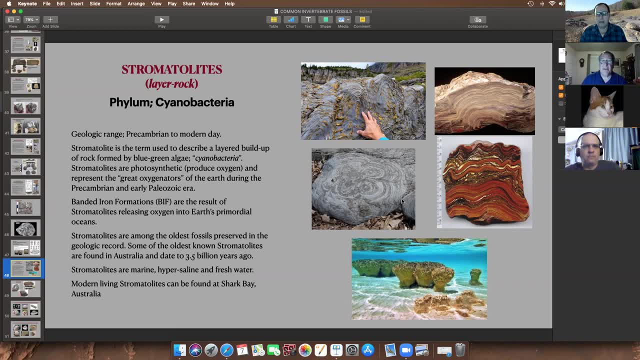 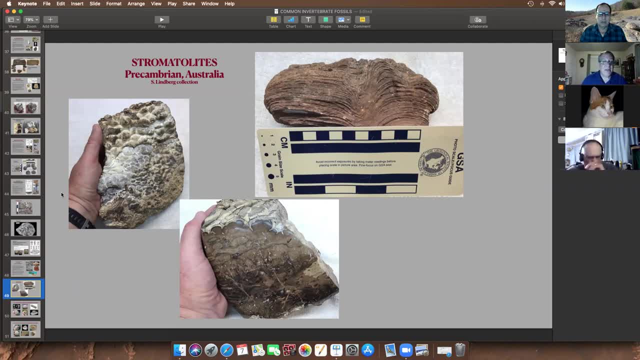 in my collection. These are all from Australia. They're all pre-Cambrian. This is a large chunk of pre-Cambrian stromatolite that I've cut and polished. You can see kind of like the textured, lumpy surface. This would have been the upper surface of a growing stromatolite. 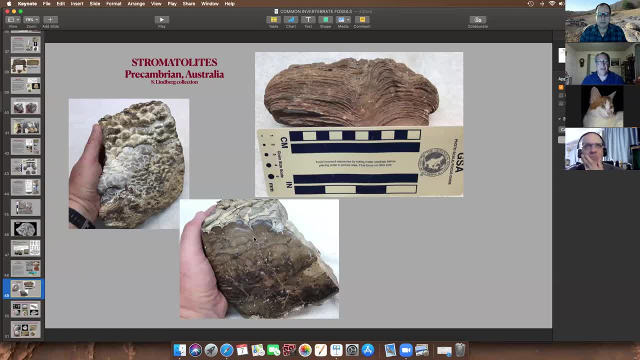 and the laminae are kind of difficult to see in here, But you can see the layered growth. And this is a stromatolite, I believe, from up in Canada, And this is a stromatolite from um. it hasn't been cut or polished. this is how it was weathered out of the rock. so with stromatolites, 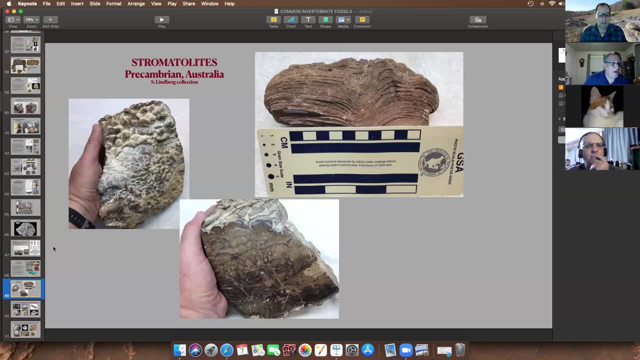 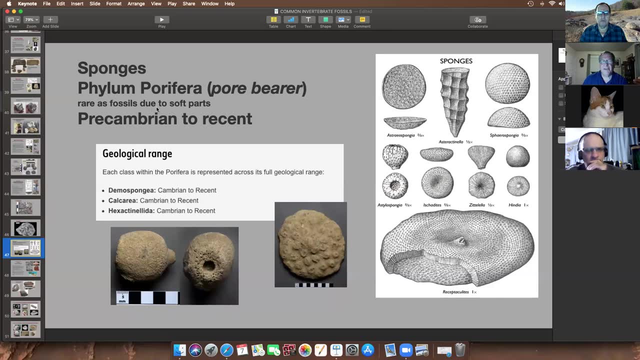 oh, one other thing i'll mention um the uh under periphera in the new paris limestone quarry. another class of periphera are the stromatotoperoids. stromatotoperoids look like stromatolites but they're actually related to sponges, and there are a lot of them in the new. 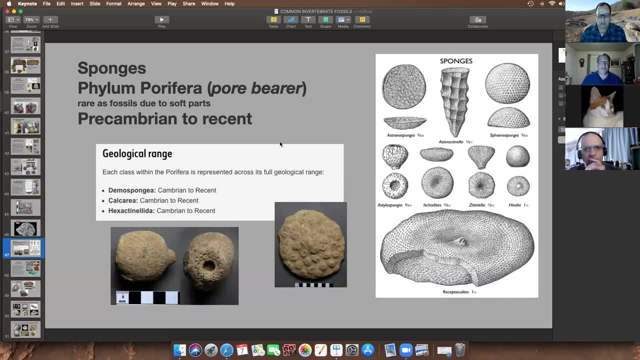 paris limestone quarry. so you'll have a chance to, if you're going on that trip, you'll have a chance to find some stromatotoperoids which, um, uh, look a lot like, uh, stromatolites, but they're- but they're more related to sponges. so that takes us through, i think, pretty much all the major phylum. 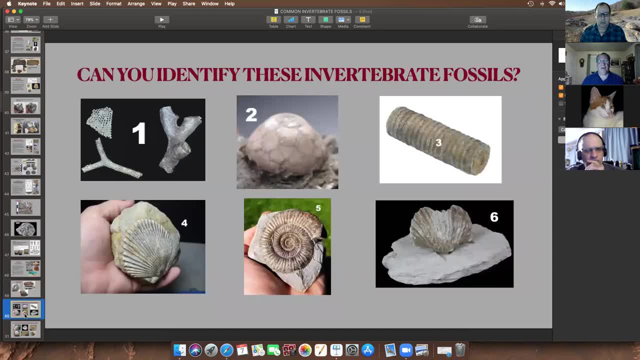 of um invertebrate fossils. then i just kind of um- i wasn't sure how much time we would have left and i was just going to kind of show people some quick pictures and ask them to chime in on their identifications. so i'll just show these to you and you can just do. 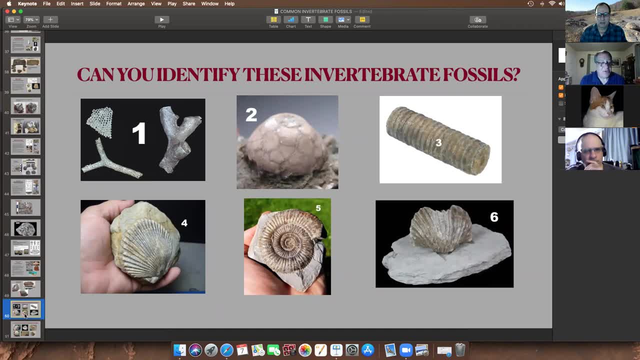 it. uh, so we don't take up more time. if there's any questions, we'll leave a little bit extra time. so you can just kind of look at pictures one through six here and see if you can identify either the common names or the phylum or what. what six organisms are you looking at there? 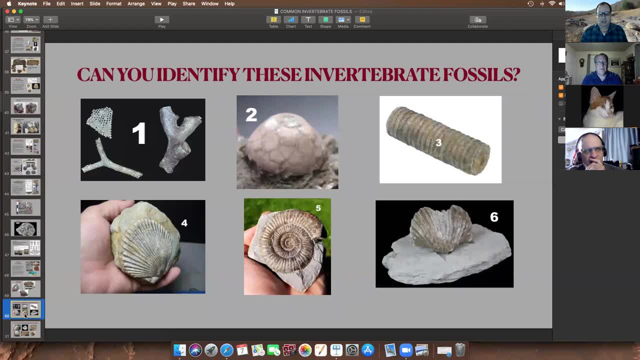 all invertebrates. so, number one, these are, um, these are bryozoans. number two, it's upside down, but uh, this is the calyx of a crinoid, the cup, the body of the crinoid, with the plates. number three, this is a crinoid stem. 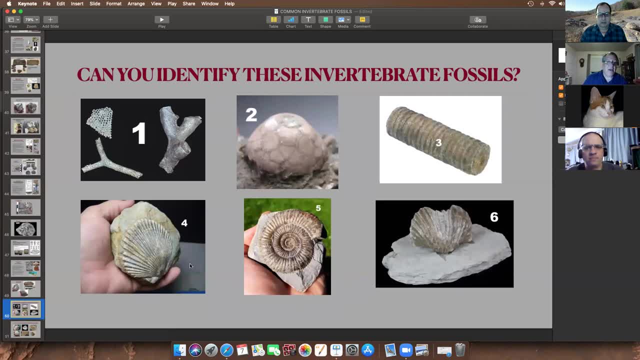 part of the column number four. uh, number four is actually a? um, that's a bivalve. all right, you're not seeing the other side, but that's actually a fossilized bivalve, not a brachiopod. uh, the other shell would have been symmetrical. this is an ammonite and there's a brachiopod. and then, finally, 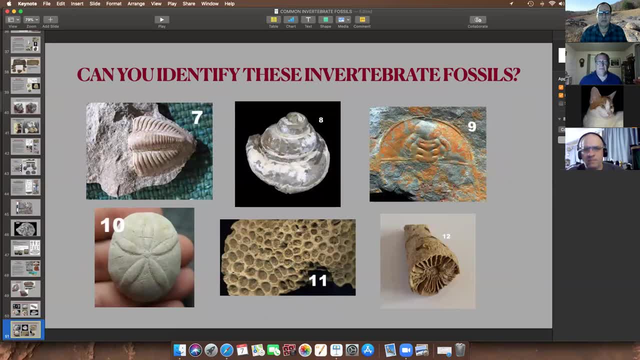 uh, here's uh, six more so you can see if you can identify the name or the phylum or the type of animal you're looking at. number seven is a? uh, this is the tail or the pagidium of trilobite. uh, number eight is a gastropod. number nine: this happens to be, uh, this happens to be a. 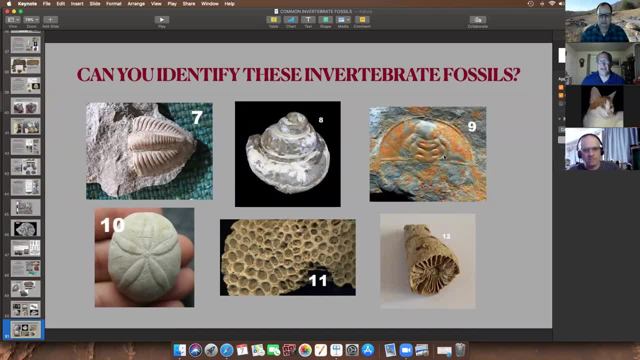 cambrian, lower cambrian trilobite. i think this is, uh olamelis. uh, this is from nevada, one of the earliest known trilobites. that's just the cephalon, uh, the part of the head. it's probably part of a. 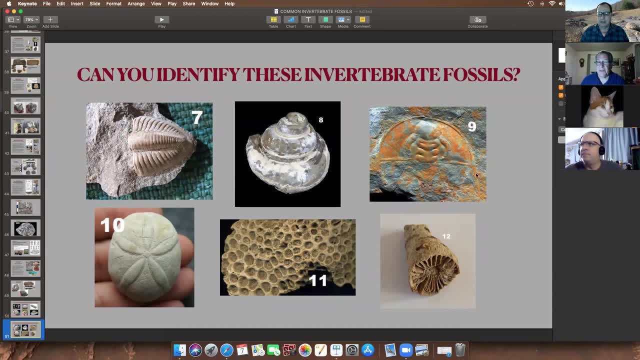 malted shell. you can see a little bit of the genal spine here, one of the spines coming down off the right side. here's an echinoid, uh, fossil sea urchin or sand dollar fossil coral. it's actually a hexachoral. and here's a? um, a rugosa, a rugose coral. 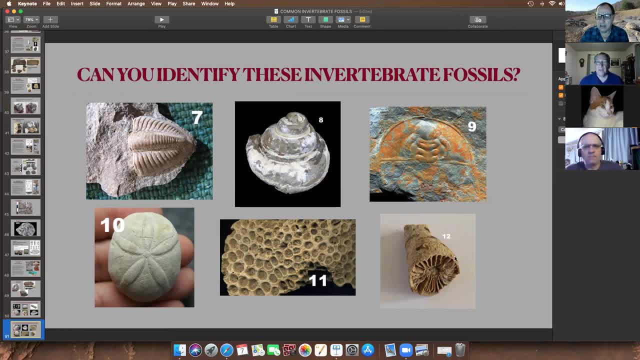 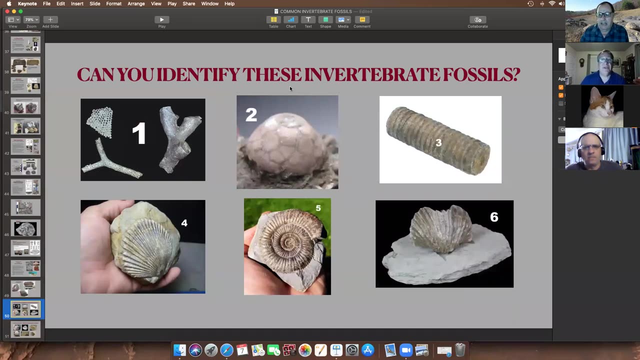 giant solitary coral from the paleozoic. so that brings our program. i ended up going to late 20, so we have a question back on the previous slide and number five. yeah, uh, number five. yep, oh, it's where chat. yeah, how can you tell the ammonite from a nautilus? uh, let's see. oh, how can you tell the? 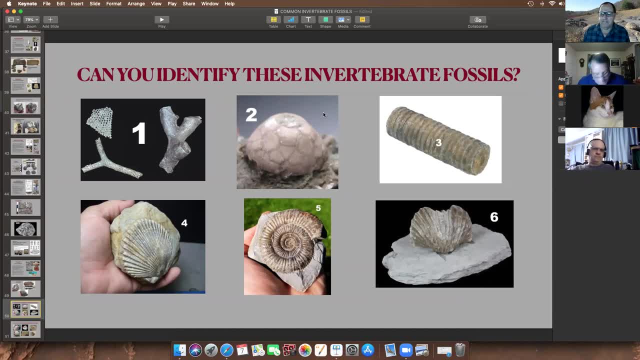 ammonites from a nautilus. okay, the nautilus will have. let me get my, get my magic marker out here, probably the easiest way. if you um trying to draw a nautilus shell here, okay, if you look at the shell of it. if you look at the shell of a nautilus, okay, the um, if you can see the fossilized cy funcle. 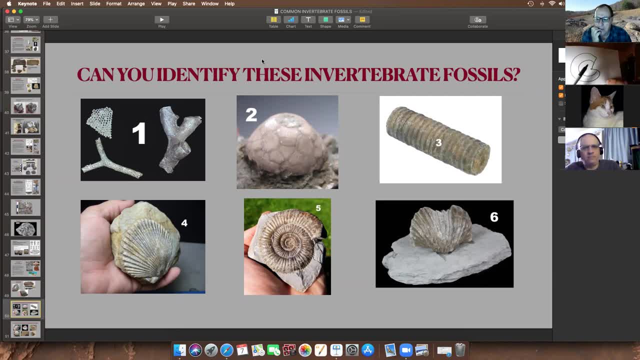 the. the cy funcle of a nautilus will go through the- i'm trying to do this backwards here- cy funcle of a nautilus will go through the middle of a shell and if you have an ammonite, the cy funcle. i'm just going to draw this as a squiggly line. 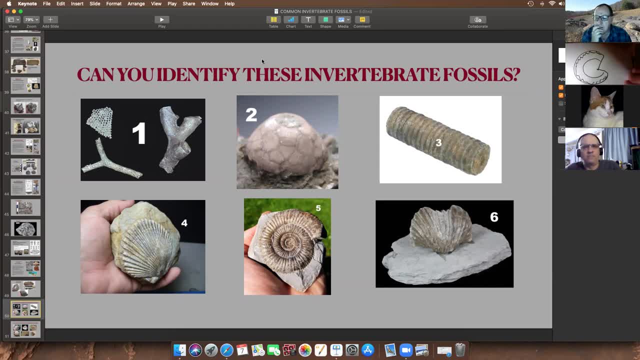 if you have an ammonite, the cy funcle on the inside of the shell, or is my pen, the cy funcle will go along the outside of the shell. so a nautilus- a nautilus has a centered side funcle and an ammonite has a side funcle that goes through the outer edge of the shell. the other 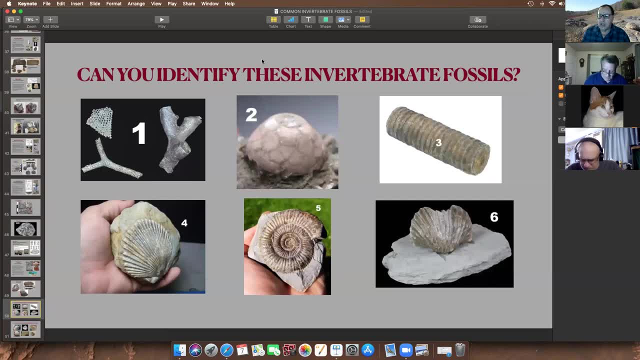 way you can tell is if you look at um, let's see, i'm just going to draw the- uh, i'm just going to draw. here's a piece of um, here's a piece of the shell, all right, so if that's a shell, a nautilus. 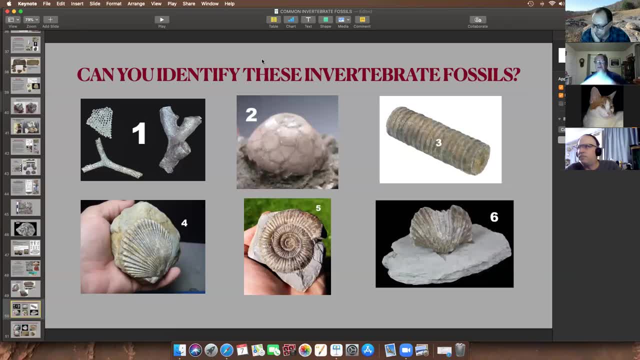 will have. a nautilus will have a suture line that looks like that. so on the outside of the shell you will see a wavy suture line. these are called saddles and lobes. so a nautilus will have lobes and saddles. an ammonite looks like an ammonite, has saddles and lobes, but they look like this. 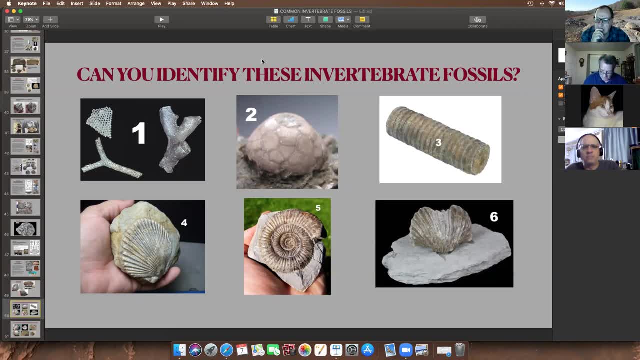 and i'm just going to take second here to draw them. so here's what a nautilus will look like. i'm sorry, nautilus. a nautilus has a smooth, simple saddle and lobe suture line in ammonite. the suture line looks like this: it is extremely ornate. 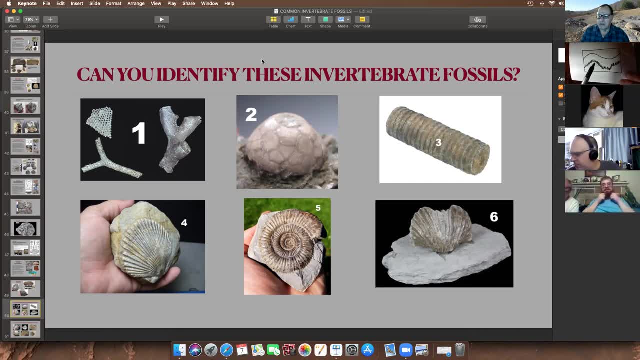 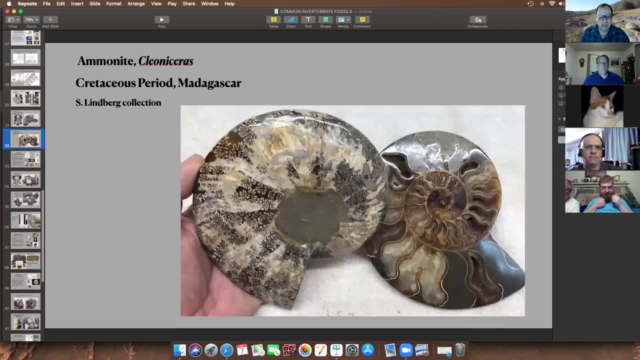 and um, we call that, uh, saracitic or ammionitic, and um, let's see, we can just go. let me go back here. where was uh? there it is, this is uh, this isn't. this is definitely 100, this is an ammonite. um, you look at the outside of the 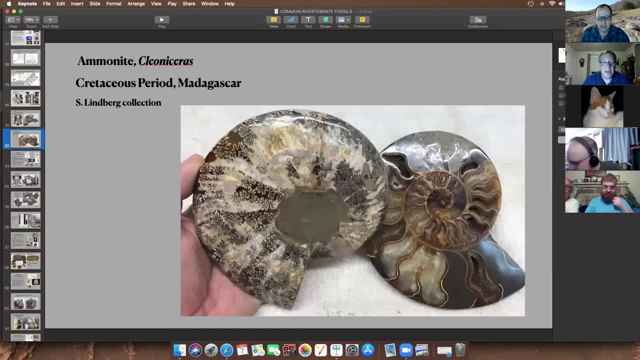 shell and right there you can see the suture line. and look at that. it almost looks like i. i tell my students: um, in ammonite suture pattern, it looks like the frost that you see on a cold winter morning on your window. if you look at the, if you look at the frost. 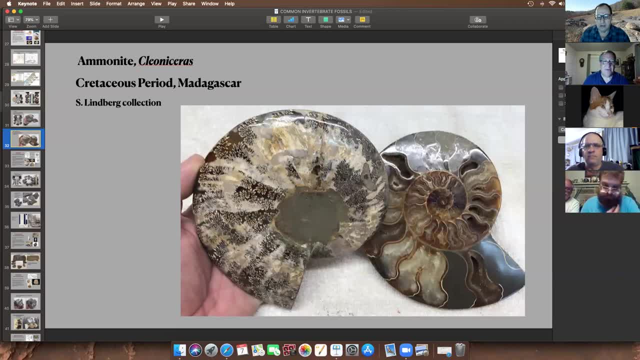 that forms on your window. it will sometimes make this type of pattern. so an ammonite has this very intricate and deep, detailed suture pattern and if you have a really, really well preserved animal, you can pick this up on one side of the shell and you can actually trace it the entire way around the shell to the 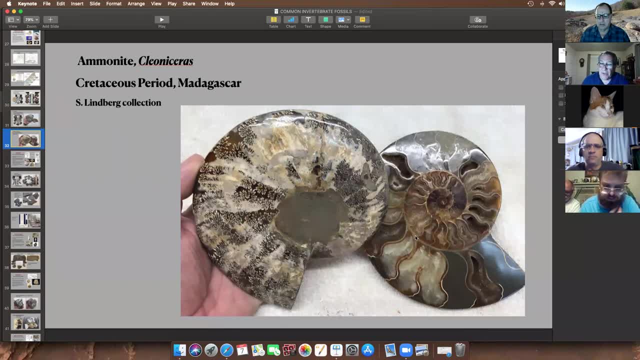 other side and what you're looking at. you're looking at this septum right here, um, where it touches the outside of the shell, that contact point, um, now this, this ammonite, the uh, the siphuncle is not preserved. this is not the siphuncle, that's the this was. this is the outside of what uh used to be the shell. 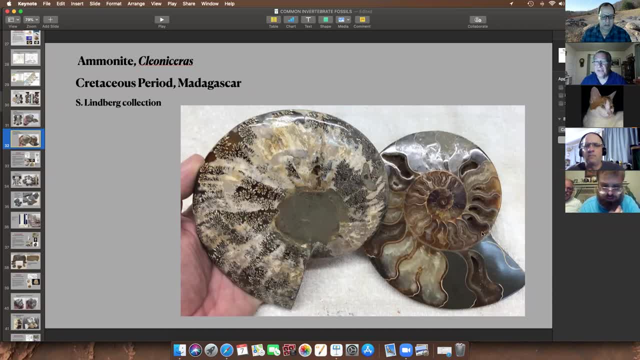 all right, so that's the previous growing chambers. the side: the siphuncle would be in here somewhere, but it's not preserved. the siphuncle probably ran through this little lobe right here, so you can see that each one of these septa has a lobe in it. so that's where the side. 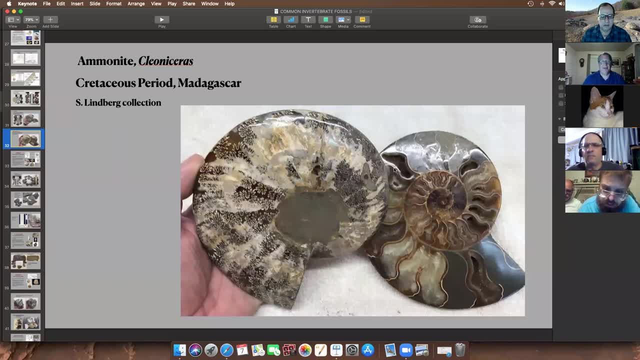 the siphuncle is usually not preserved because it's a soft tissue part in an ammonite, so does that answer? you have other questions? uh, core trip is free. yeah, um, i suggest everyone coming to the core. you want to? um, uh, and you know.